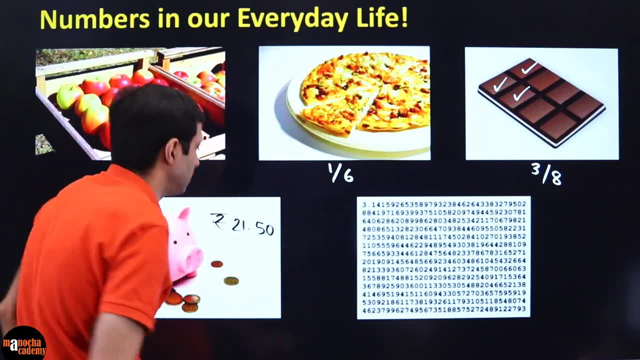 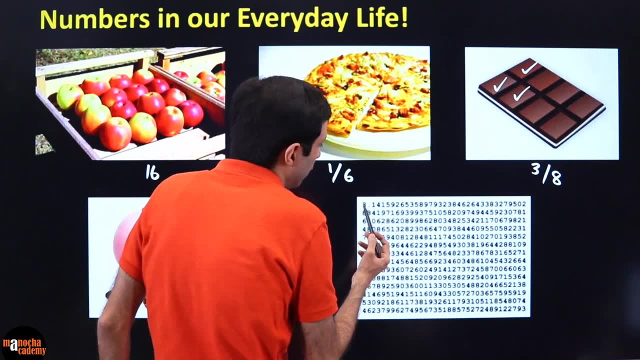 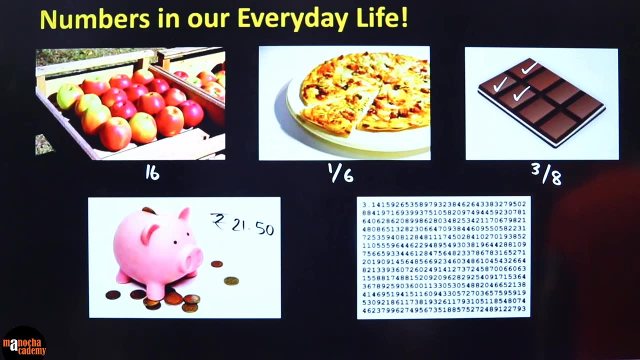 21.50 rupees. So that's a decimal number. We use decimal numbers. Can you guys recognize this number? Let me read it out for you: 3.141592653535897932.. Anybody recognizes? Wow, you guys are fantastic. Chatura Ashmit, Sian Jishnu. 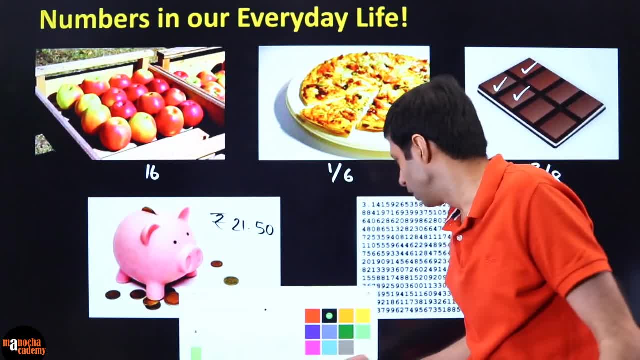 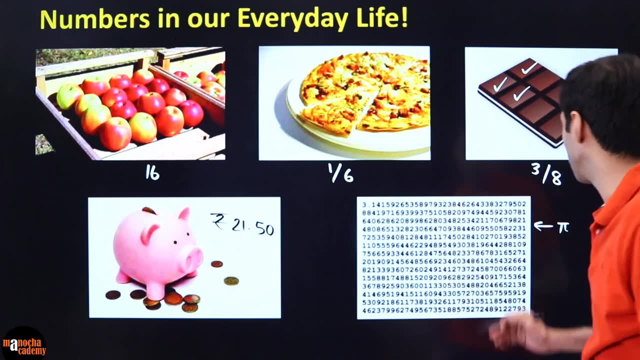 Eram Kaushik. everybody has the right answer. Tamogna. very good. So this is nothing but the value of pi. You'll say, why is it so long? Yes, it's crazy, And we're going to talk about pi today. 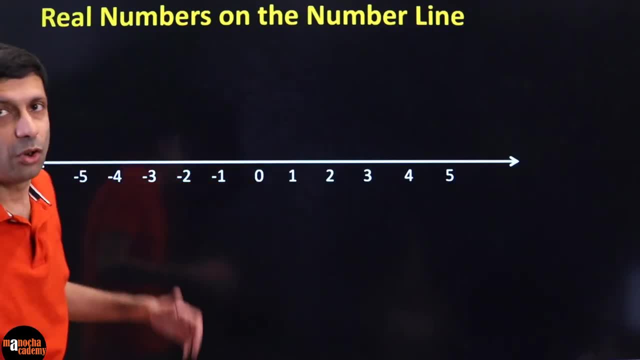 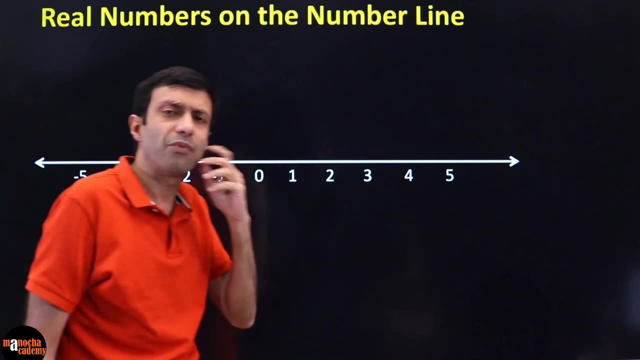 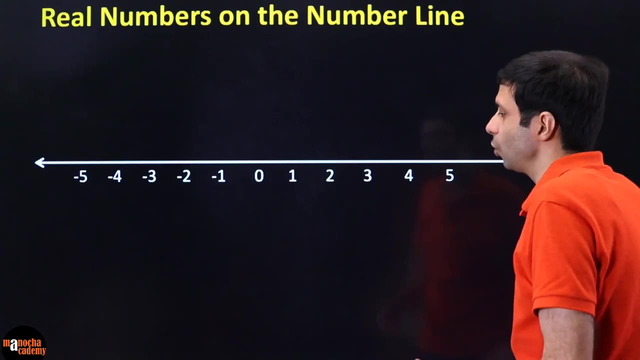 The famous pi of mathematics. So there are lots of numbers And there's this important term: these, all these numbers are called real numbers. So question is: how do you define? so all the numbers we talked about right in this previous slide? These are all real numbers. How do we? 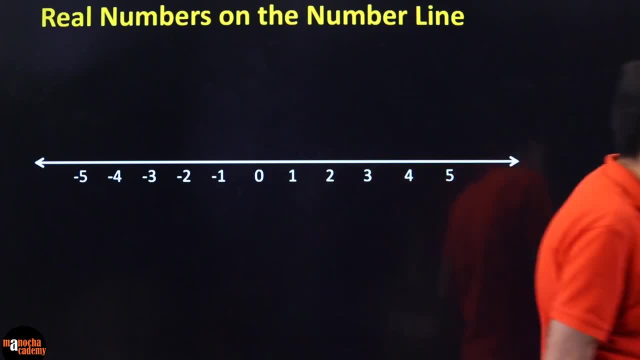 define what are real numbers? can you guys tell me what are real numbers? every number is a real number. integers, rational, irrational. see i'm getting different answers. numbers starting from one: those can be shown on a number line. okay, many many this thing here, so i'll come to that question. 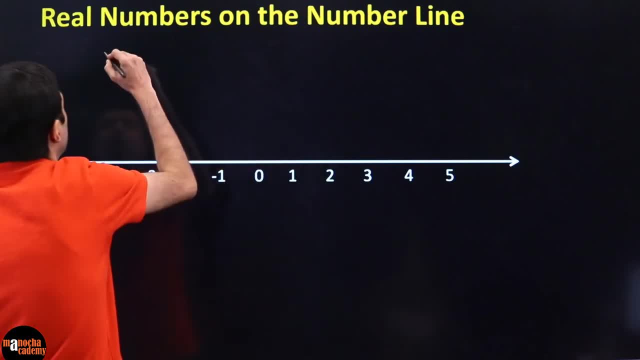 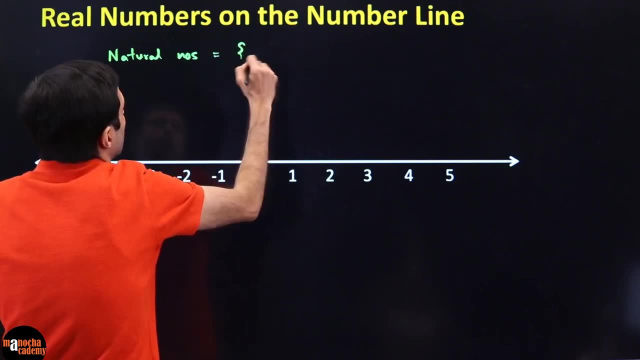 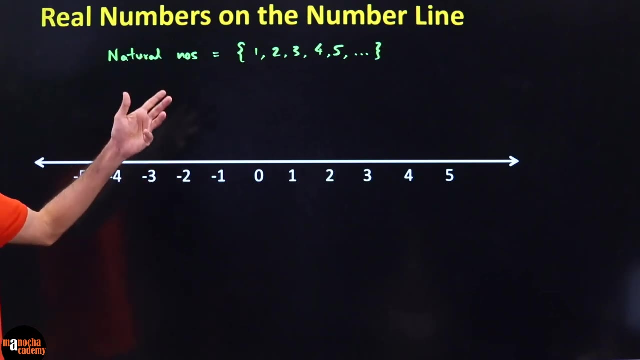 first let's talk about the simple numbers that we know already. you guys have heard of natural numbers. can you give me example? what are natural numbers? natural numbers are when you start from one, like one, two, three, four, five. these are natural numbers, right counting numbers starting from one. 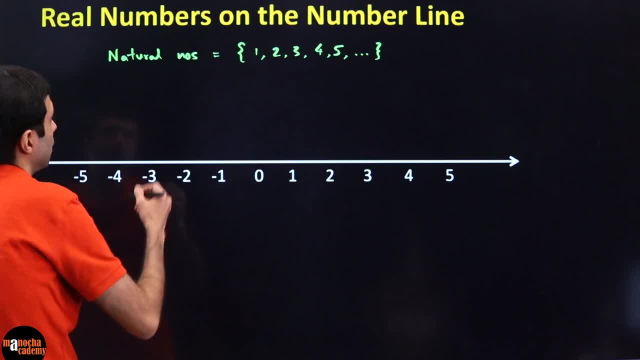 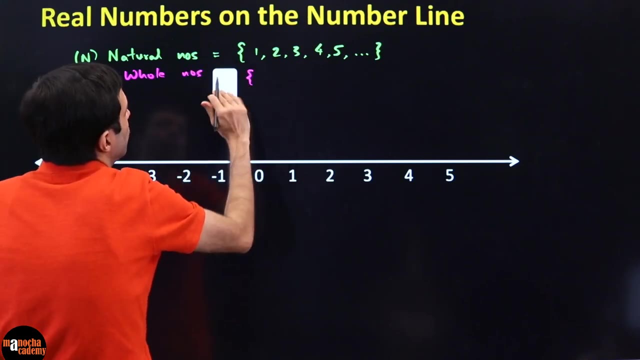 next, you guys know what are whole numbers: natural numbers we represent with the symbol n. then you have whole numbers. whole numbers we represent with w. what are whole numbers? again natural numbers. the only thing is you add a zero to that. so zero one, two, three, four, five and so on. 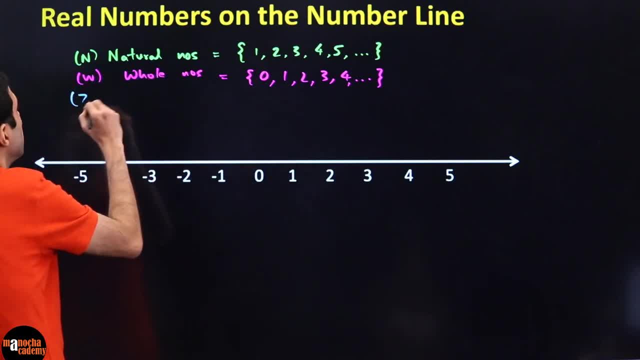 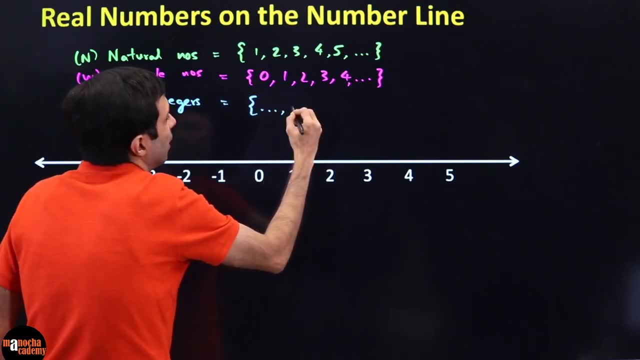 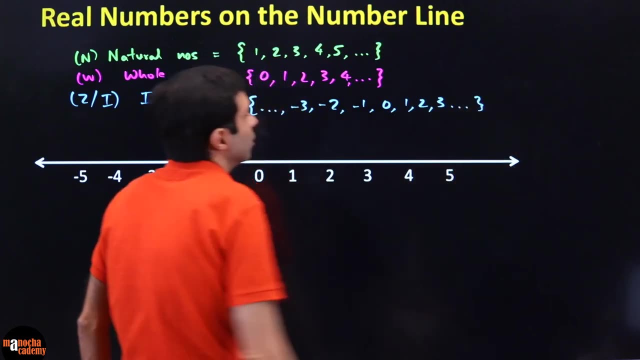 then what else? you know, there's something called integers, which is represented by z or i. what are integers? they are all the whole numbers, and then negative numbers as well, like minus three, minus two, minus one, zero, one, two, three and so on. so all whole numbers and their negative are integers. 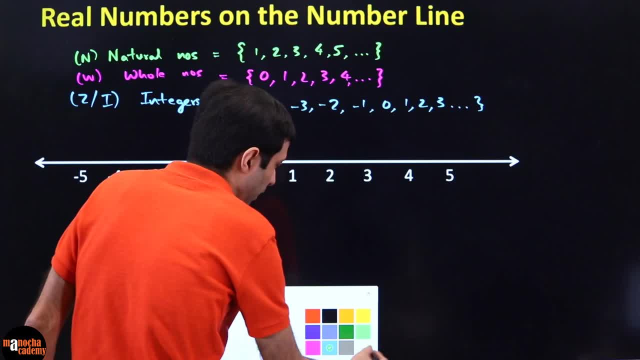 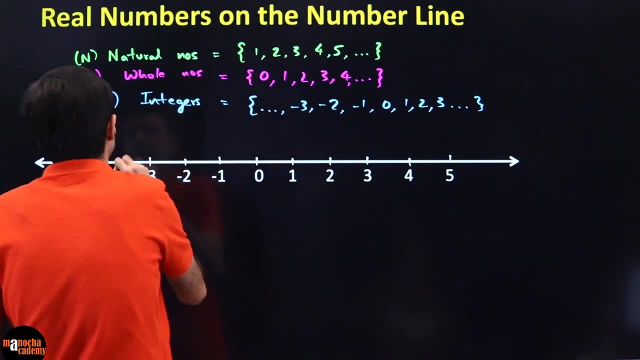 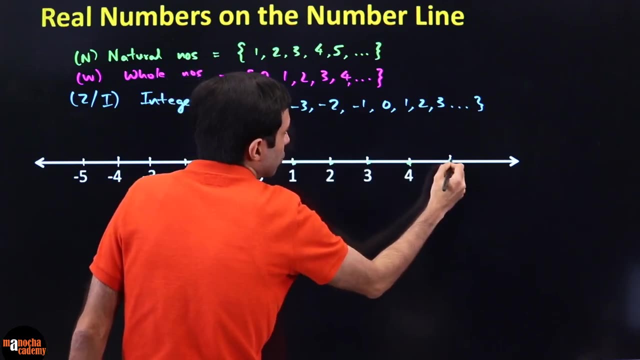 can you represent all these on the number line? you guys have heard of this number line, right? so you have zero in the middle. you have one, two, three, four, five. so all these are numbers on the number line, like natural numbers we can put over here: one, two, three, four, five and so on. 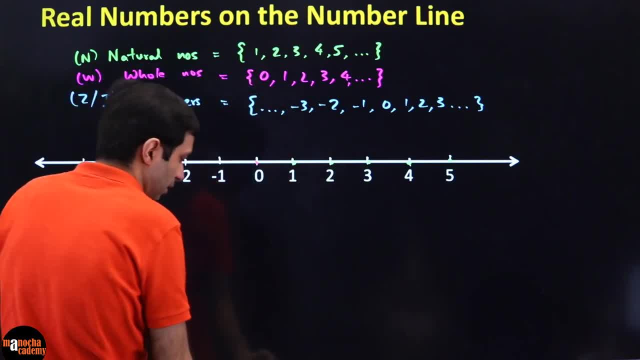 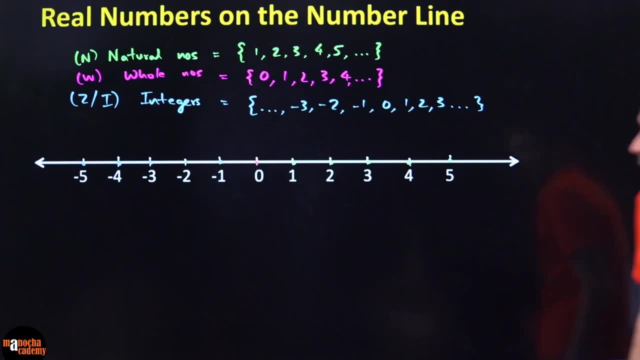 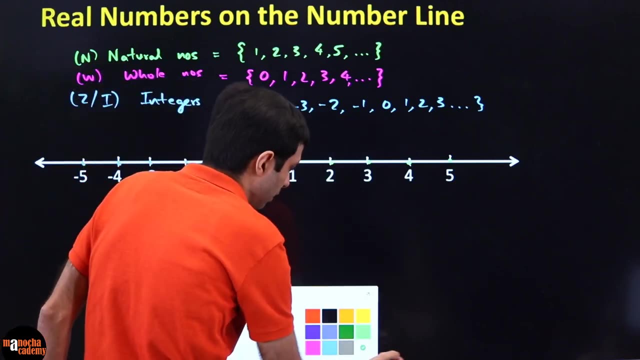 whole numbers is all these natural numbers and the zero as well. integers are all these numbers and minus one, minus two, minus three, minus four, minus five and so on. but now the question is: are there more numbers on the number line beside these ones? yes, certainly, why not? there is the number you have half on the number line, which is exactly between 0 and 1. 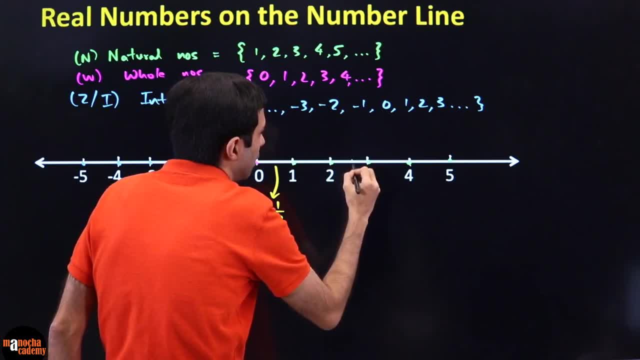 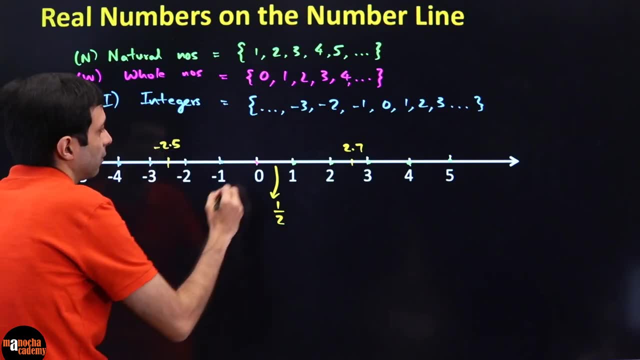 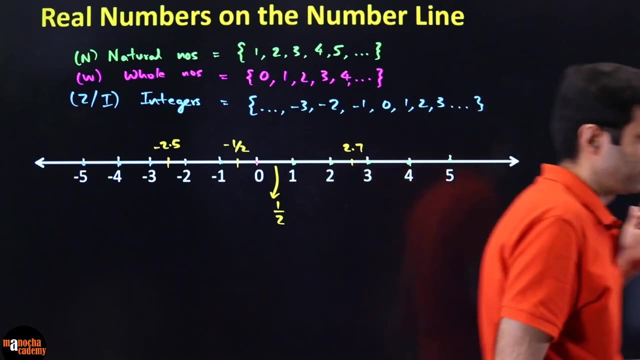 then you can have, let's say, we can have a 2.7 here, right? we can have a minus 2.5, we can have a minus half. so what are all these numbers? what do you call these that i'm putting over here fractions, decimals. very good, these are in fact called the rational numbers, right? 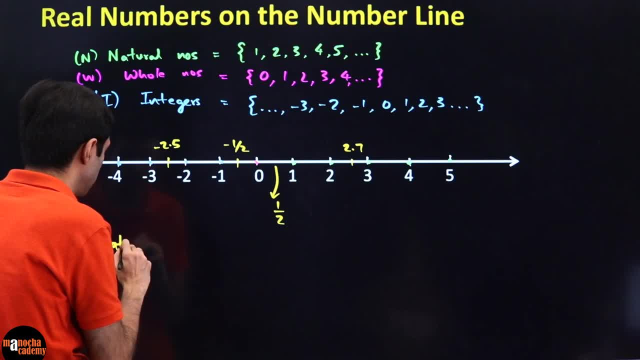 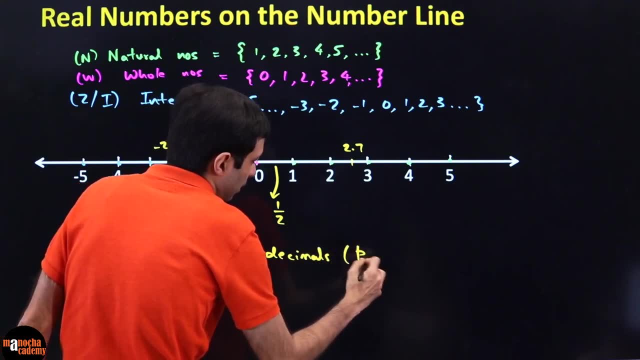 so all i'm showing over here these are all rational numbers, which are all these fractions and decimals that we'll talk about in p by q form. they can all be put on the number line. and then are there more numbers on the number line besides number line. 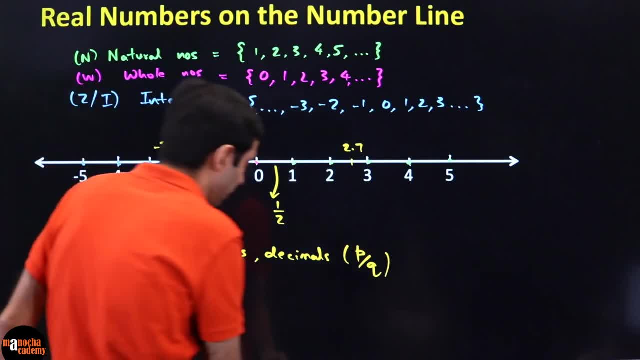 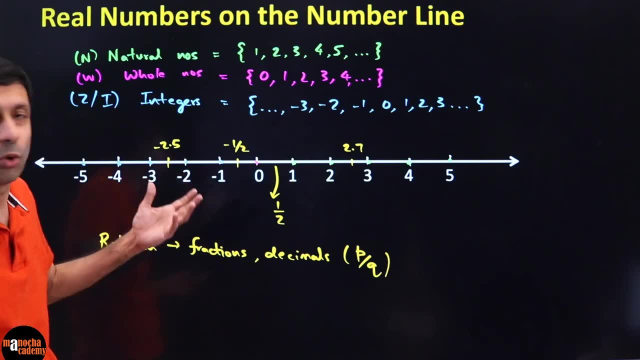 decimal line fractions. yes, there are something like you know. you can have a, you can have the value of pi, you can have root 2, root 3. there are so many more numbers on the number line. so the collection of all these rash, this natural whole number, integer, rational, irrational numbers. 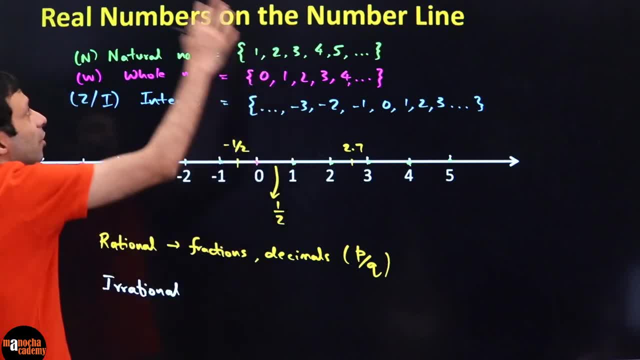 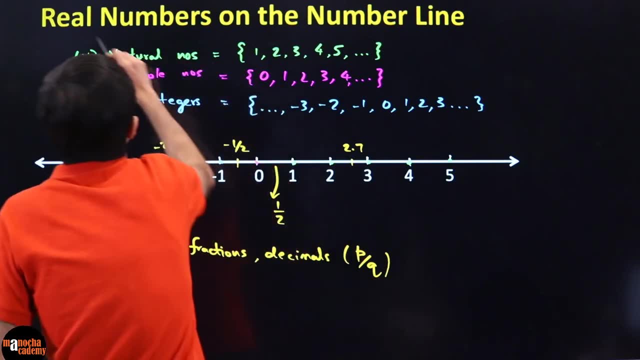 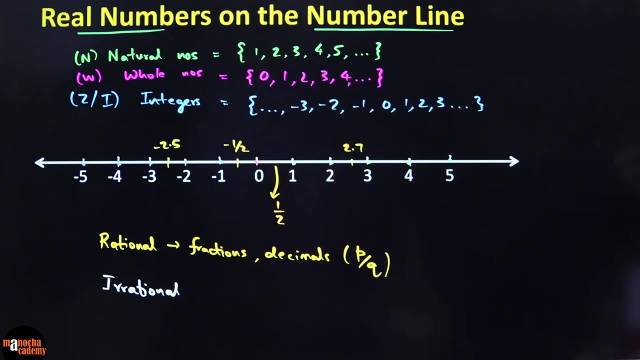 all of these together are known as real numbers. and real numbers you can visualize, you can plot them on the number line. so real numbers can be plotted on a number line. clear, that is the meaning of real numbers. now question is: is zero positive integer, negative integer, or is it neither? 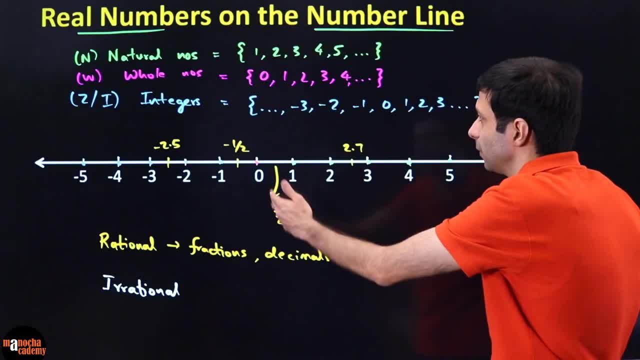 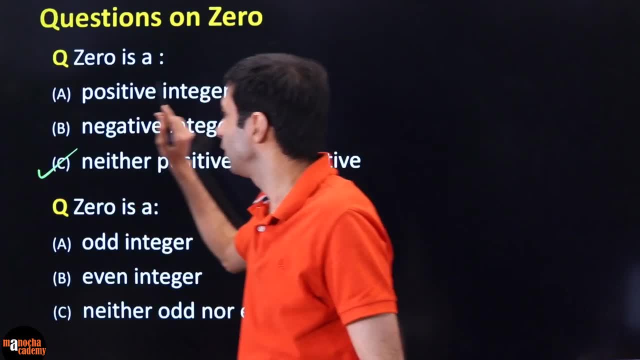 positive nor negative. so zero is right here in the middle. here you can see all the positive numbers, here are all the negative numbers. so here we can say the answer is going to be: it is neither positive nor negative, because it's in between is zero an odd even. 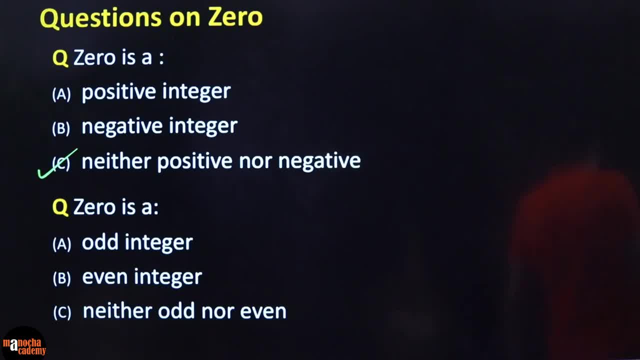 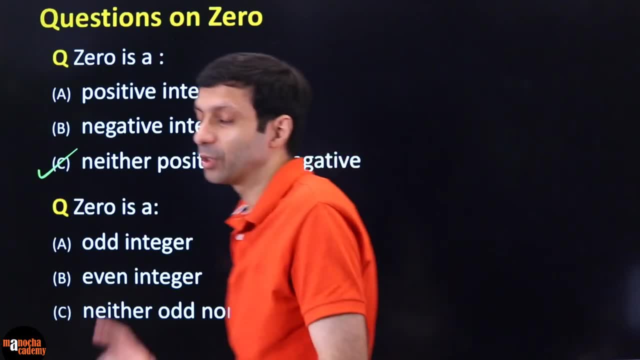 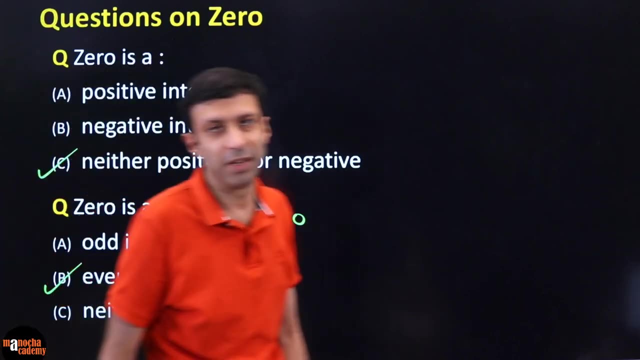 Integer or is it neither or not even? Do you guys know the answer for this? I think Sian has the right answer. Anybody else? 0 is considered even. Why? Because even means something which is divisible by 2.. 0 by 2 is 0. So it's divisible by 2.. Answer is an even integer. This chart is: 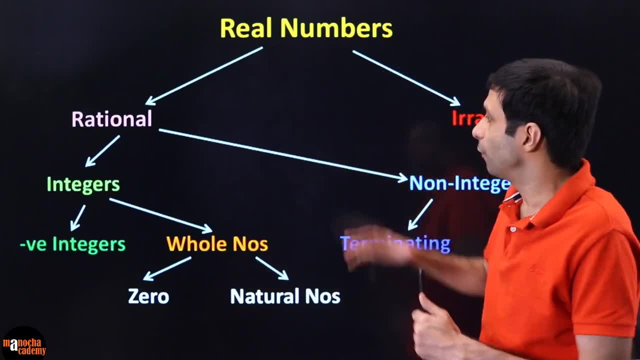 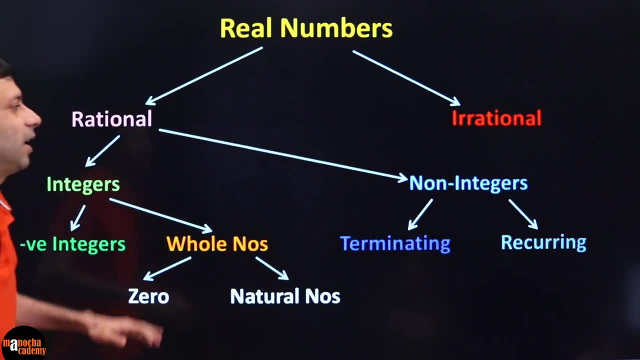 very, very important. I want you to visualize this. In fact, you can even draw this and we're going to discuss, because there are so many terms over here. You can see, and we are going to understand, how real numbers are divided like this. Till now, we have done the easy stuff. 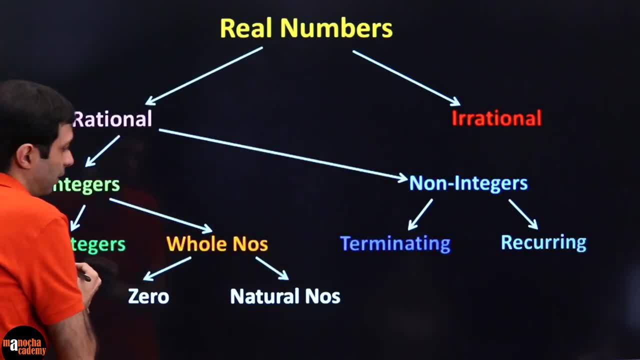 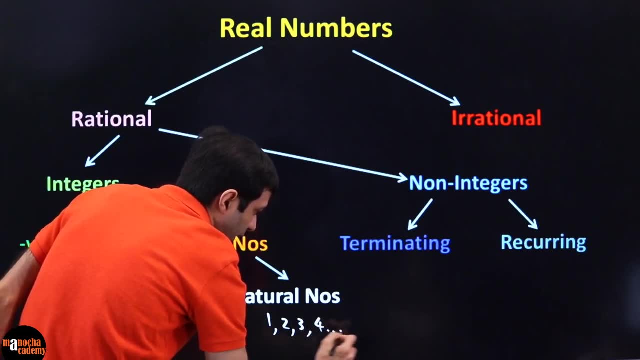 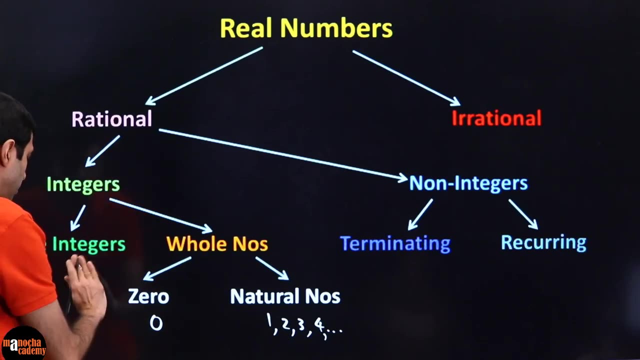 We have talked about the negative. We have talked about the natural numbers like 1,, 2,, 3,, 4 and so on. These are also called counting numbers. If you add 0 to that, then together they are known as whole numbers and then negative integers. you guys know minus. 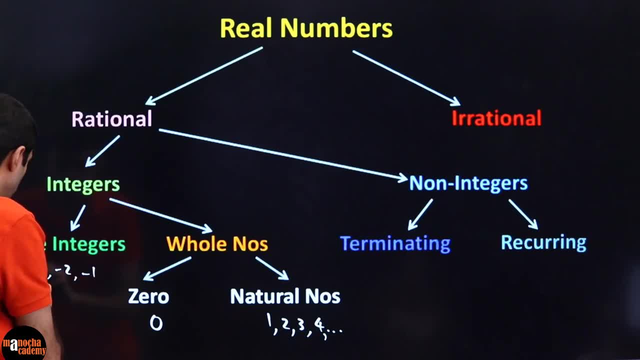 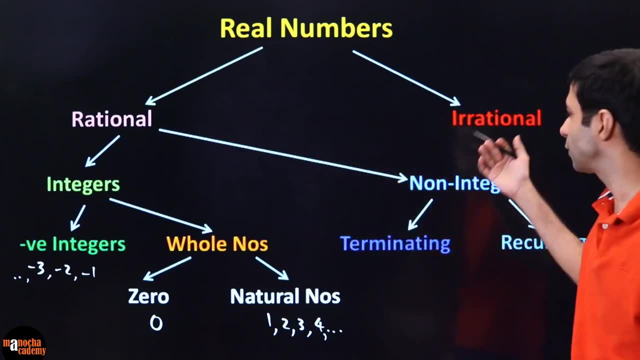 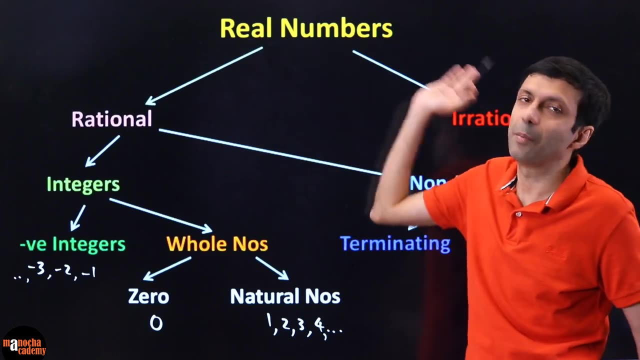 0.. Minus 3, minus 2, minus 1, and so on. So you guys are familiar with all of these and together these are all known as integers. But what are rational, irrational, all these non-integers, terminating, recurring, Let's talk about And remember? these all come under real numbers. 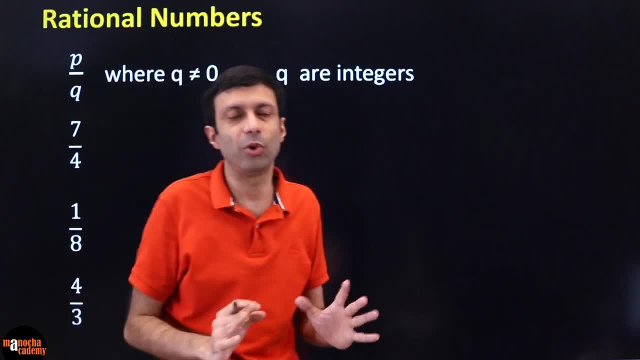 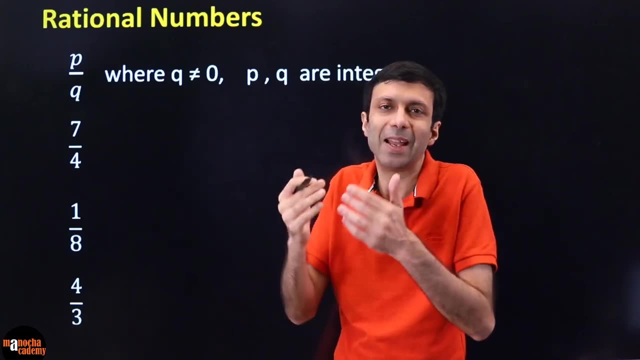 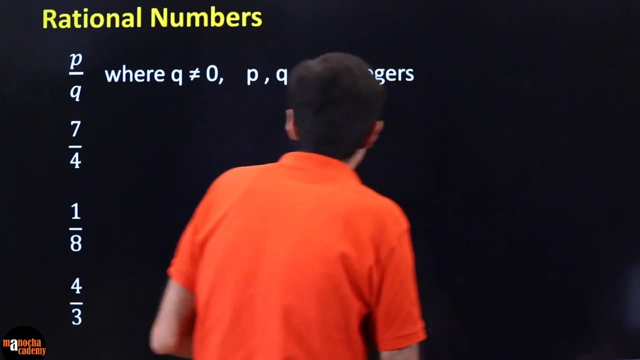 So first let's talk about what are rational numbers. The easiest way to remember this is rational numbers can be expressed in p by q form, p by q. in p and q are variable, like x by y, 3 by 5, 2 by 3.. So basically you can remember, rational numbers are fractions, because you can 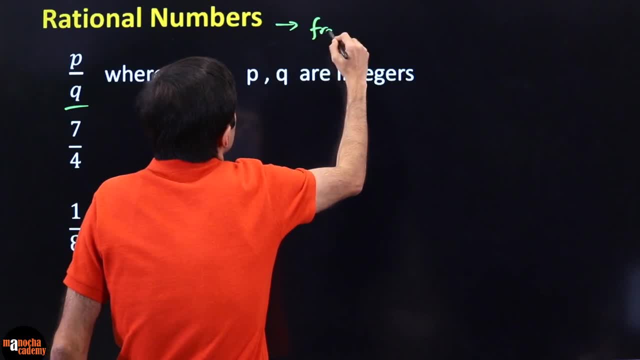 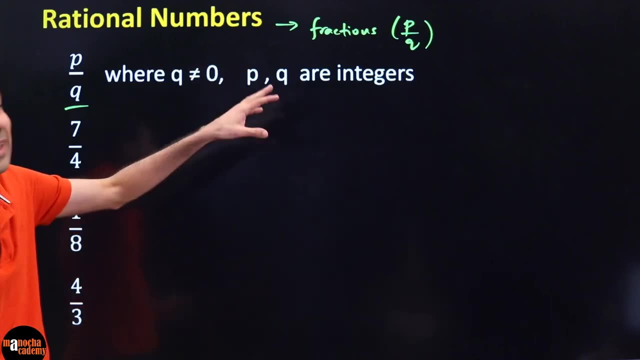 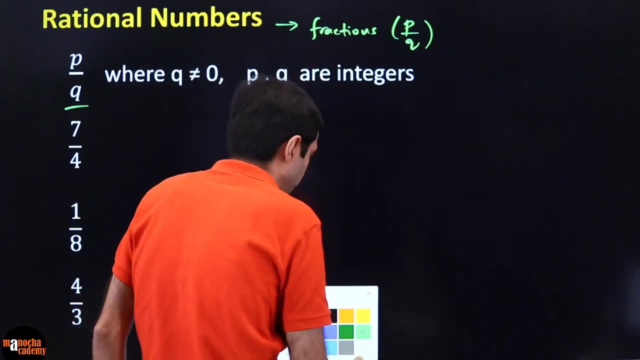 express it as a p by q form. So easy way to remember. hey, these are fractions p by q form, where p and q are integers. In some books you will also written it's co-prime, which means they don't have any common factor. Like if they had a common factor, you have cancelled it, For example. 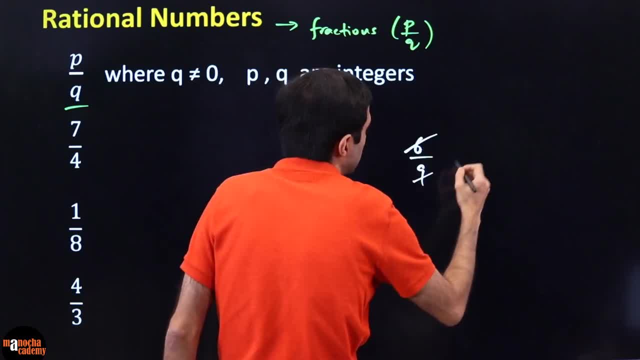 if something was 6 by 9, you will not keep it 6 by 9.. You will cancel and you will not keep it 6 by 9.. So if you have a common factor, you have cancelled it. For example, simplified to 2 by 3. You will divide both numerator denominator by 3.. So many times. 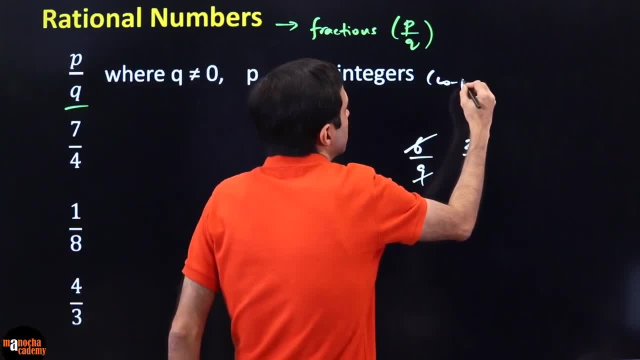 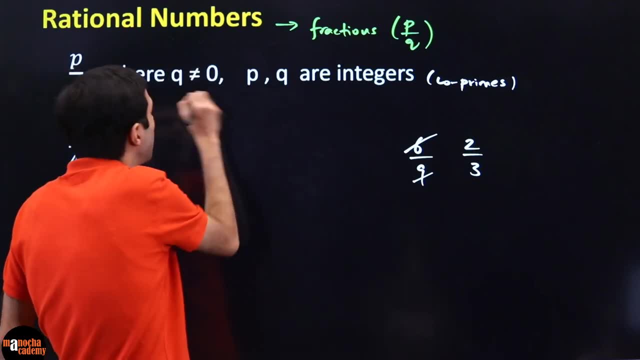 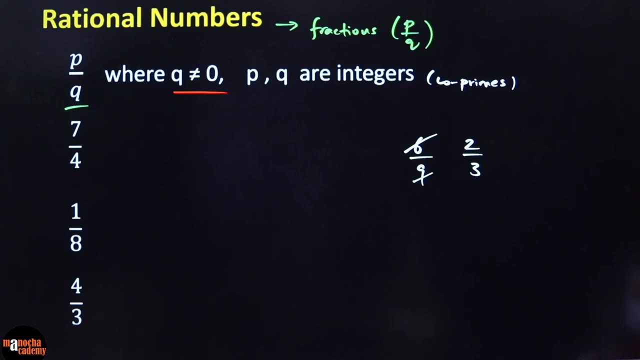 you will see it's written as they are integers, They are called co-primes, No common factor. Now why this restriction that q is not equal to 0? Why do we have this restriction on rational numbers, Imaginary numbers? very good, So that is out of the syllabus right now that you can. 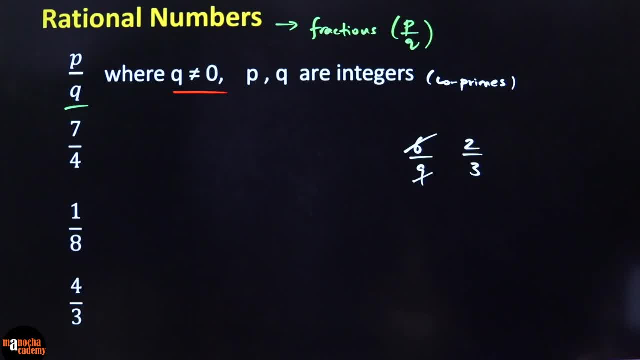 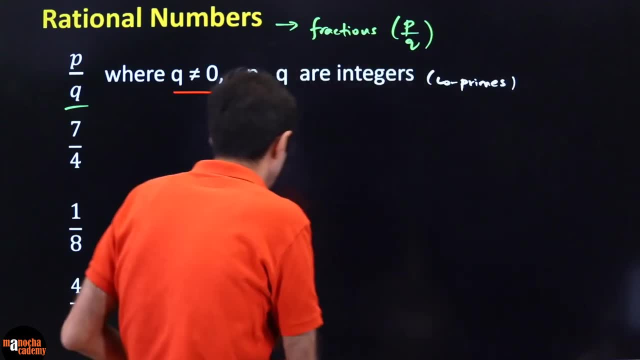 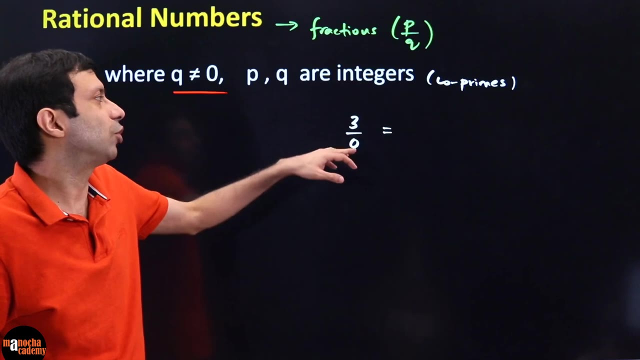 have numbers which are imaginary or not real. So but why this restriction? that, hey, p by q is integers, but q should not be 0. So you take an example: If I tell you guys, hey, let's do 3 by 0. What is the answer? What is 3 divided by 0? You have 3. 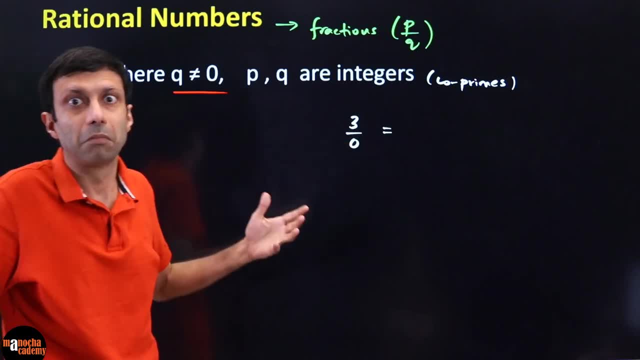 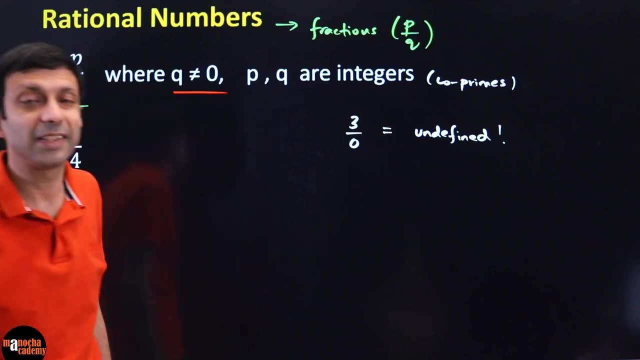 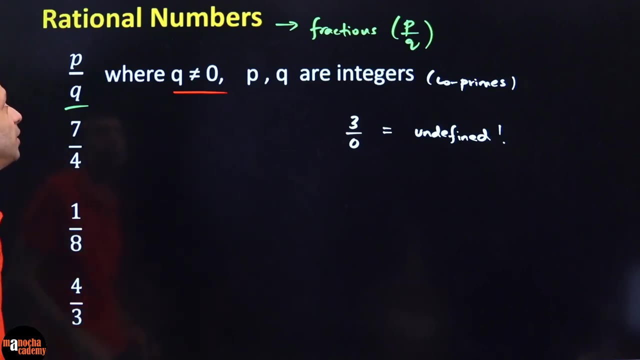 chocolates and 0 people to eat it. How much does each one get? In mathematics this is considered undefined. This has no meaning. 3 by 0- undefined, It's like a crime in mathematics. So that is why we say, hey, q better not be 0.. Okay, q should not be equal to 0. So we 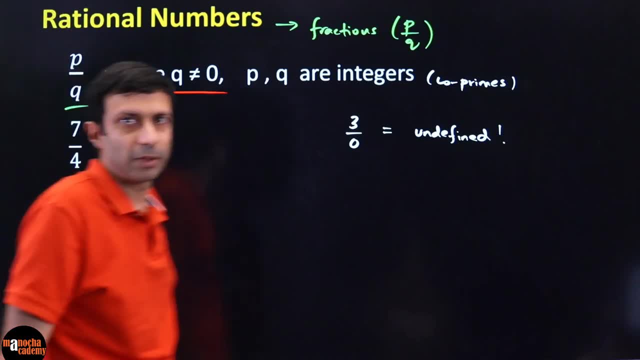 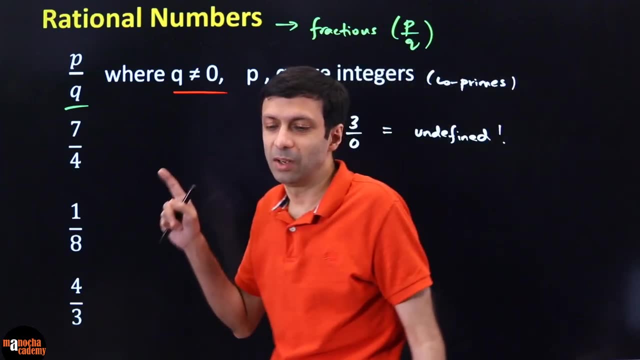 say rational numbers are p by q form. Is 7 by 4 a rational number? Yeah, it's like error in computer Error, error error, Exactly. So 7 by 4, see it fits p by q. and if you do 7 by 4, what is? 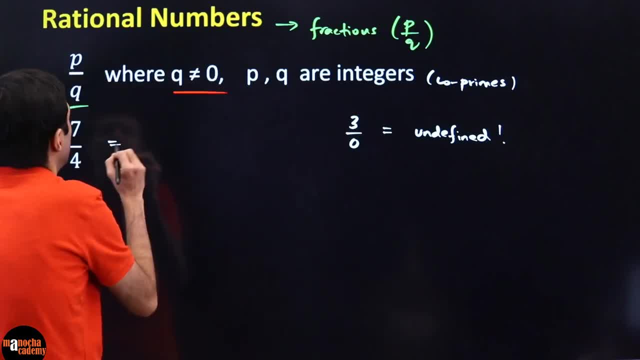 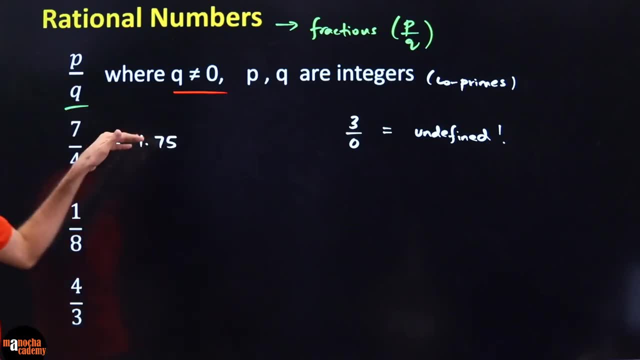 the value you guys are going to get If you do this division: 7 divided by 4 is, I think, 1.75.. So, yes, rational numbers can also be. p by q can be converted to decimal form as well, as you can see here. What about 1 by 8, guys? That is also. 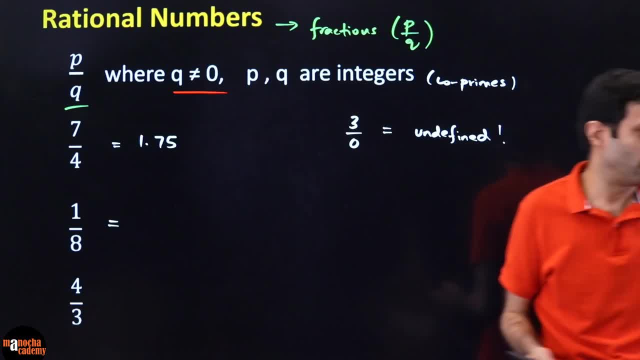 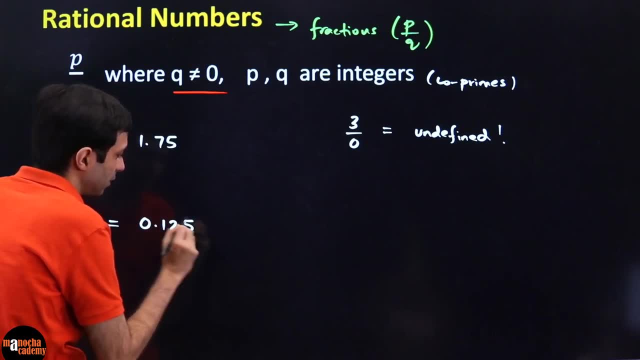 rational p by q form. Can you convert it for me? What will you get if you do the division 1 divided by 8.. Come on, do it guys. I think 0.125.. See again, it gives you a decimal number. 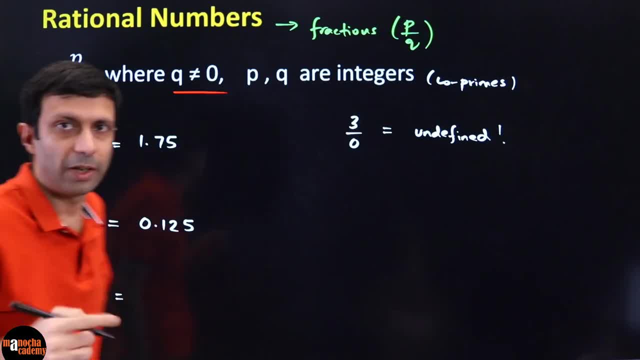 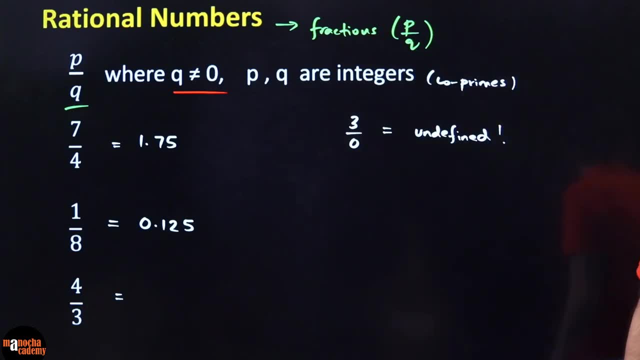 No problem. What is 4 by 3?? If you guys do the division, don't use a calculator. Try to do it yourself, Right, Without any calculators. What is it? Very good, 1.33.. But how many 3 should I put? 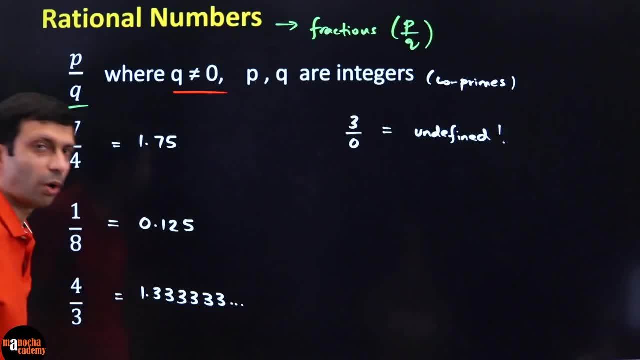 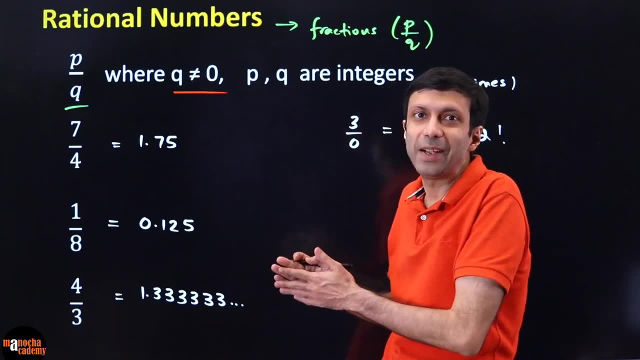 3?, 3., 3.. It just goes on and on. What do you call these kind of decimal numbers which don't stop? They are not. when you stop, we call it terminating decimal stops. This guy is not stopping, Irritating. 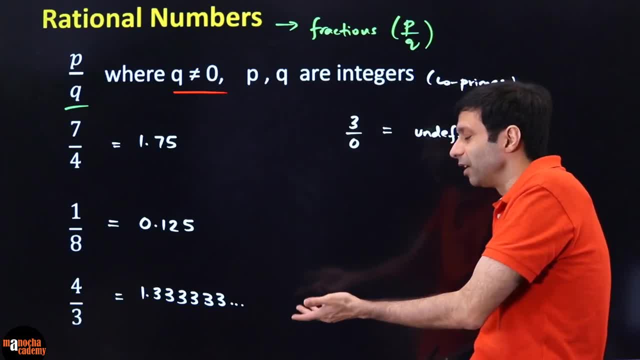 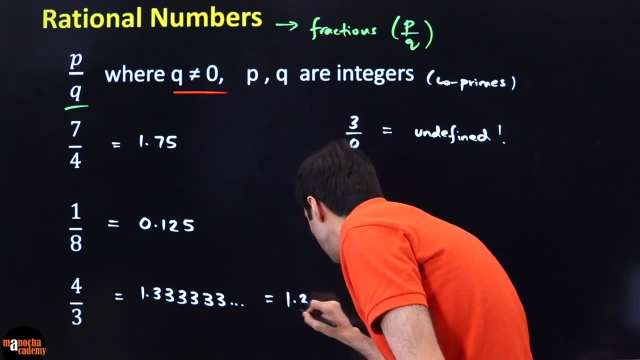 guy, It is non-terminating, or we also call it: since this 3, 1 is repeating, it is non-terminating and recurring. So you must have seen this notation. in maths We write it as 1.3 bar or 1.3 dot, because 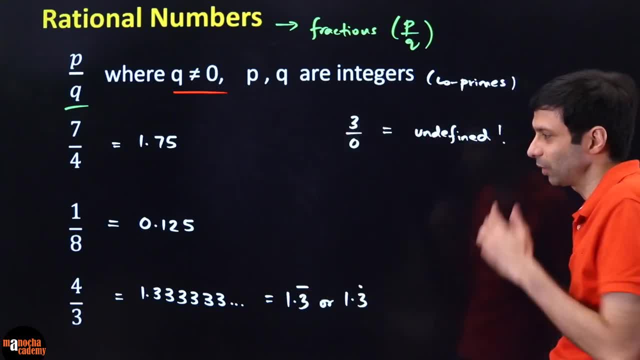 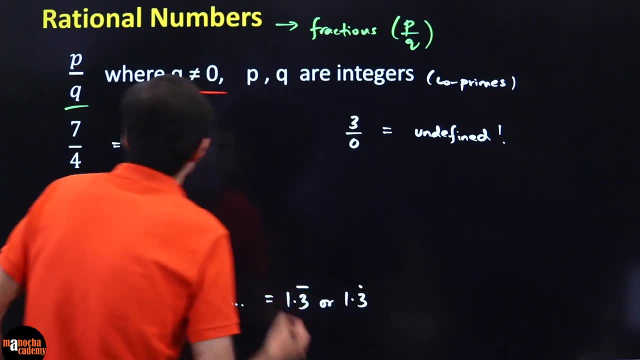 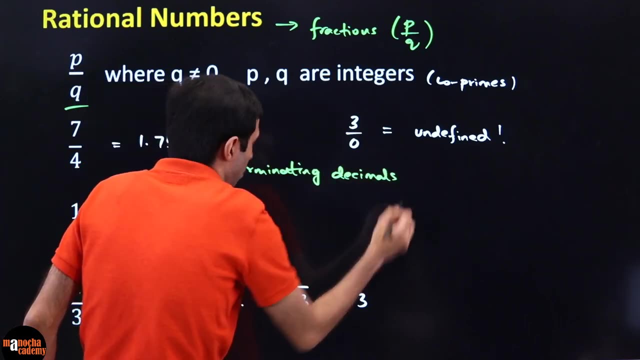 3 bar means 3 is repeating again and again. 3 dot. Okay, These are the irritating numbers not terminating. So what we can say, Rational numbers can be terminating decimal, which means they finish off, not going on and on, thankfully. or they could be non-terminating, which means it is never finishing. 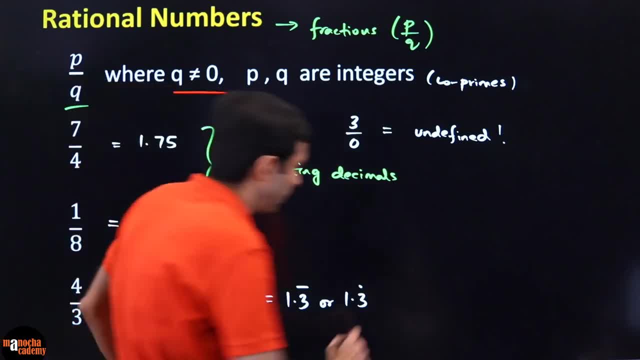 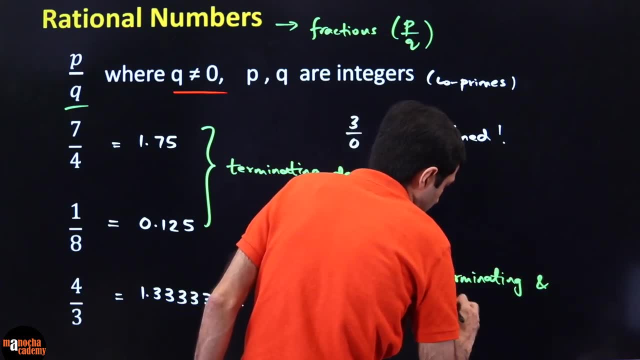 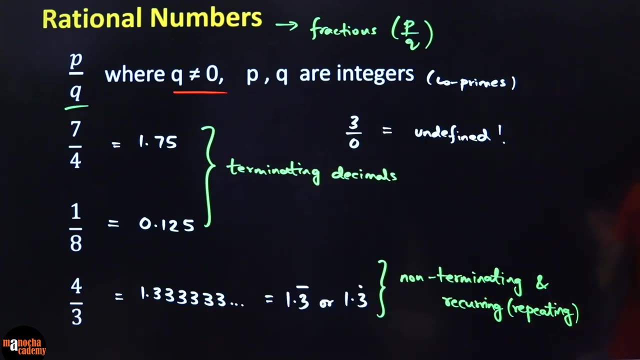 but repeating. Can you see the repeating pattern? 3 is repeating, So they can also be non-terminating, not ending, and recurring. Recurring means repeating, Exactly. Yes, Rishabh Banerjee. It is going on and on. 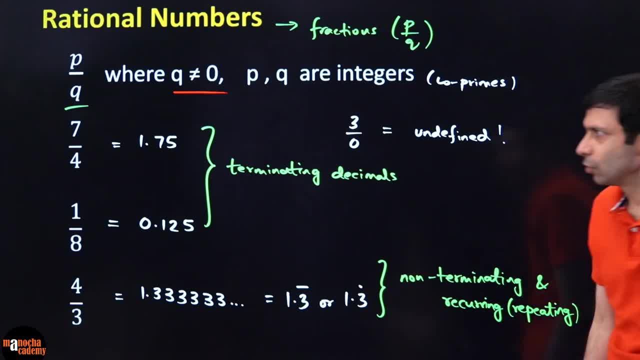 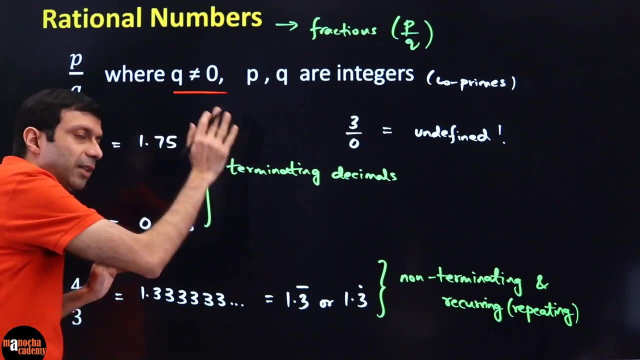 1.33333333.. Okay, So this is one thing. lot of students have confusion. So, first of all, in summary, what have we done? Rational numbers are p by q form fractions. If you sit and divide them, it may terminate- which very nice it has stopped. or there are two options here. It may either 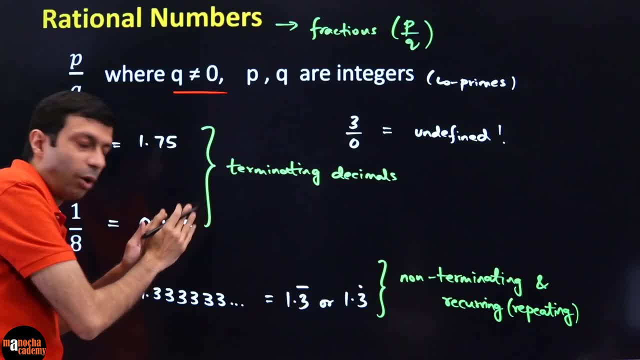 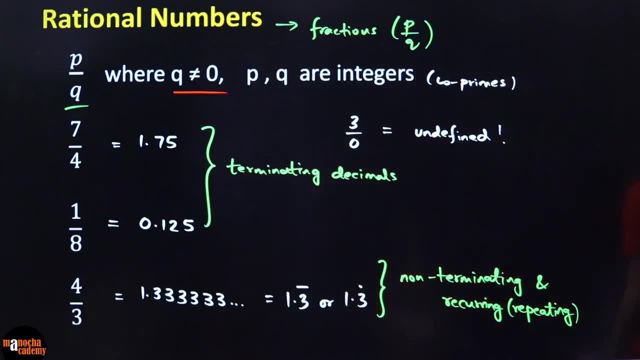 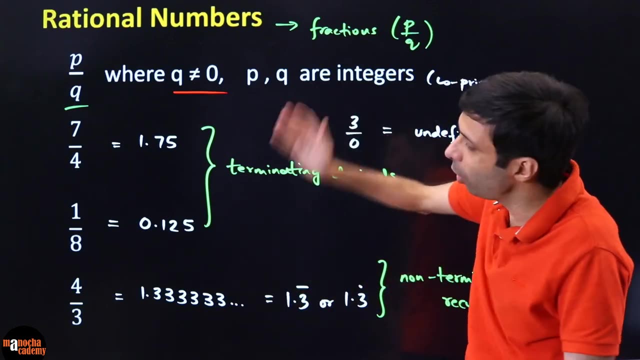 terminate, terminating decimal if you do the division, Or it can be not ending, non-terminating but repeating pattern recurring. Those are the only two possibilities. Nothing else is possible. Clear, So please write that in your book right now. Rational numbers means terminating decimal or non-terminating, never ending but repeating. 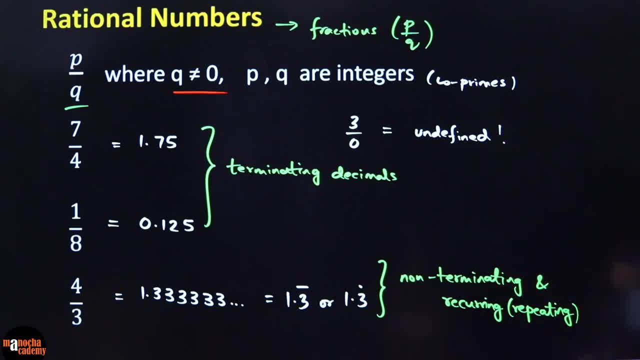 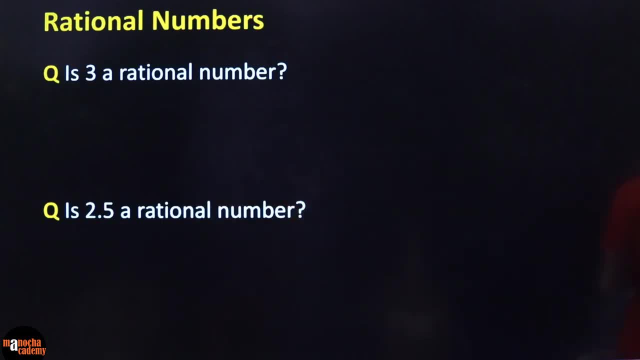 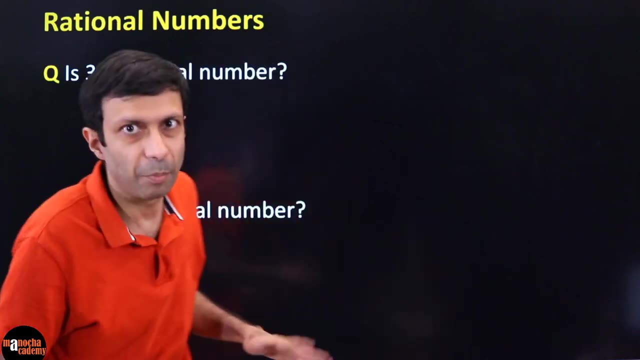 and recurring or and repeating. Have you guys written that? Please write it down. Now the question is: is 3 a rational number? What do you guys think, Yes or no? So I can see most of you are telling me yes, and you are absolutely right. 3 is, of course, a natural number, It's a whole. 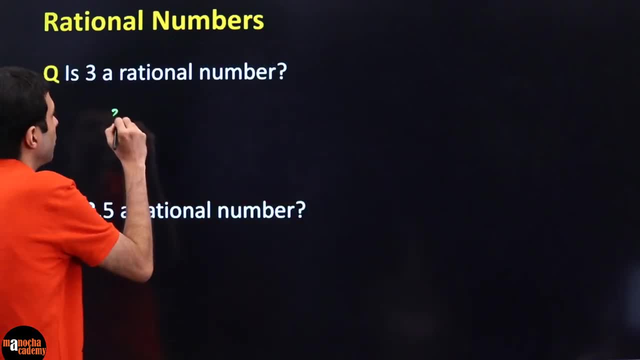 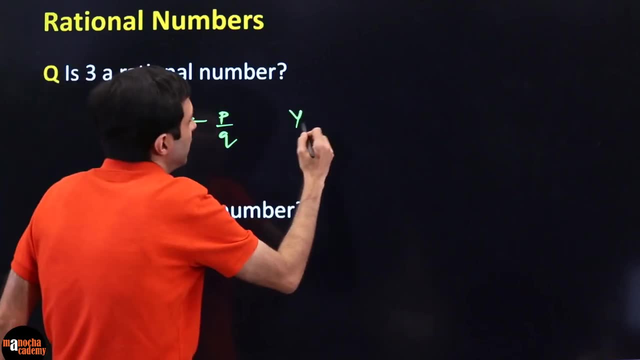 number. We can consider it integer. But why is it a rational number? also Because 3 we can. I can write it as 3 by 1 and there you go, I approved it to you. It's p by q. So the answer is yes. 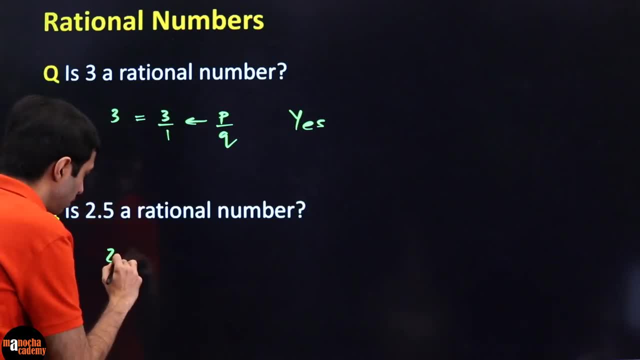 What about 2.5?? Is it a rational number? Again, same trick, See decimal. you can always convert to fraction. So there, 22.5 is 25 by 10.. Now it doesn't look nice, Math teacher will not like. 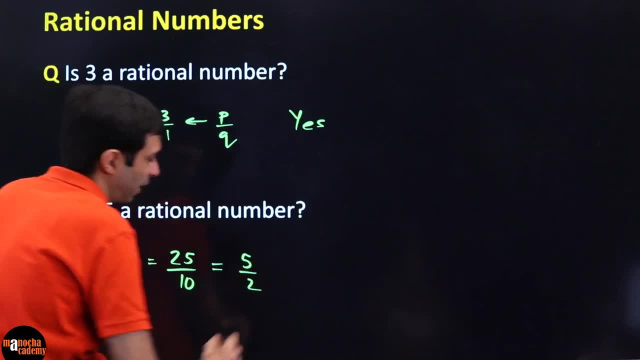 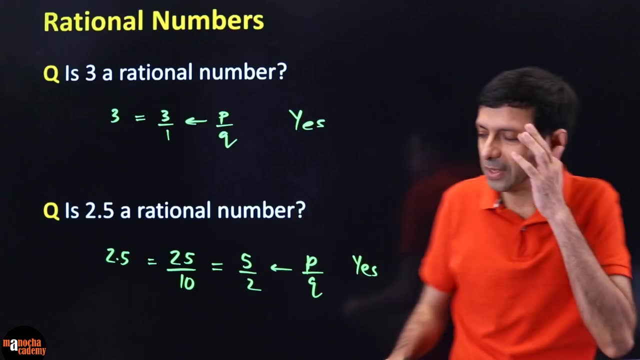 If you have not simplified it, So you should write no. no 5 by 2 will cancel by 5, and that is also p by q. So the answer is going to be yes, yes, yes. So if I can express it as a p by q form, 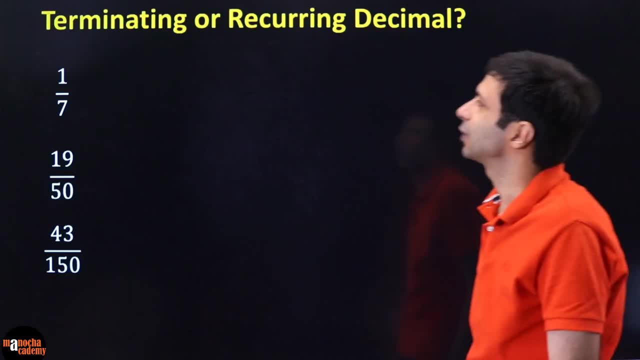 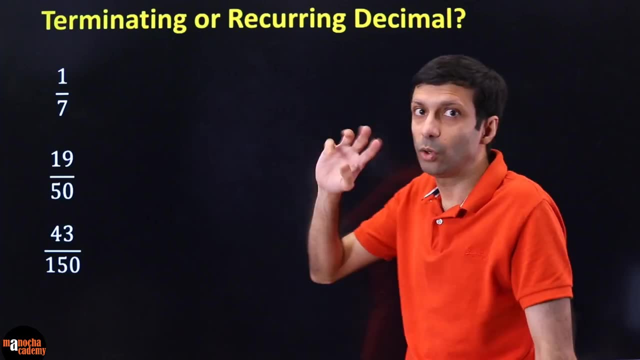 a fraction form. we are good. Now if I ask you this question, that, hey, I have given you some fractions. These are all rational numbers. They are all p by q. Now I am asking you because I told you rational number can be either terminating or non-terminating and recurring. So can you guys? 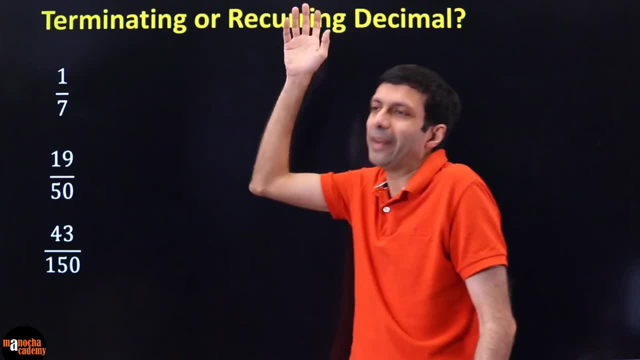 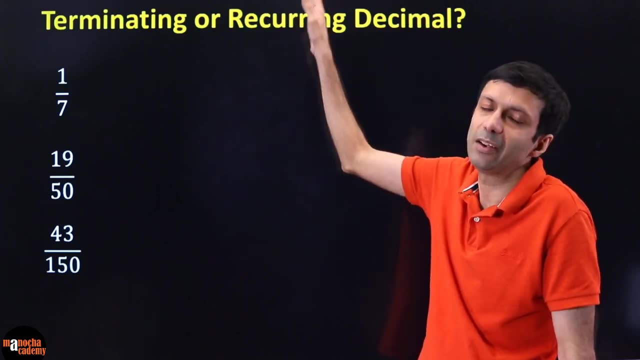 tell me, is this going to give me a terminating decimal? or by recurring I mean non-terminating right Repeating pattern means it is not ending, So sometimes you will see that non-terminating word is not written there, It is directly written: recurring. So can you tell me which of these are? 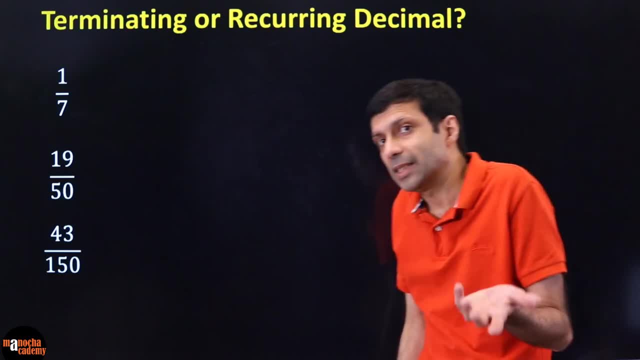 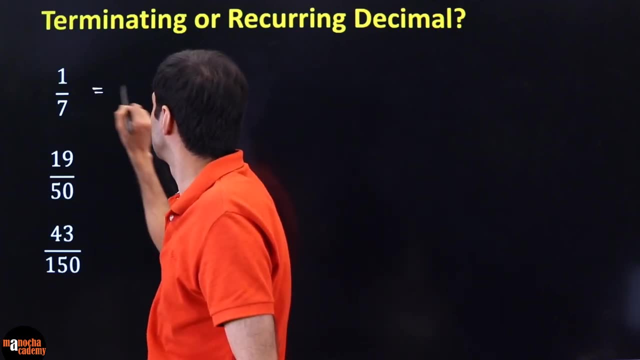 terminating or recurring. One very simple technique is sit and do the division. So if you sit and do the division 1 by 7, what will you guys get? So please sit and do the division. I am going to be a little lazy here and use the calculator. 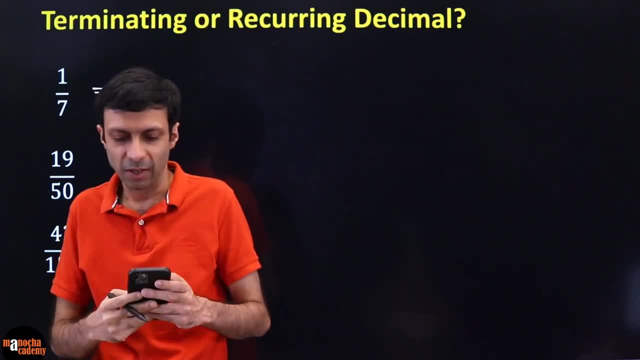 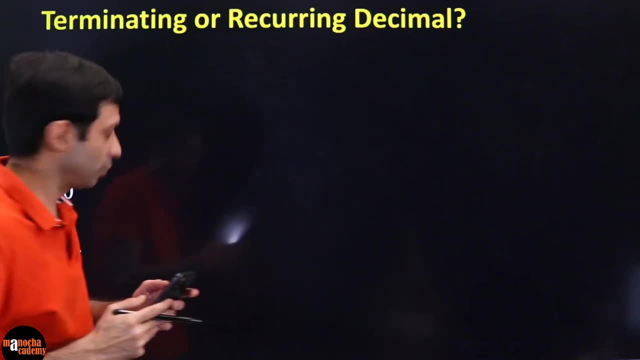 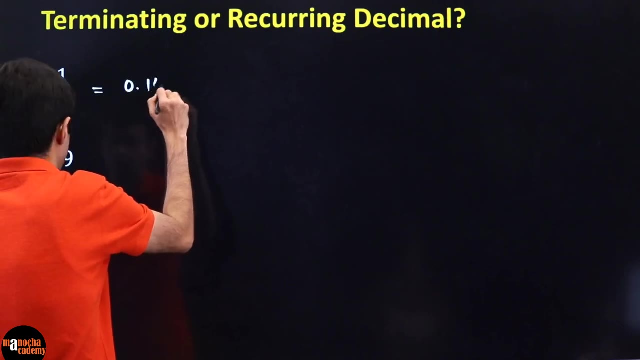 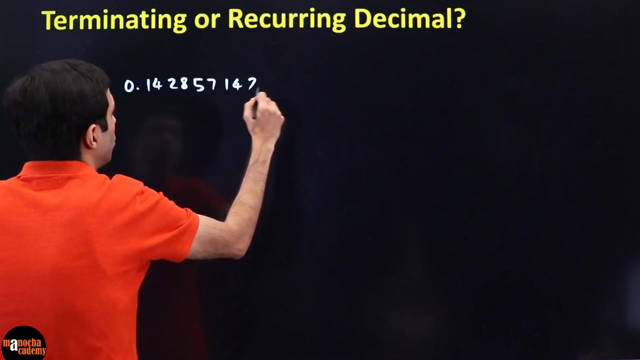 But you guys do not do that please. Very bad thing that I am showing here, But just to save time I am going to use the calculator. So if I use the calculator and I do 1 divided by 7, I am getting 0.142857142857 and so on. So what is this? It is not ending. 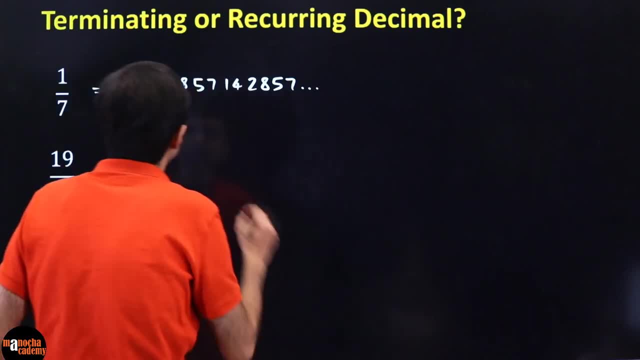 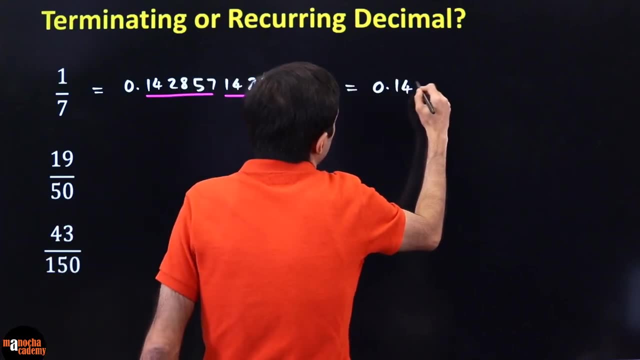 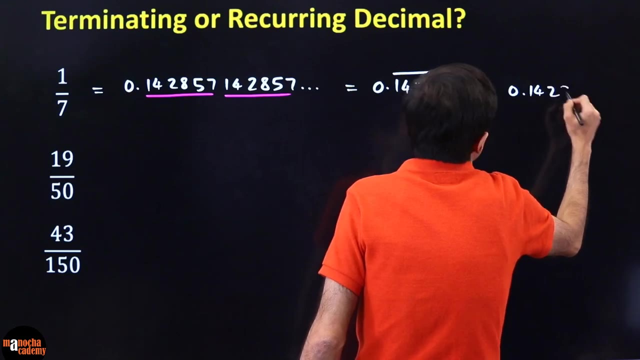 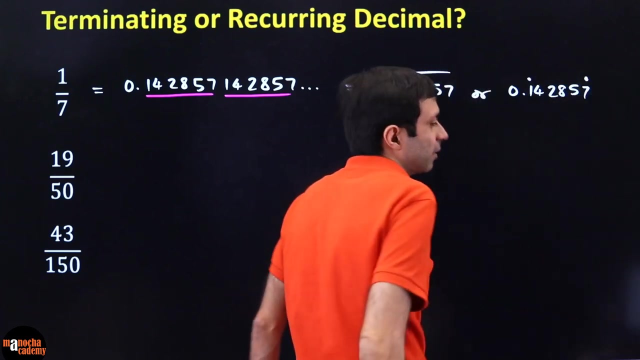 But can you see that there is a repeating pattern here? Can you guys see 142857142857.. So this I can write it as 0.142857 with the bar on top, or some books write it like this: 0.142857.. Since this whole part is repeating, we put a dot on top of 1 and a dot on top of 7.. 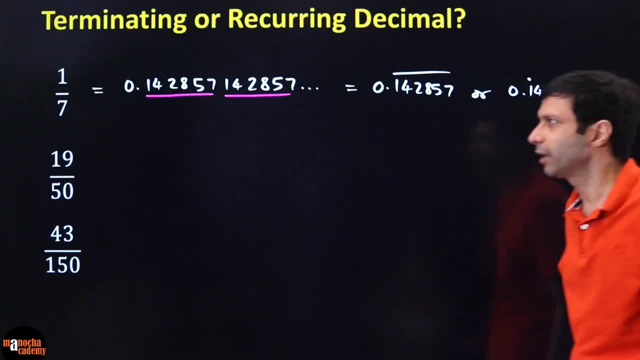 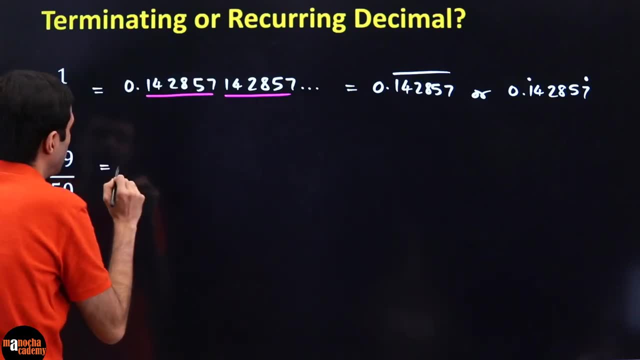 Is it clear. So that is one way you can easily check. Similarly, if you do the情况, 17 by 15, this one is easy to divide. In fact, I can show you a nice trick: if you have 50, you just multiply the numerator by. 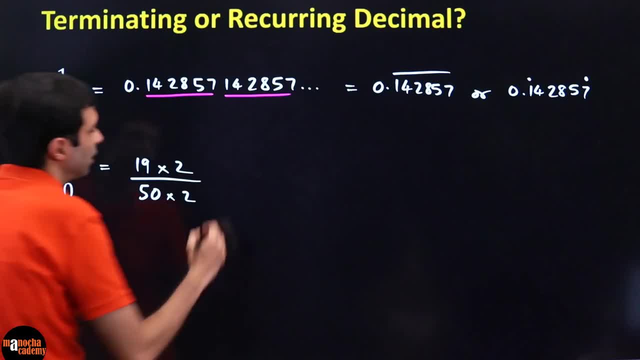 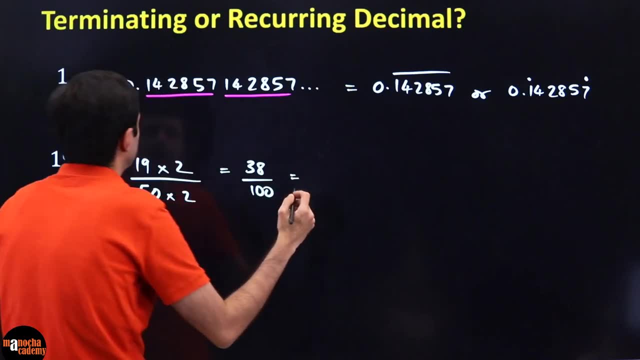 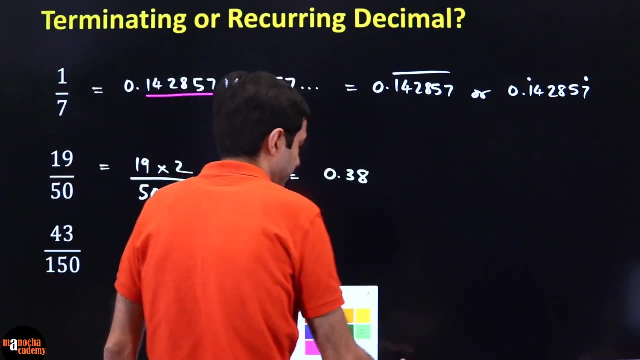 2 and the denominator by 2, because I have changed it to 100.. So what is 19 times 2?? 19 times 2 is 38 divided by 100, 0.38.. That is it. So what did we get here? Here, we got a recurring decimal terminating or. 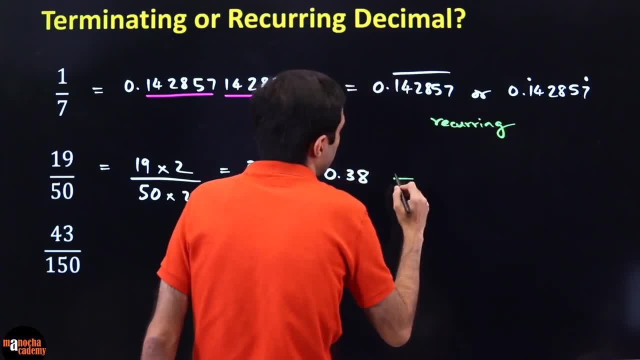 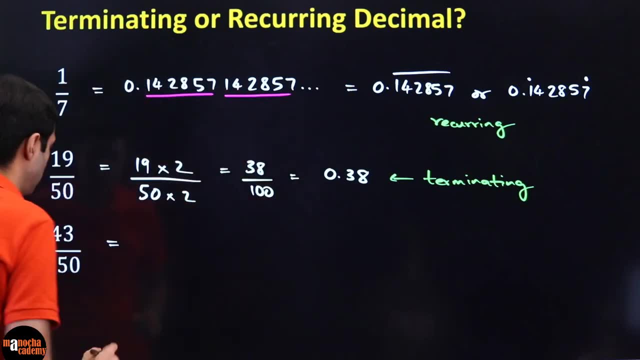 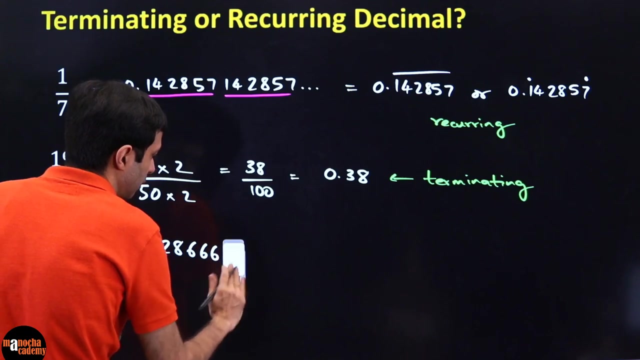 sorry, Non Terminating, not repeating and recurring. here we got a terminating decimal. what about the last one? 43 by 150. so please check it again. i'm going to be a bit lazy here and do the division 43 by 150 with the calculator and don't do this. i'm just doing it to save time: 0.28666666, it's just going. 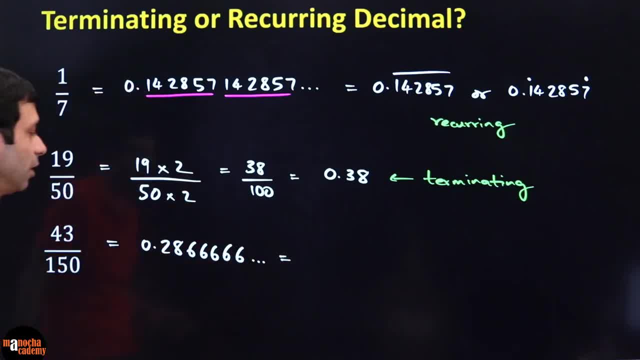 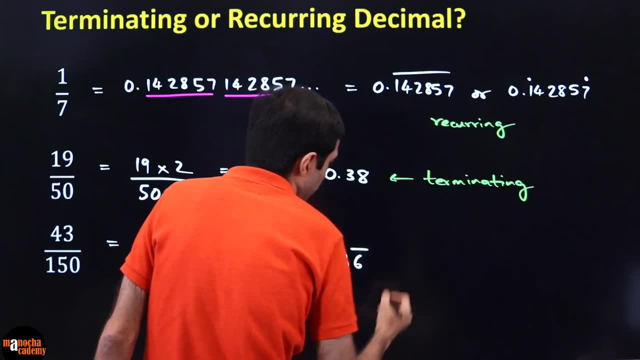 on and on. so it is clearly recurring, not, uh, not terminating, and you can see i will write it as 0.28. only the 6 is repeating, so we'll put a 6 bar, or we can say 0.286 dot. please don't put the bar, or. 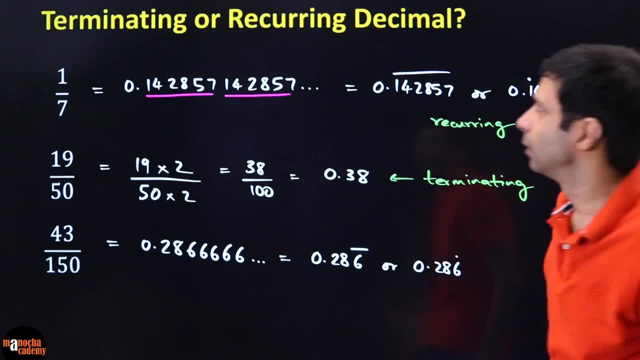 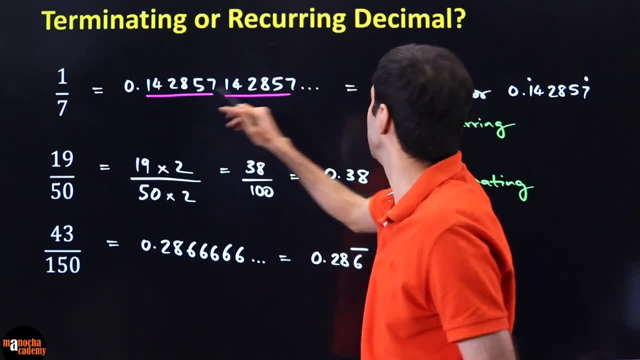 dot above 28, because that part is not repeating the first one. also, if you keep dividing, you'll keep seeing this: 142857, 142857. you keep doing it, it's keeping on repeating. so this entire pattern is repeating here. only the six part is repeating. so we write it like this. so this is also a non-terminating. 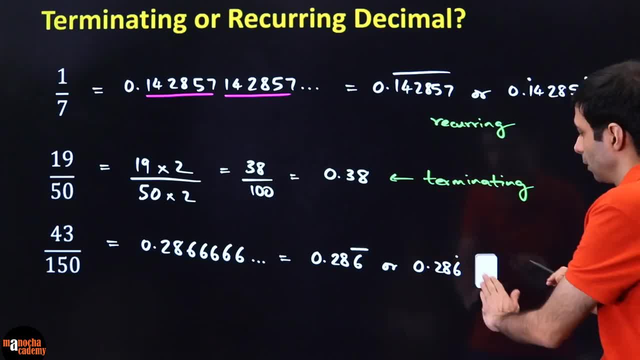 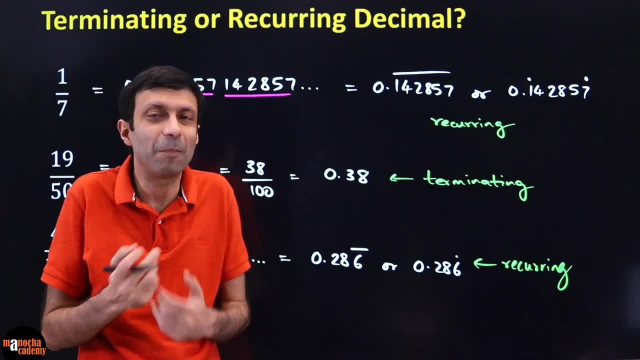 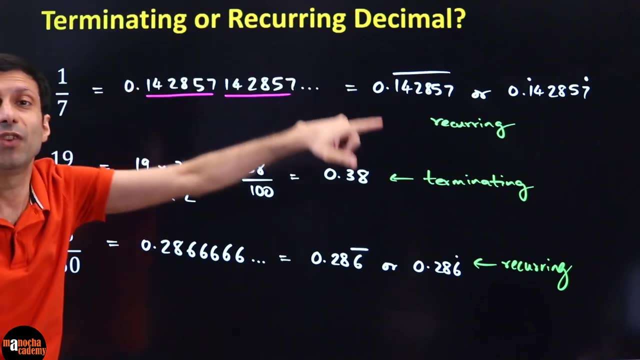 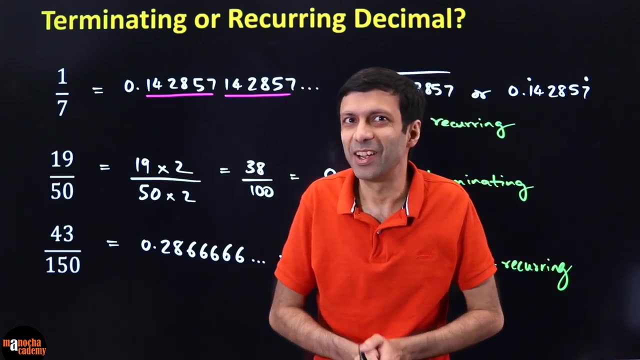 recurring, or we can simply write recurring, repeating pattern. do all of you agree with these answers? but this is time consuming, right? we are having to do division. is there some magic trick where i can give the answer of terminating or recurring even without division? is there some magic trick? the answer is yes, it is a very simple trick. what is the trick? you just 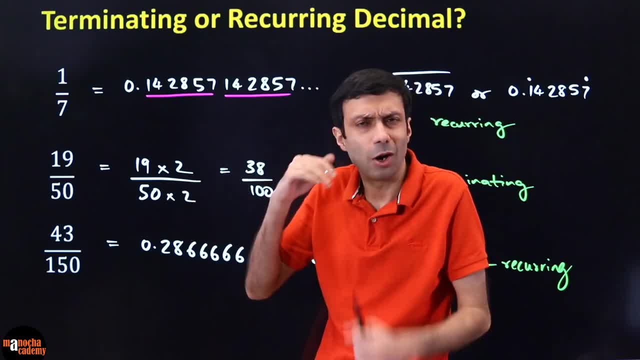 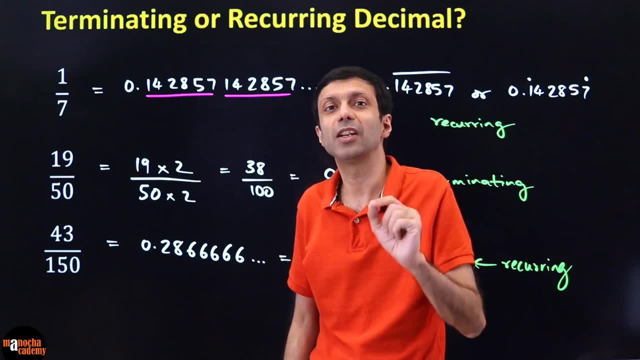 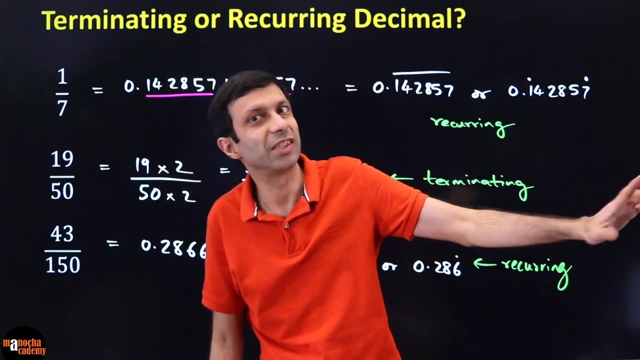 have to first have to look at the denominator of the fraction, not the numerator. don't even Look at of the fraction and check if it has factors of 2 and 5. only then it will terminate. otherwise all other fractions give recurring decimal answers. so what is the shortcut trick so you can say: 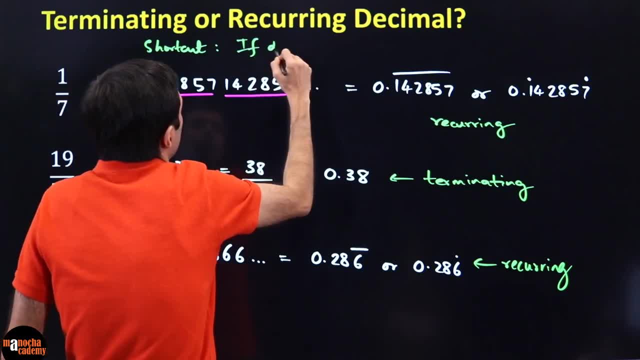 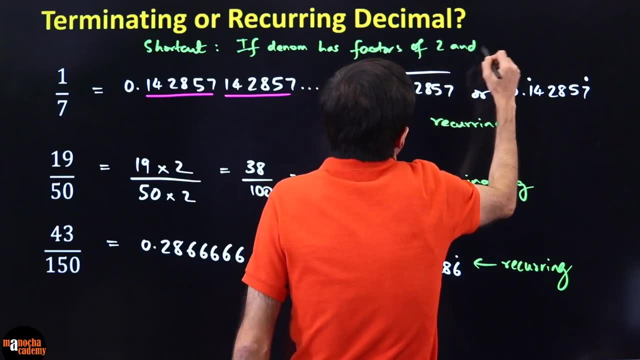 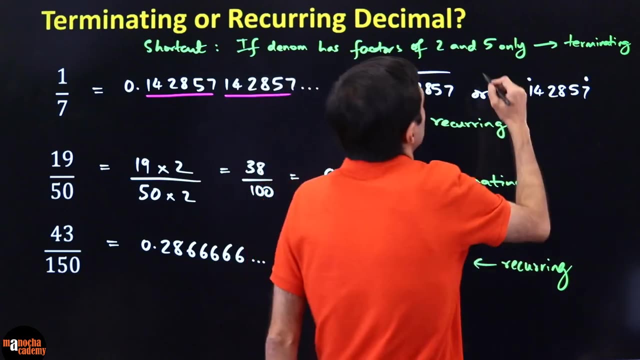 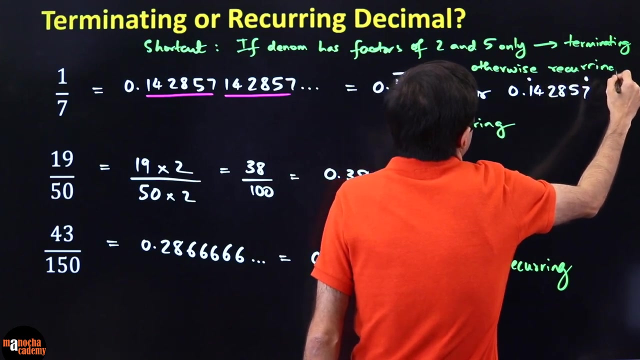 shortcut is: if denominator has factors of 2 and 5, only then it is terminating, otherwise it is, else otherwise not terminating. otherwise it is recurring, because in rational numbers you always get a non-terminating repeating pattern. is this clear to all of you? so that is. 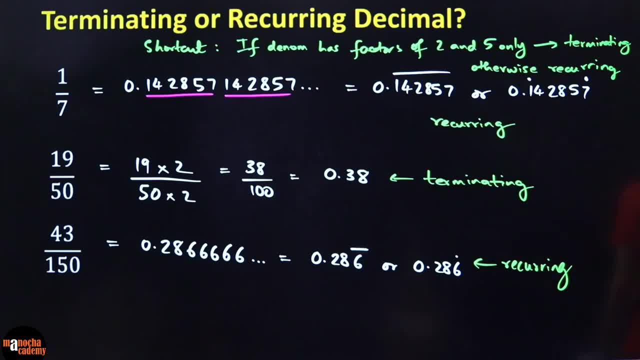 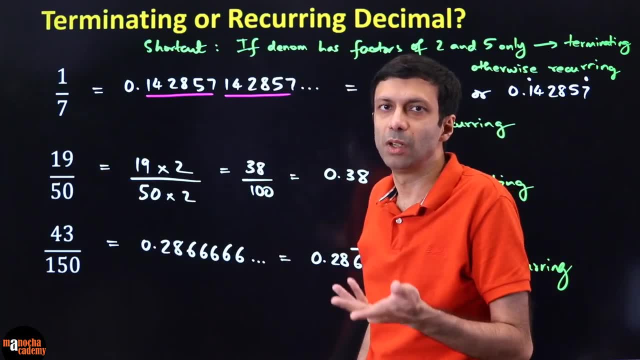 the quick trick. that's the check you have to do. so you guys can go and check that. so let's apply that trick here: 7. 7 is the denominator. is it having factors of 2 and 5 only? no, there's only one factor here: 7. it will be recurring. see, this is what we got: 50. what are the factors? 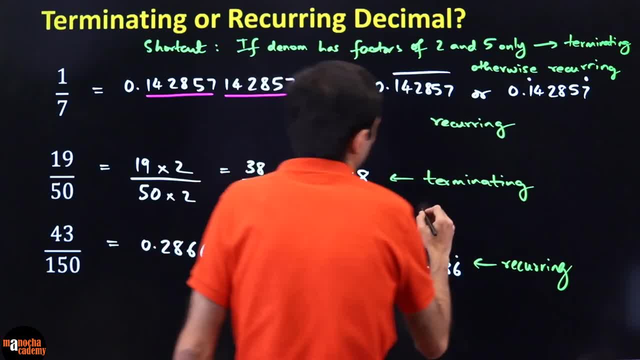 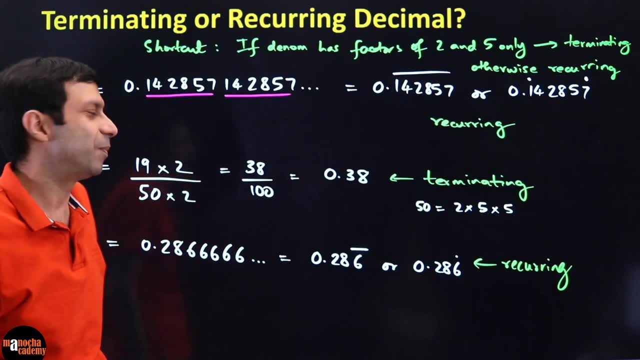 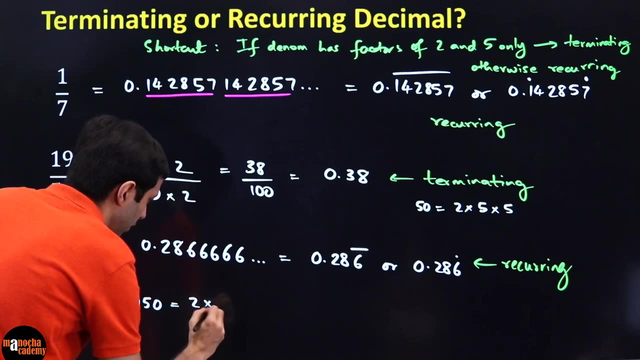 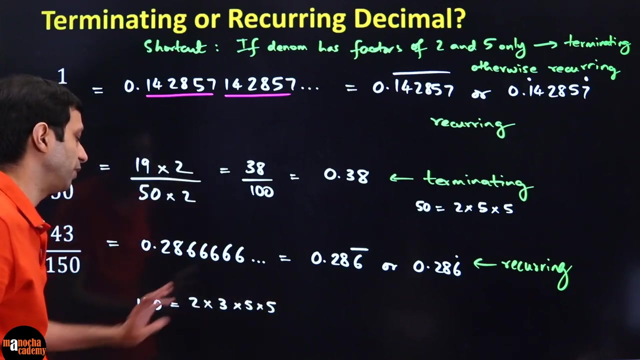 of 50. if you break down the factors of 50, you can see 50 as the factors 2 times 5 times 5, factors of 2 and 5, only terminating 150. what are the factors of 150? we have 2 times 3 times 5 times 5. check it: 25 times 250, 50. 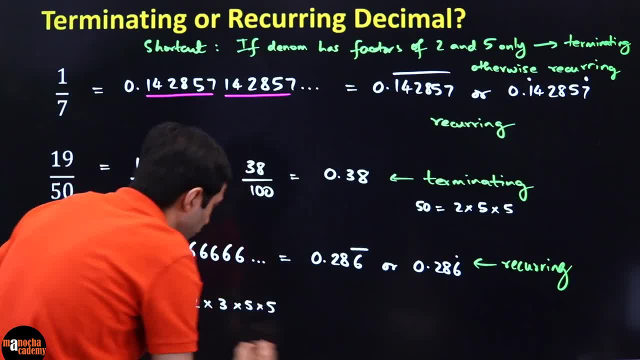 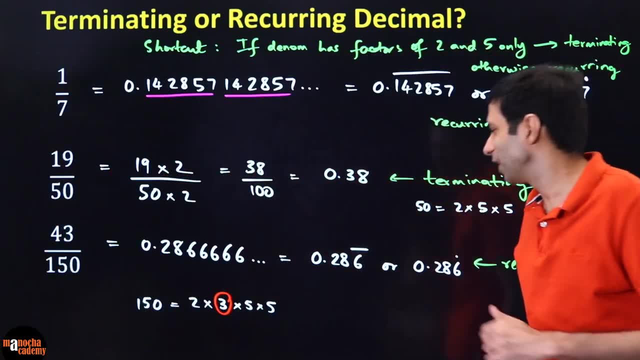 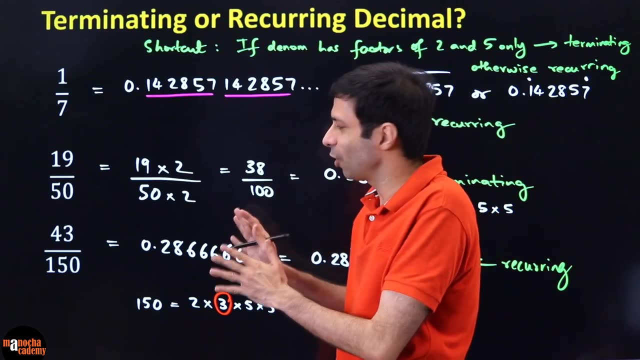 times 3 is 150, but the problem is factors of 2 and 5. only there are 2 and 5 factors, but 3 is also there. this Mr 3 has spoiled it right and that is why it is giving a recurring decimal number. so this is the simple magic trick. all you have to do is just check the denominator. you don't. 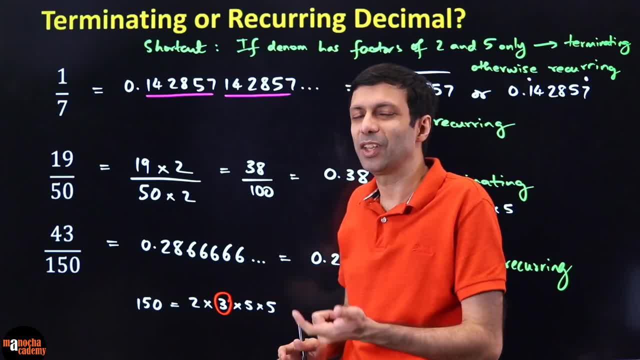 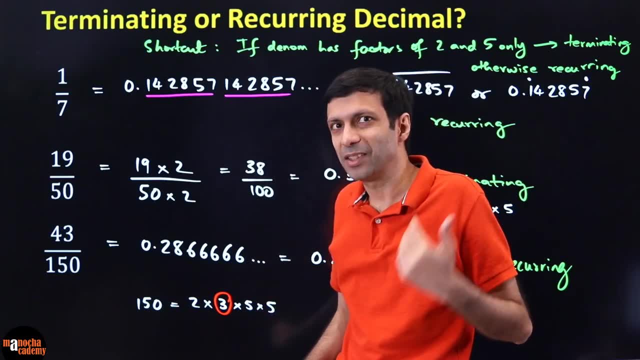 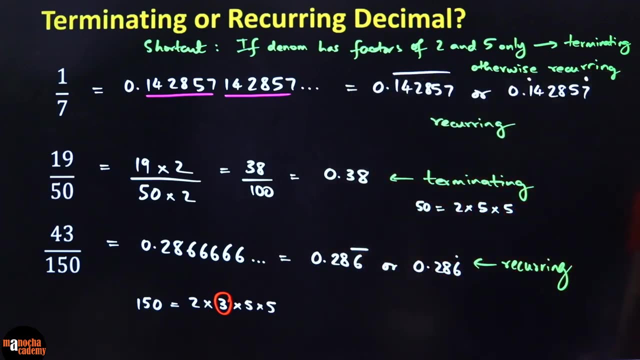 have to do all that division. no need of calculator, just check if the denominator has factors of two and five, only terminated if it has more. if it has other factors, it is recurring crystal clear. is this magic trick clear to you? and yes, that is why in many of the books this trick is written. 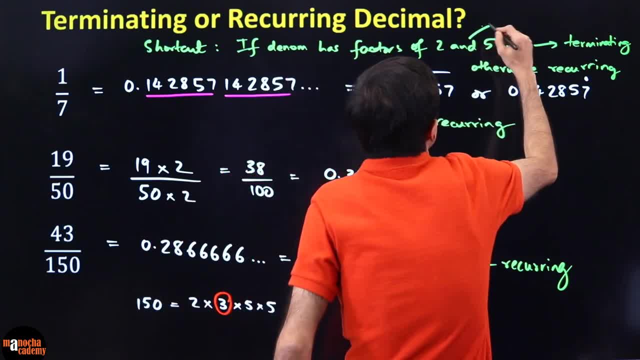 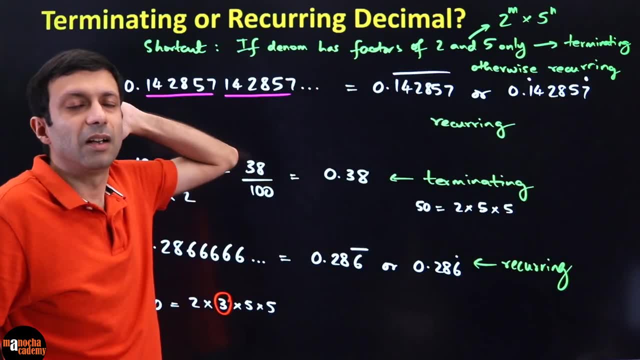 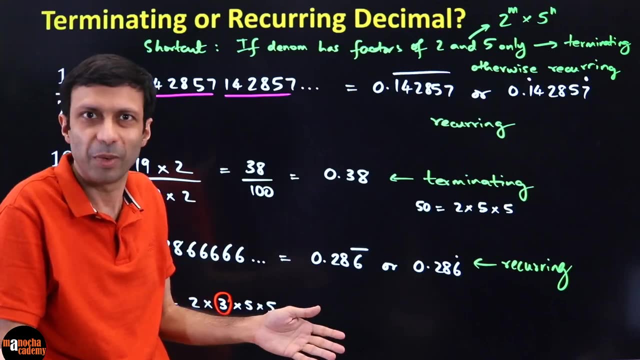 like that, that two and five only. they write in the book as two to the power m- very good- and five to the power n, basically saying that, hey, the denominator should be only two to the power, so it doesn't have to have two and five. it could be only twos like half one. fourth, these are: 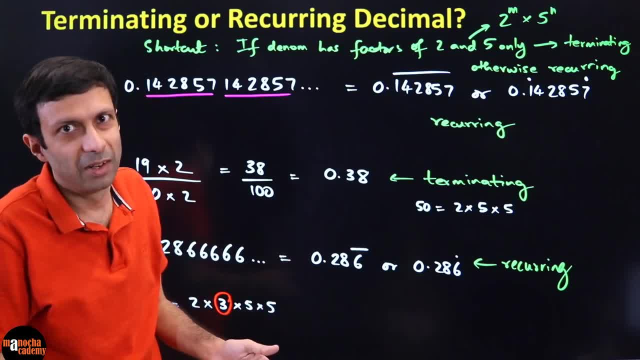 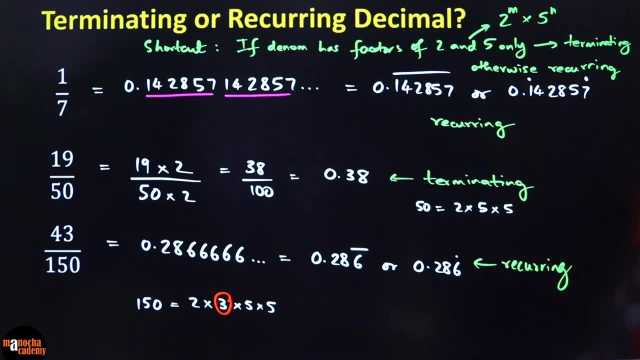 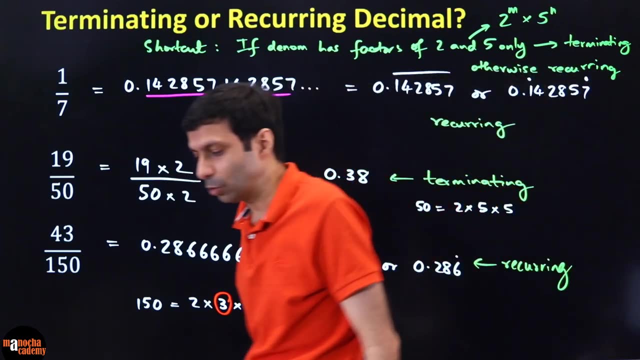 terminating, one by five, one by twenty five, also terminating. so it doesn't mean it has to have two and five, but two and five only, nothing more than that. okay, ankit shah, is that correct? so ashmit is asking: is non-terminating and recurring the same? no, it is not. we are coming to that. there are some. 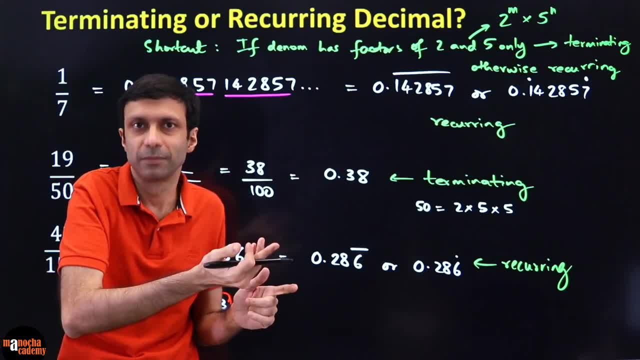 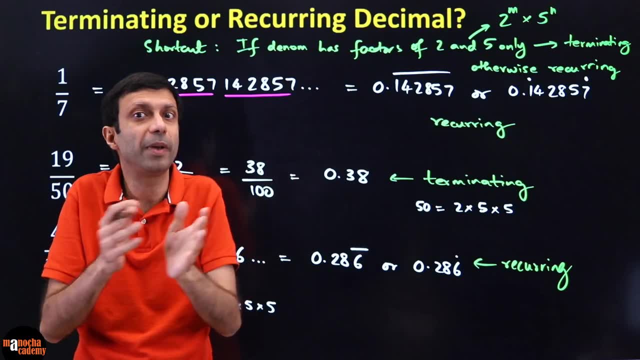 decimals which are non-terminating and recurring the same. there are some decimals which are non-terminating, but they don't repeat. okay, there can be decimal numbers which are non-terminating, like pi, they never finish, but there is no repeating pattern. we still haven't found any repeating pattern. 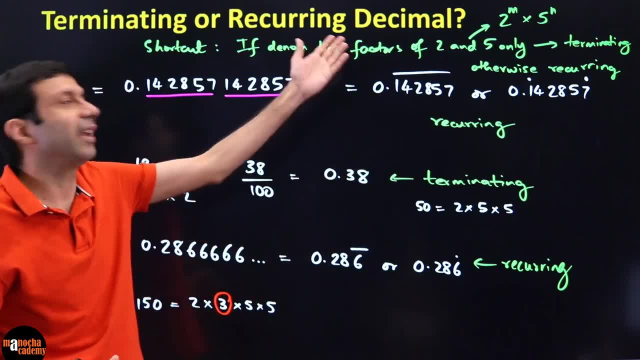 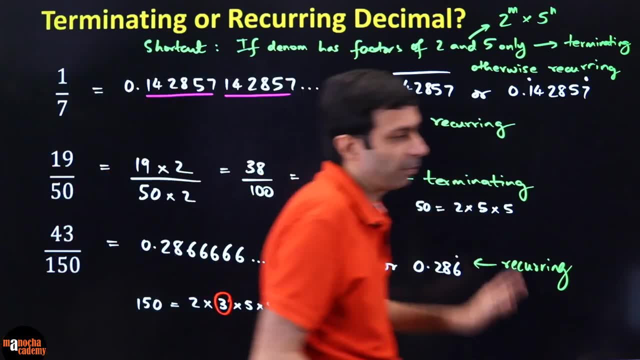 okay, but when we say the word recurring- repeating- it has to be a non-terminating. you cannot say, hey, this is a recurring decimal, because it stops. there is no repeating pattern. okay, exactly, they are irrational numbers. ankit shah, correct, we are coming to that. 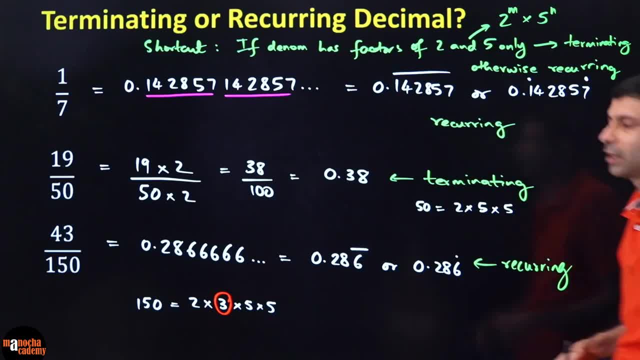 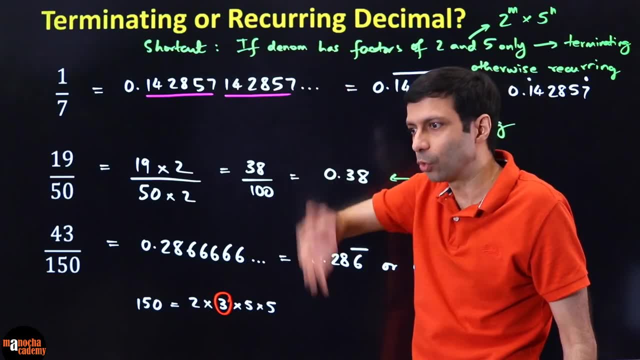 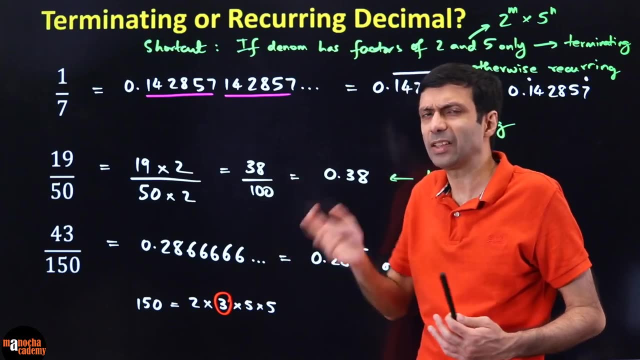 if the denominator has factors. so you find the factors of the denominator. if it has factors of two and five, only then it will terminate. it could have factors of only two or only five or both. two and five basically means only two, only five or both. but if it has some other factors, like three, 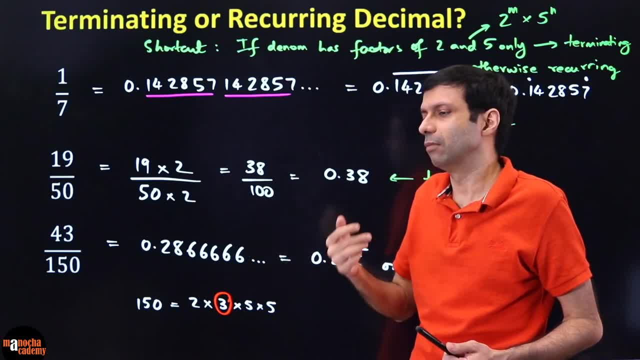 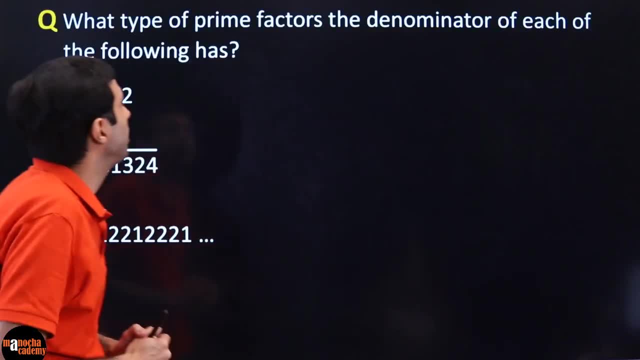 seven. you know prime factors, of course, or you know 17, 11, then it will give you a recurring and you guys can check that. so this is another related question: what type of prime factors the denominator of each of the following has. so this is the reverse question we have given you. 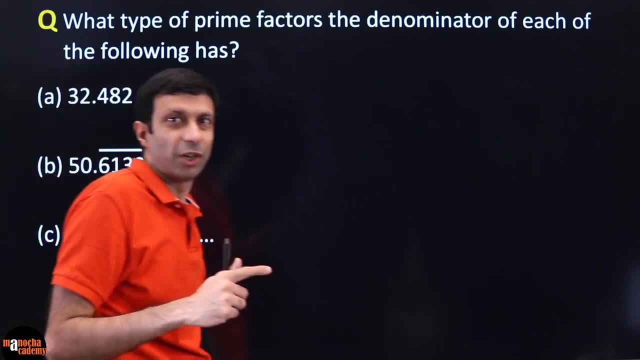 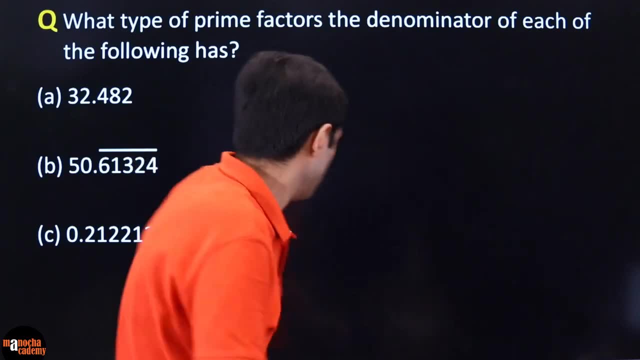 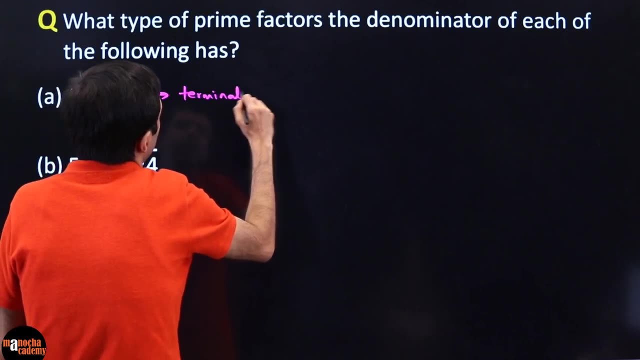 the decimal numbers. here you have to tell the prime factors of the denominator. so we can use that trick, because we had learned that if it is terminating like this guy is terminating right. so if you look at this fellow, this is clearly a terminating decimal. now because it is terminating. 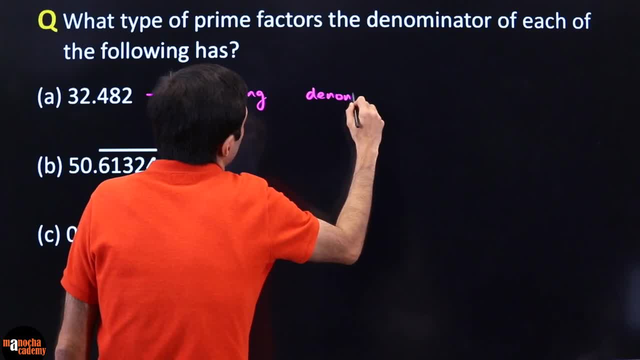 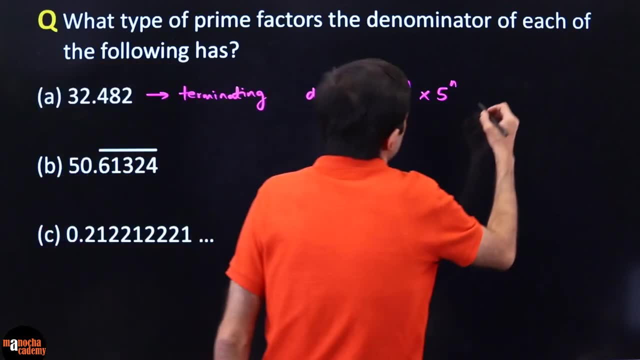 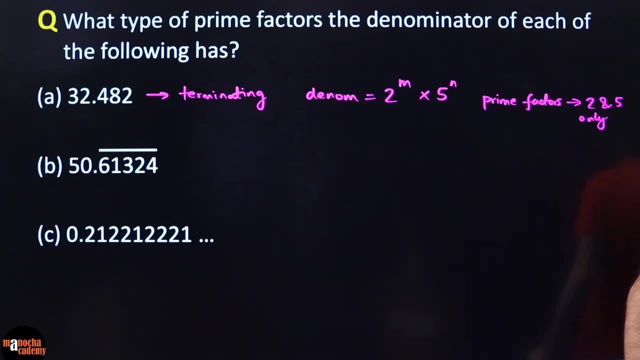 so we can say the denominator is of the form two to the power m, five to the power n. what does this mean? only multiples of two and five. so we can say prime factors of the denominator are two and five. only that's it clear. now what about this one? 6.1324. but you can see there is a, a bar. 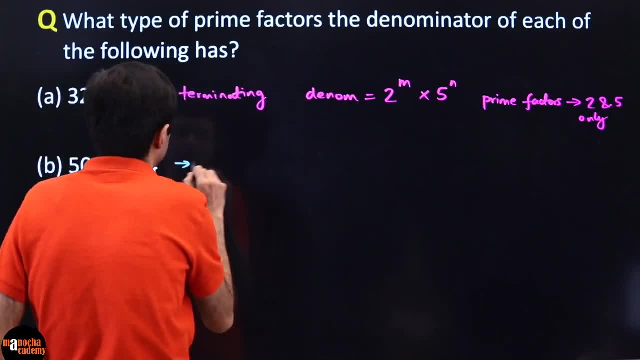 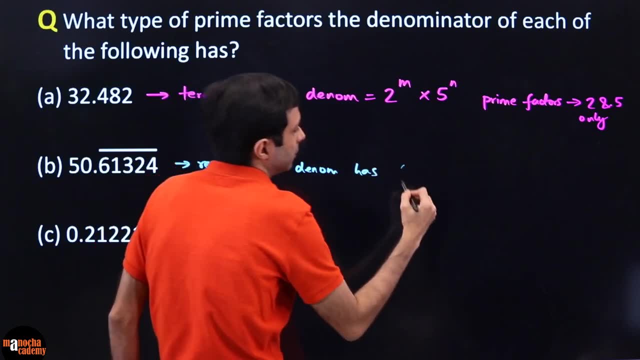 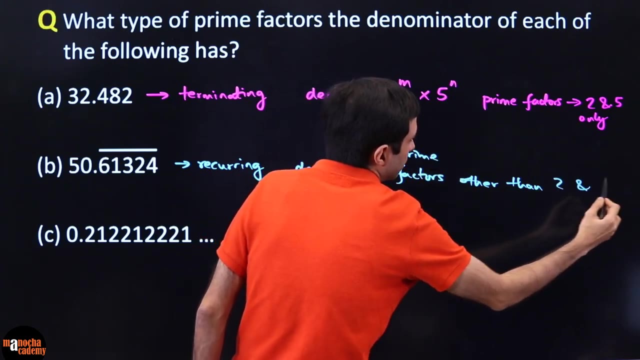 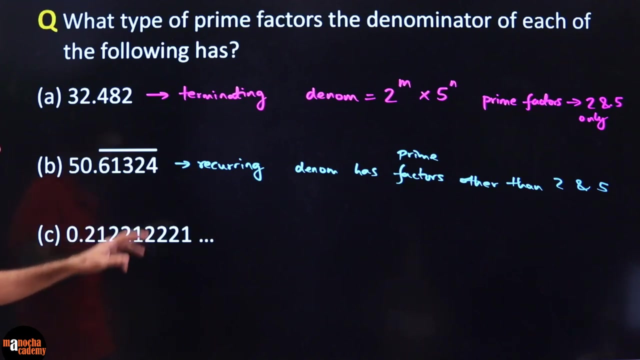 here. that means this is clearly recurring, repeating. so therefore, denominator has factors other than, or prime factors other than, two and five. yeah, it has to have some more factors. what about this? one point two, one, two, two, one, triple two, one. what about the last one? the problem here is that there is no. 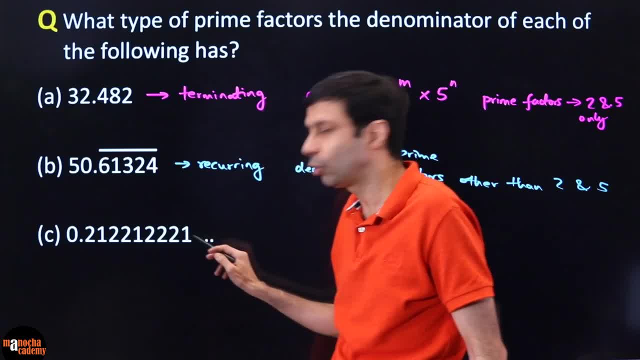 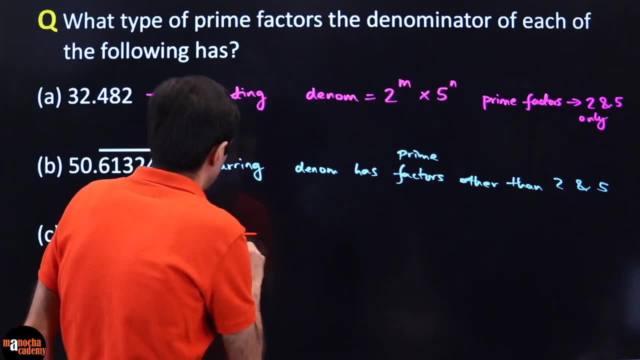 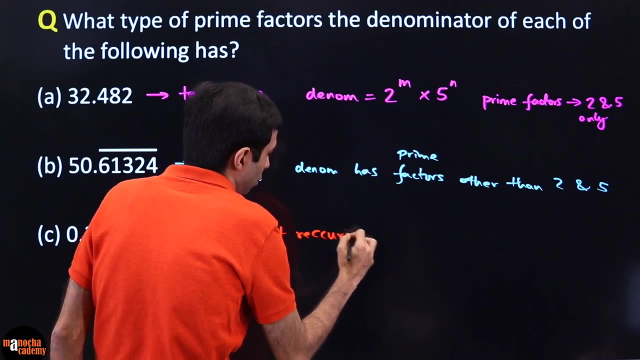 repeating pattern, because 21, then you have two, two, one, then you have triple, two, one, so there is no repeating pattern. so what is the problem here, this guy? we say it is not recurring, it is non-terminating, as you can see, it is never ending, but it is not recurring. so therefore it is not a rational number. 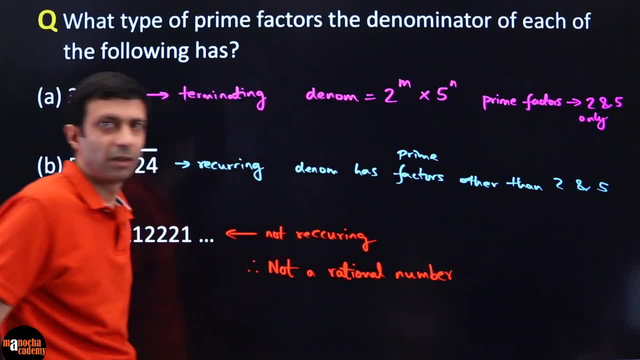 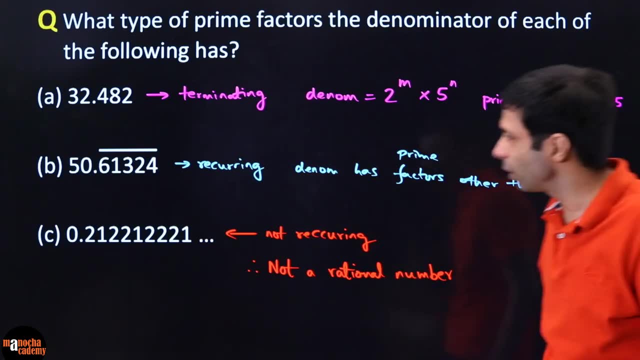 if it is not a rational number, is there any question of a denominator? is there any question of p by Q? if it is not a rational number, what do you guys think? so, because it is non-terminating, not recurring, so there is no question of a. so you know, question of denominator does not arise here. 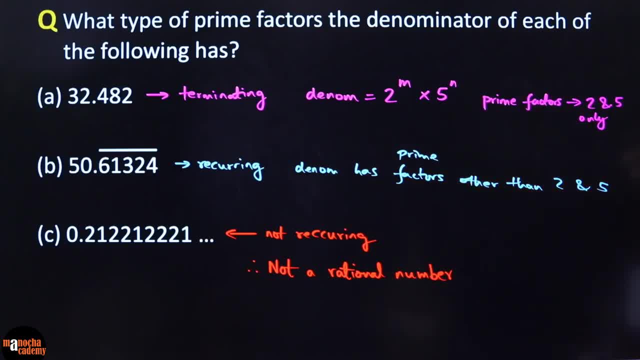 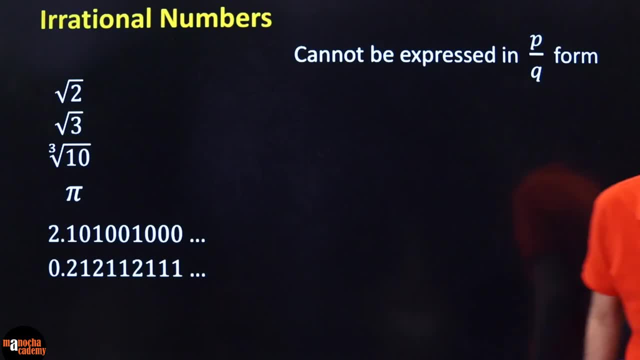 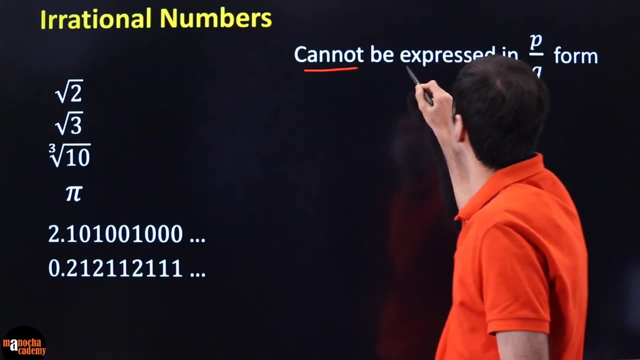 so this is like a trick question. it's like none of these. right next, let's talk about irrational numbers. so we've all been talking about rational numbers. let's get a real. let's get a bit irrational right now. what are irrational numbers? those numbers that cannot be expressed in a fraction form. you can't express it as a p by q. no, there is no magic. 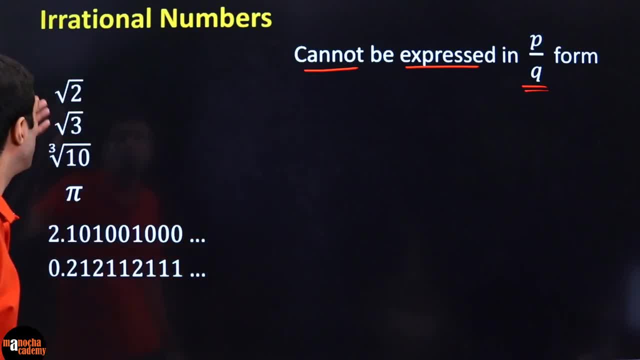 fraction that will express what are some examples: square root of 2 root, 3, cube root of 10 pi and the one the examples we discussed. right, if you have decimal numbers which are non-recurring, that means there are. they are clearly irrational, okay, and you guys can check this if you look at 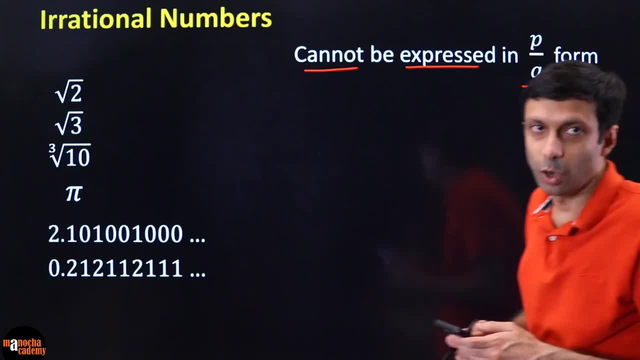 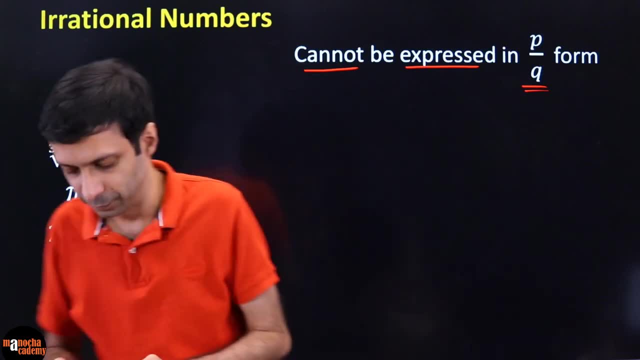 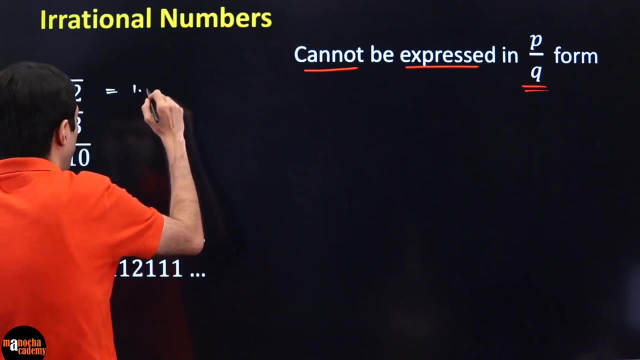 the value of root, square root of 2. what is the value? obviously this: i can't calculate a very accurate value, so i'll have to use the calculator here. so, square root of 2, square root of 2, if you look it up in the calculator, if you want to see many decimals, is 1.4. you might remember. 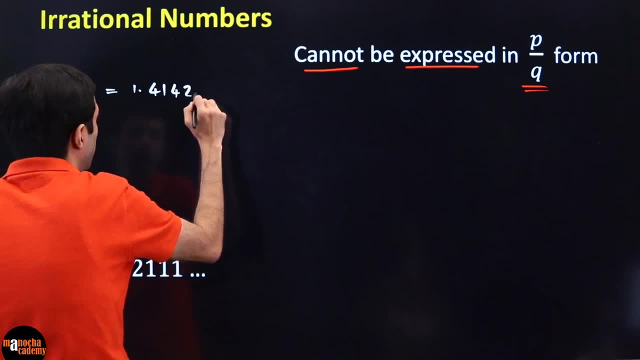 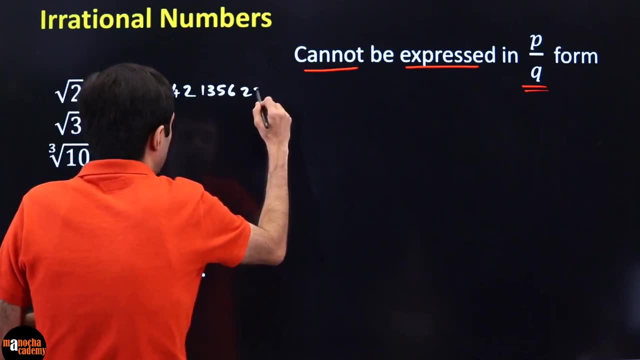 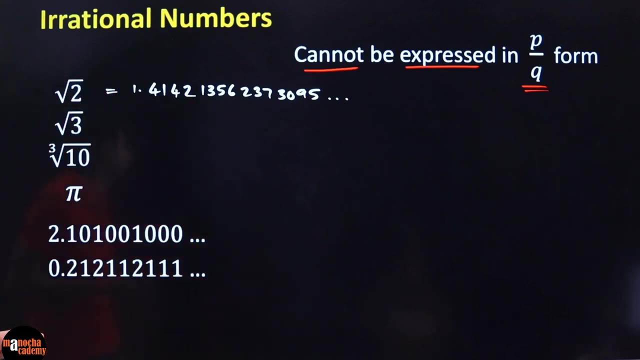 1.414, but it doesn't end there. 1.414213562373095. it's like one long phone number or something right, but the problem is there is no repeating pattern. it is non-recurring same thing. if you look at root 3, you guys check, can you find any repeating pattern here? you'll get a nobel prize for sure in. 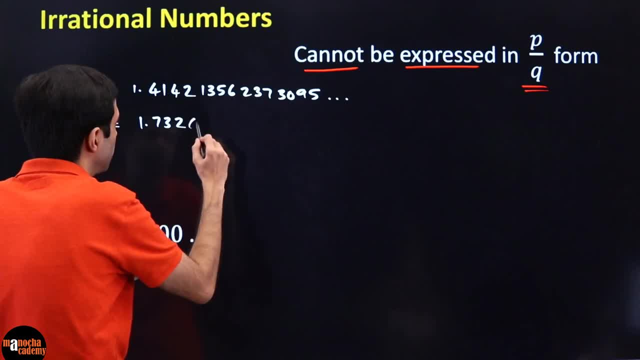 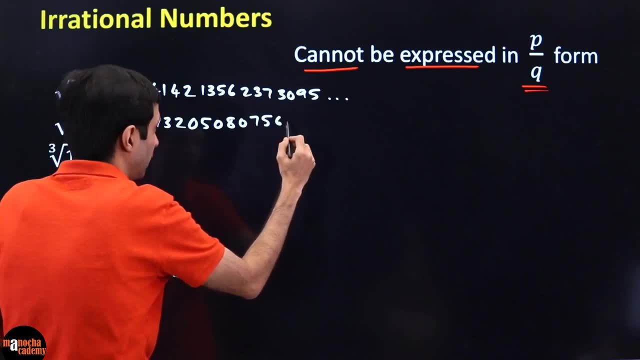 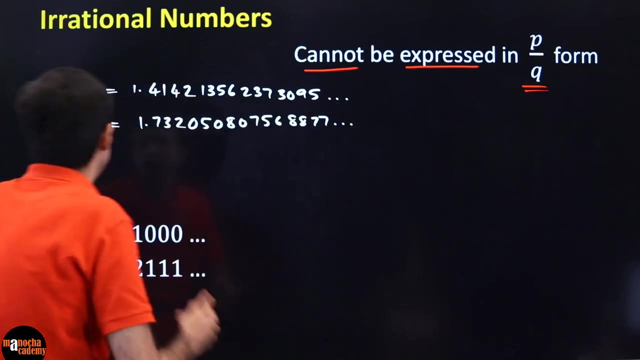 mathematics, we know root 3 is 1.73, but that's only the approximate value. there is 050807. wow, so many zeros, 568877. see, is there anything repeating here? and this is not just the end. you can go on and on right same way for these. 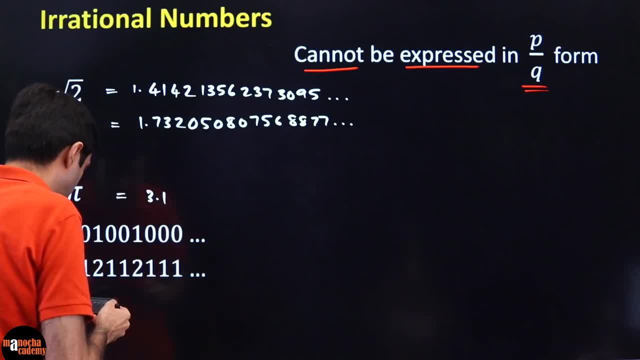 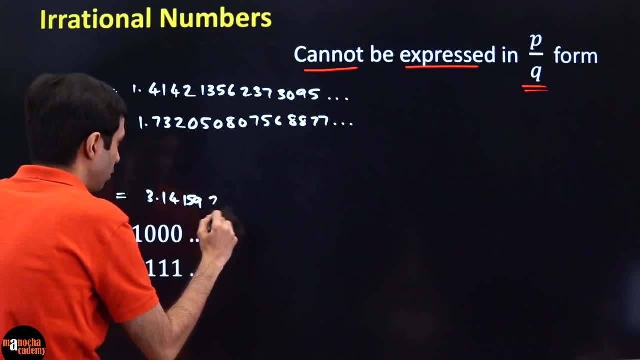 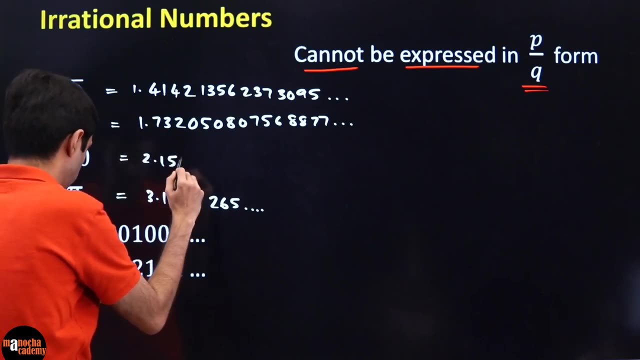 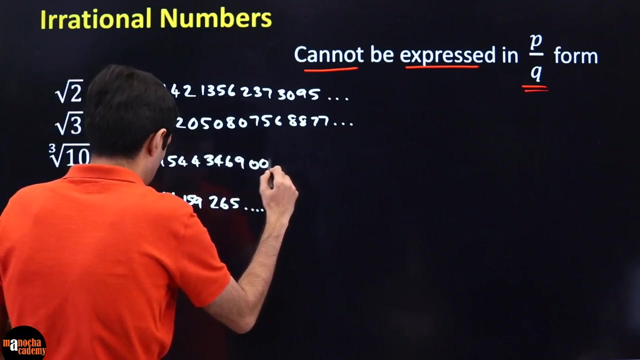 things. and pi also 3.14159. right, it doesn't end 3.14159265 and it just goes on and on and on. cube: root of 2. what is it? 2.154434690031884. i think you guys get the point. what is happening? 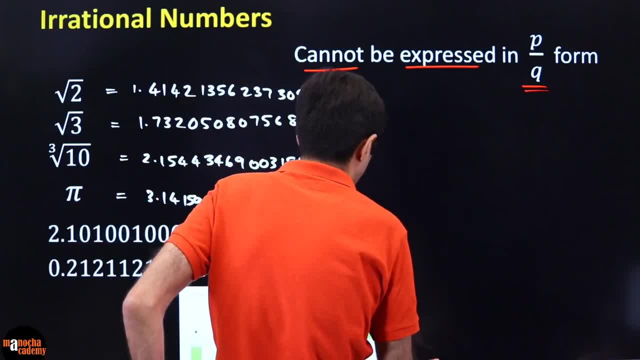 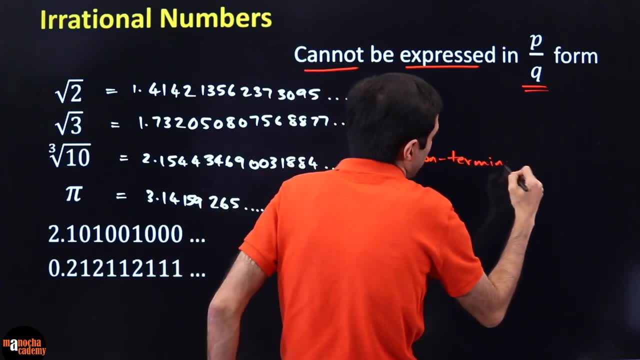 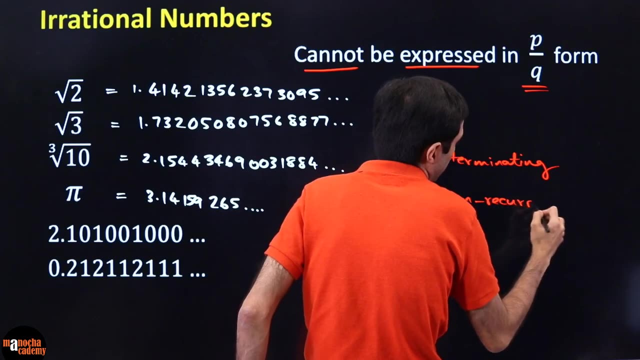 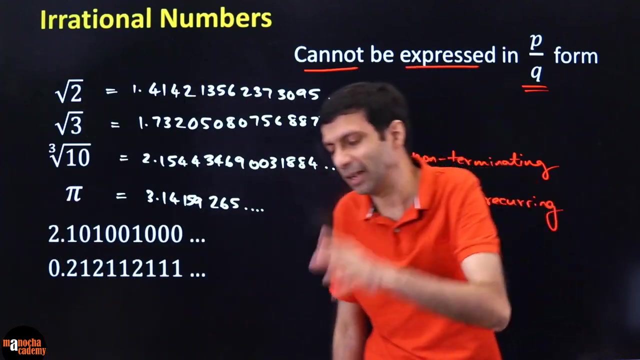 over here. these are all. all these numbers are non-terminating. the decimal number never finishes, it just goes on. your division, your job never finishes, there is no repeating pattern. that is why these are irrational numbers. rational numbers are of two types. again i'm reminding you. please be clear. rational numbers terminating, nice decimals. they 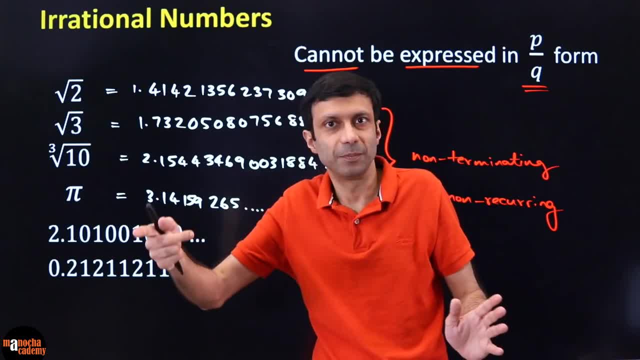 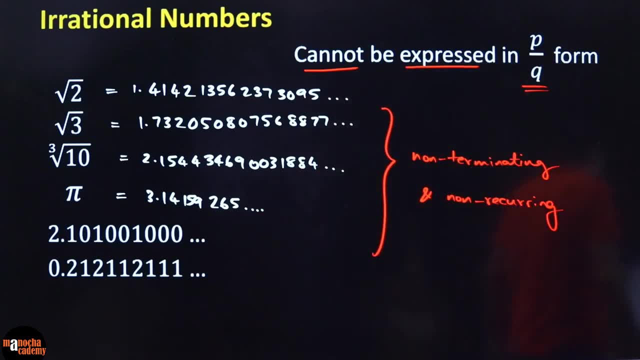 finish off or they are non-terminating. but repeating opposite is irrational numbers. they are non-terminating and non-recurring. is this crystal clear to you with these examples? so which of the following numbers are irrational, can you guys tell me? so one nice thing about the 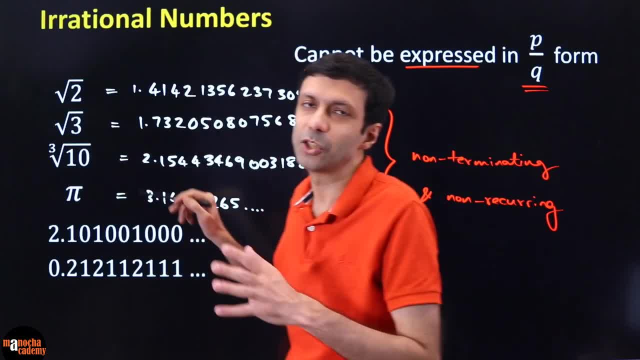 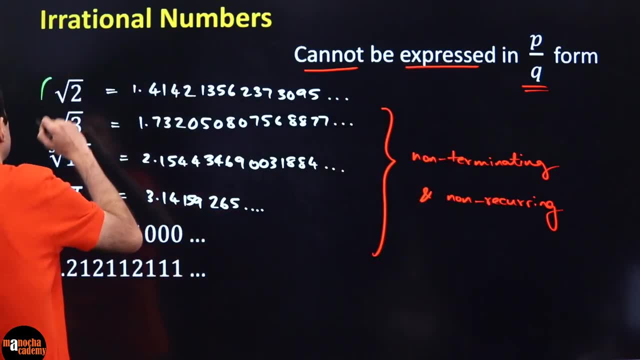 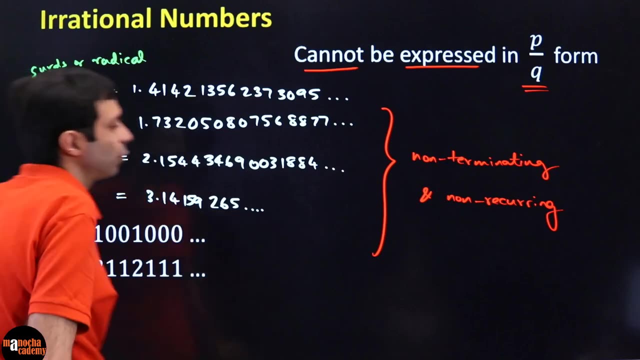 rational numbers are all these square roots. these are called surds or radicals. these are usually irrational, right? so all these roots which are known as these are all called surds or radicals. but this doesn't mean does every certain radical have to be irrational. why don't you check? 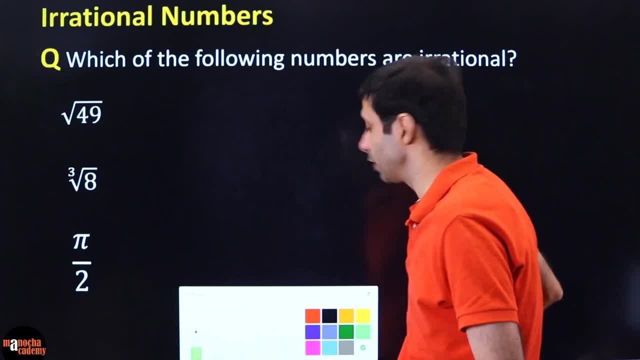 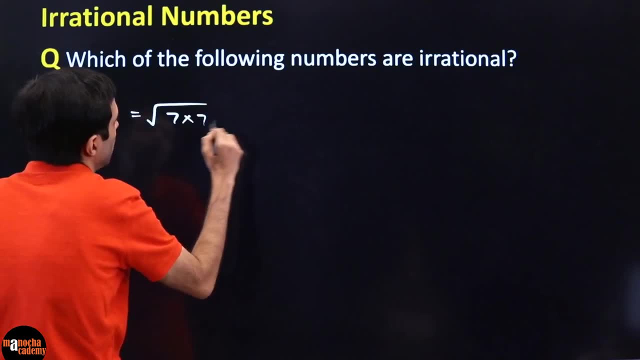 so is square root of 49 irrational. don't look at the square and say yes, because we know square root of 49 is square root of 7 times 7. so the answer is 7 times 7. so the answer is 7 times 7. 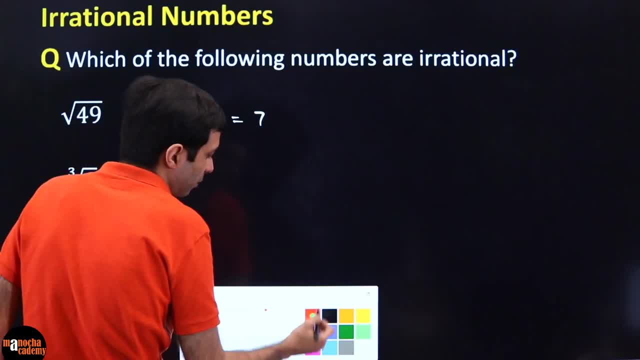 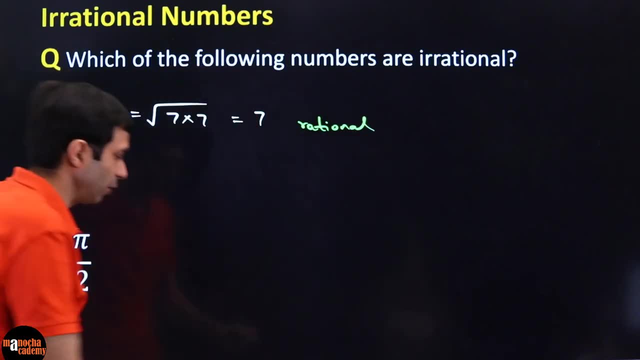 is 7 then. So that is definitely a rational number. So this is rational. What about cube root of 8?? Again, do not see the cube root and get excited. You should simplify it. It is a cube root of 2 times 2 times 2.. It is not that I saw the cube root irrational. No, no, no Again. 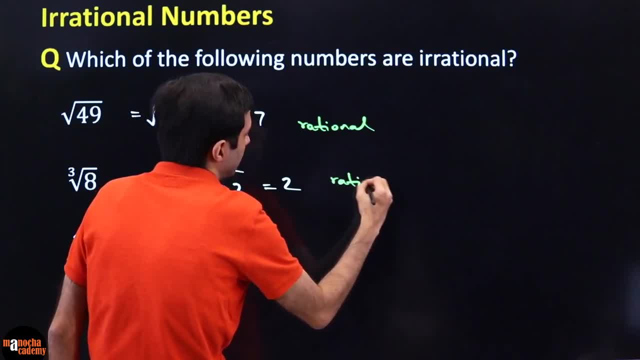 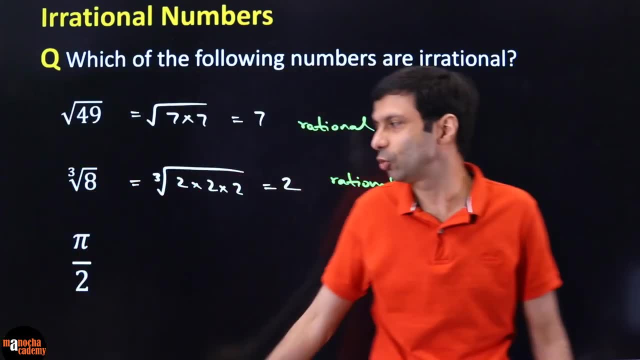 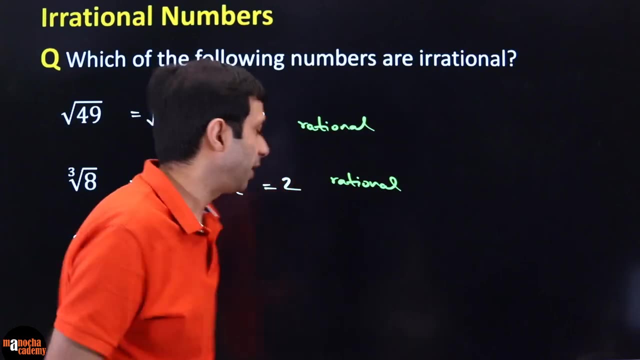 the answer is 2.. This is simply a rational number. What about the last one, guys? Pi by 2.. Can you guys tell me, is pi by 2 rational or irrational? So how do we know this answer? Pi is irrational, It is non-terminating, and if you divide that by 2, please do not take pi as 22 by. 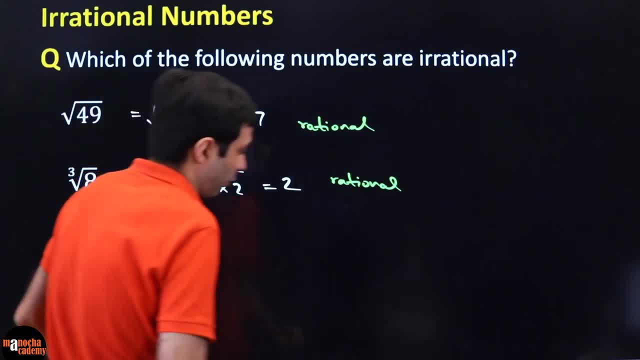 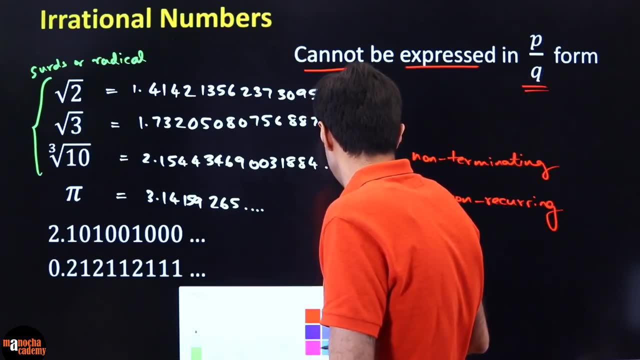 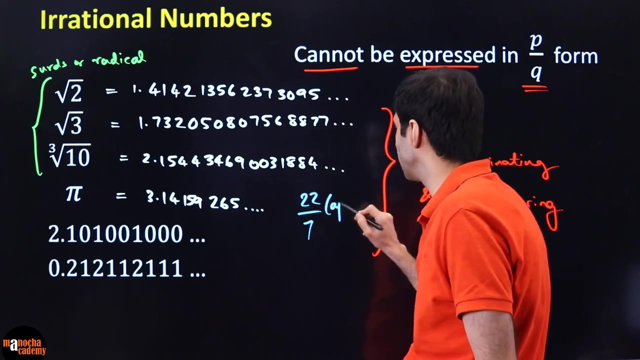 7.. That is only the approximate value. Yeah, I forgot to mention that many of you might be thinking that hey, pi is 22 by 7.. So this confusion is there. Sometimes you think, oh, pi is 22 by 7.. But no guys. 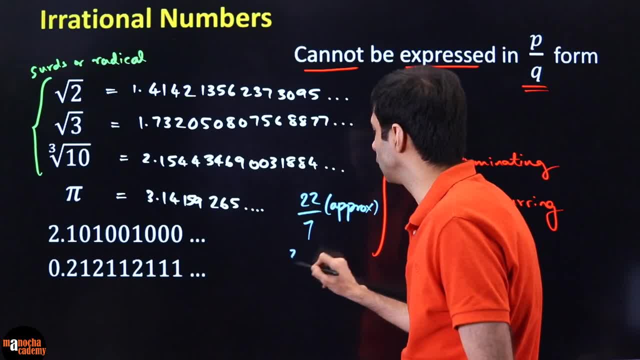 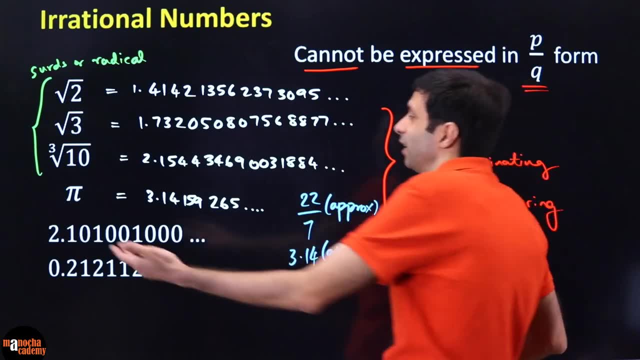 that is only the approximate value. Or sometimes you think, hey, pi is 3.14.. That is only the approximate value of pi. The real value of pi, as we discussed in that first slide, is this big, huge, massive number which never ends. Scientists have not found, mathematicians have not found an. 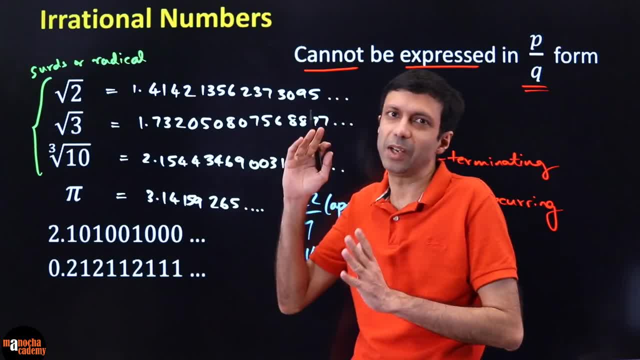 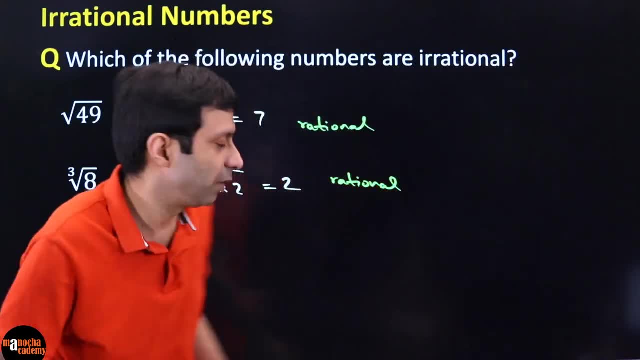 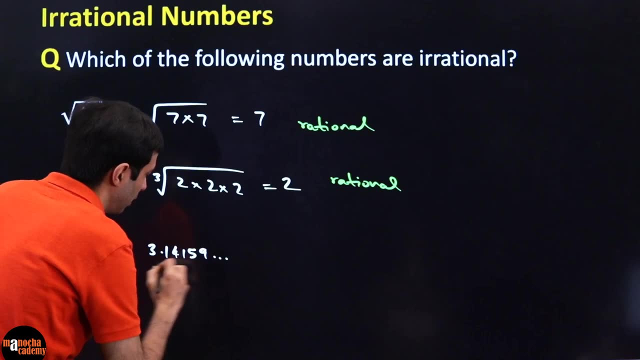 end to pi. It means a repeating pattern. It can be non-terminating, but there is no repeating pattern also. So, please, pi is not 22 by 7.. So it is basically that massive number. if you divide 3.14159, whatever, and it goes on and on, If you divide by 2, you are basically going to end up. 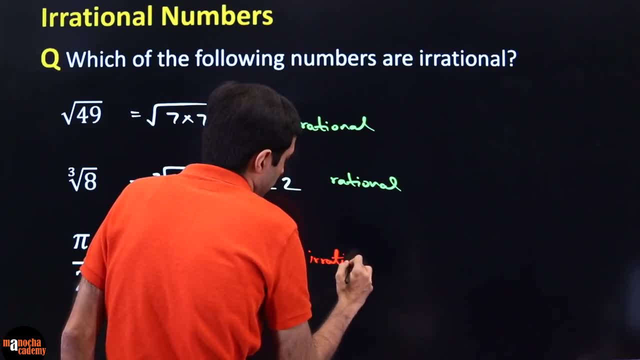 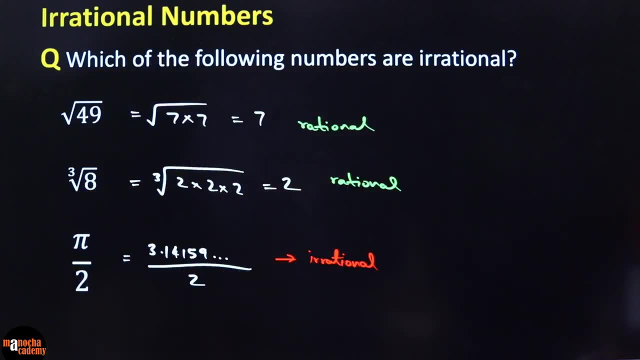 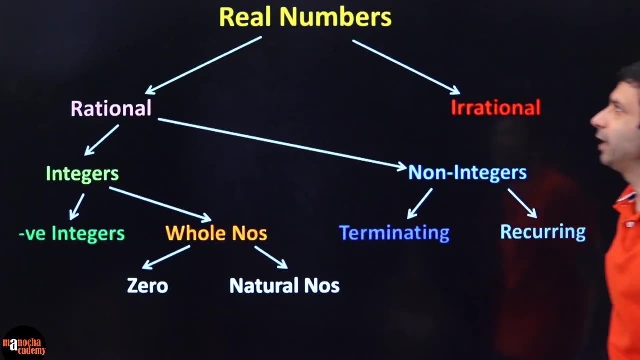 with an irrational number, Because dividing an irrational number by 2 is only going to give you an irrational number: 22 by 7, yes, that is the confusion: 22 by 7 is the approximate value of pi, not the real value Approximate. So, in summary, again I am saying this chart is very important. 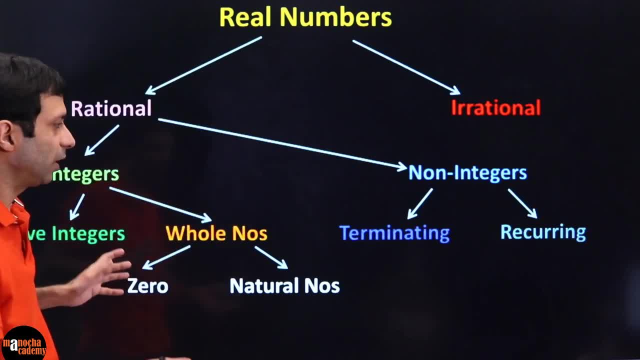 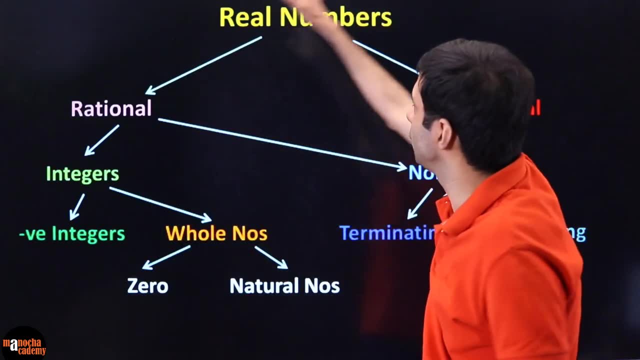 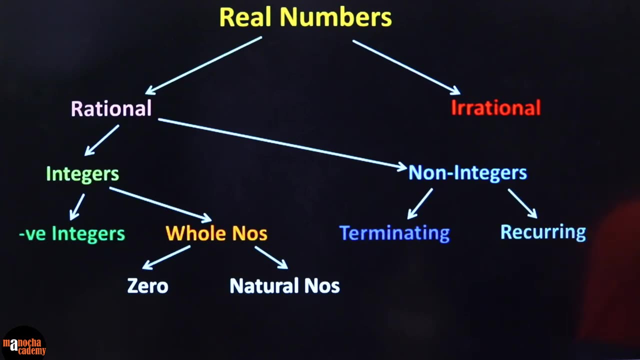 Please draw it right now And fill in some examples with me. So please draw this chart quickly, right now, Because this will really get you the whole picture clear of what is all this real, rational, irrational. everything will be crystal clear to you. Pi is even or odd. Even or odd is only for integers, Pi is not. 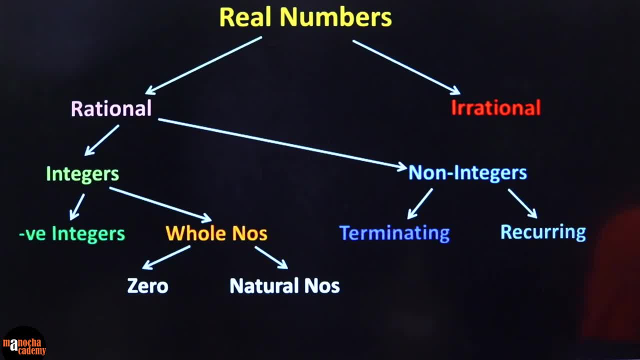 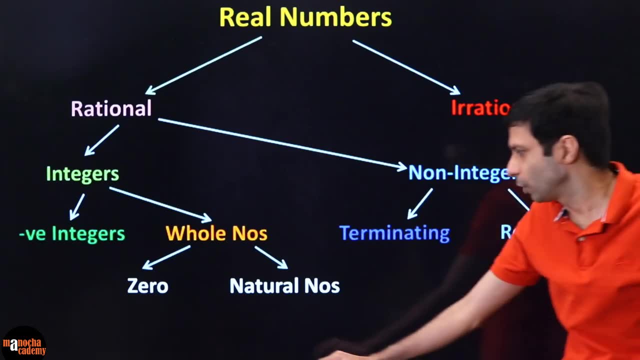 integer. it is a fraction, So we do not say even or odd. Okay, Aditya Kishore, And pi is 22 by 7 is the approximate value, not the real value. So let us look at this chart and it is always easy. 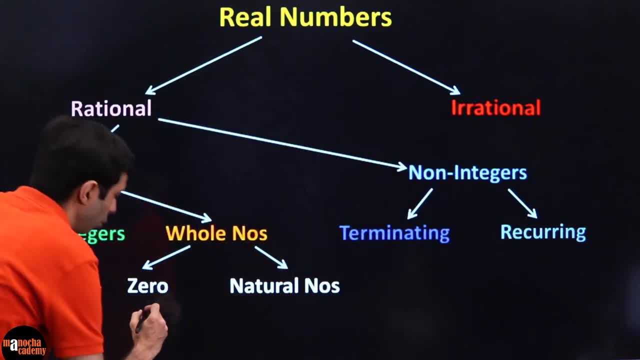 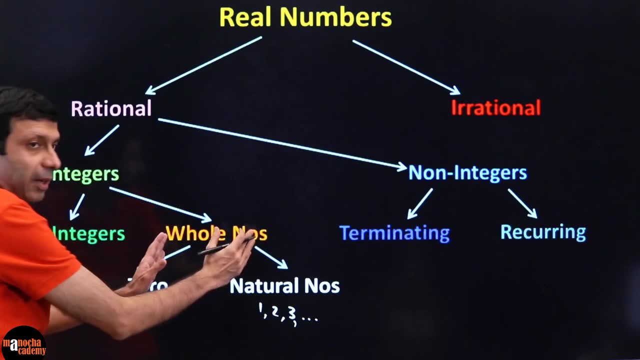 to start the chart. So let us look at this chart. and it is always easy to start the chart From the bottom. let us look with the examples. So whole numbers, natural numbers. we will start off with first: 1,, 2,, 3, the counting numbers. If you add 0 to that, it together becomes whole. 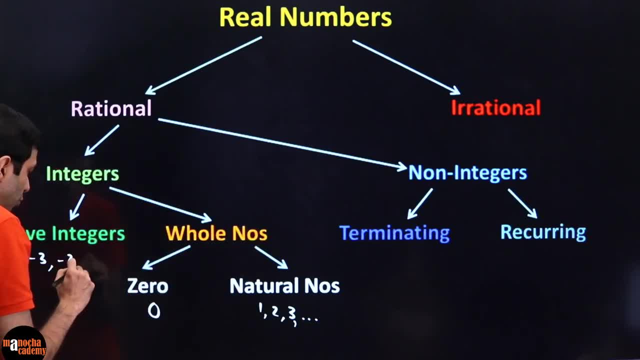 numbers. If you add negative integers to that- minus 3,, minus 2, minus 1, together these are all known as integers. So integer does not mean only negative integer, It includes 0 and natural numbers. Now if you take integers, integers are rational. They can be expressed as p by q. 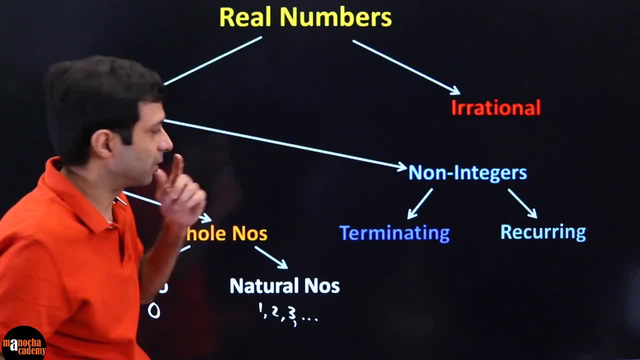 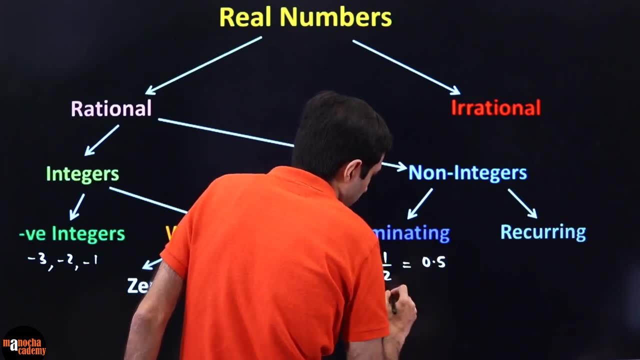 like we discussed, You can divide by 1.. But then you have also non-integers, Like there are fractions which terminate like half 0.5, like 1 by 4, or 1 by 10, 0.1.. 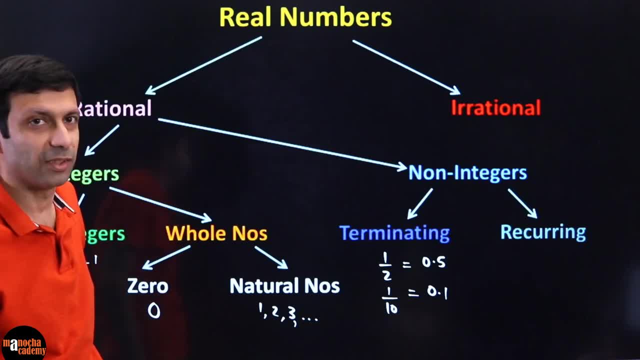 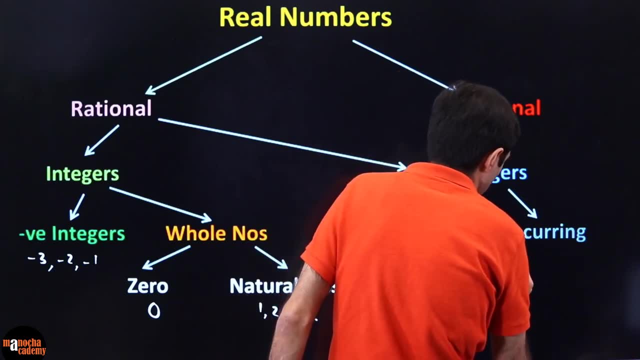 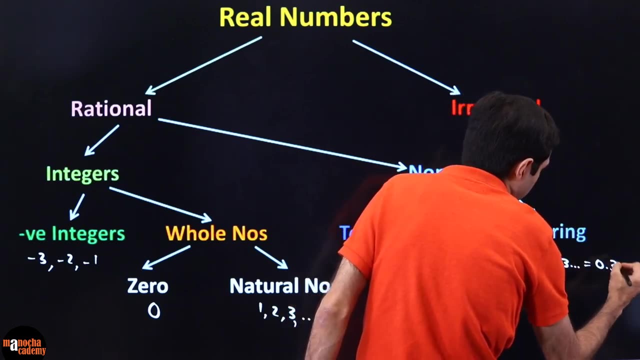 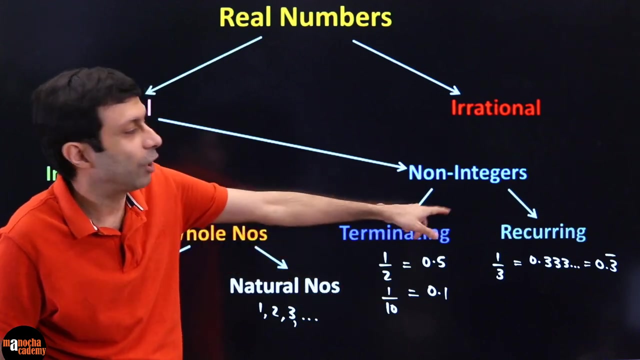 These are terminating decimals or non-integers. And then there is the recurring, which never ends, Like, for example, if you take 1 by 3,, 0.3333, or we say 0.3. recurring- and remember, non-integers means they can be terminating decimal numbers or non-terminating. 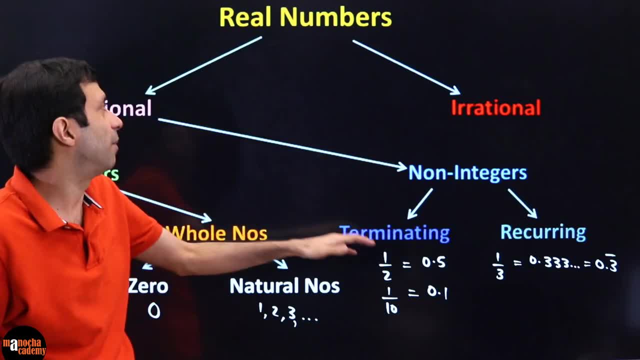 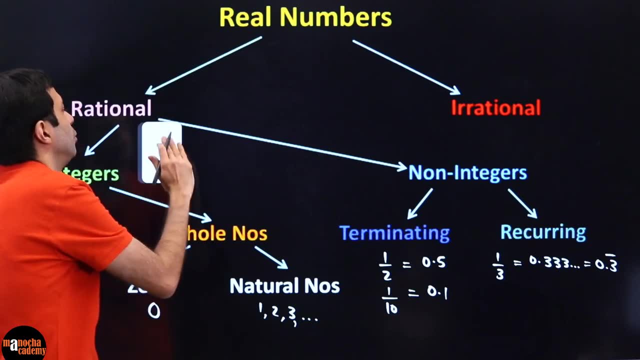 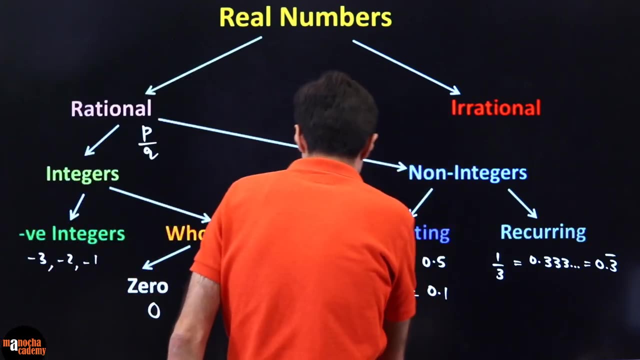 but repeating, Recurring means repeating. These all come under rational. They can all be expressed as a p by q form. But those numbers which cannot be expressed as a p by q, they are called irrational numbers, For example. so these are not p by q. 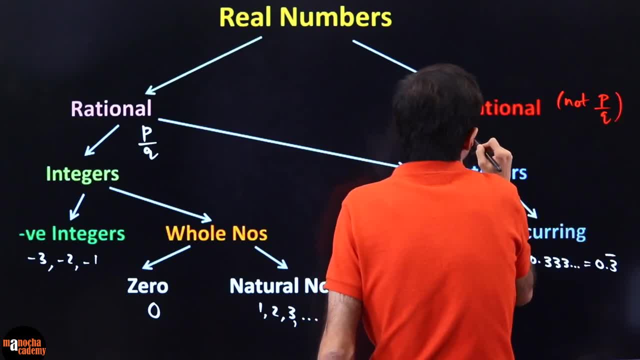 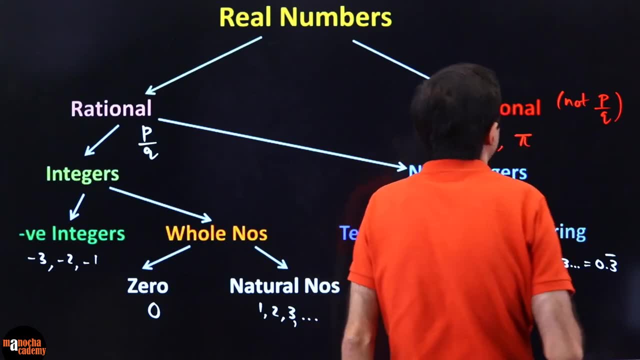 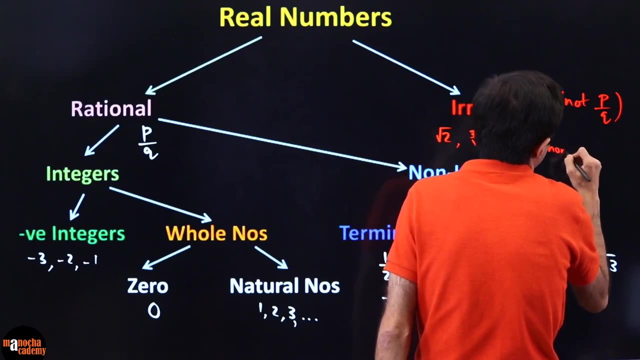 Not in a fraction, For example, square root of 2, cube root of pi or the value of pi. These are all irrational and they are all non-terminating. The decimal never finishes- Non-terminating and non-recurring. There is no repeating pattern that the mathematicians 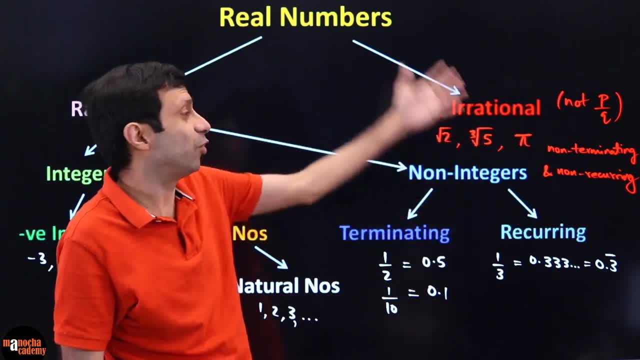 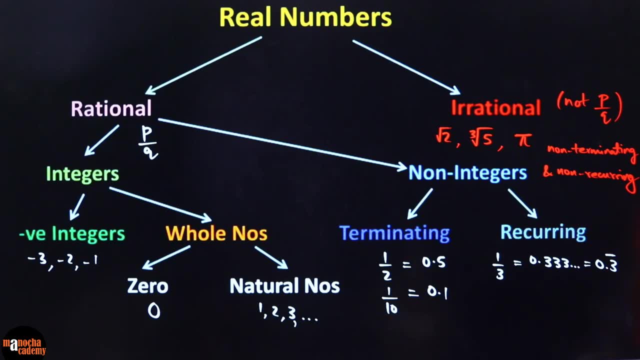 have found here. So that is why it comes under irrational. Is this full chart clear to you? Very important: Can irrational numbers be represented on the number line? Wow, Neha Shreev, excellent question, and my next slide is on that itself Because remember, 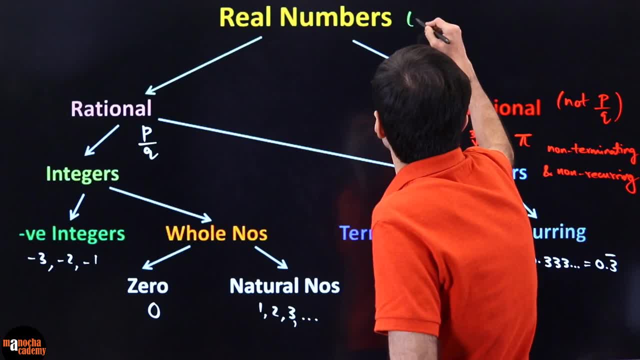 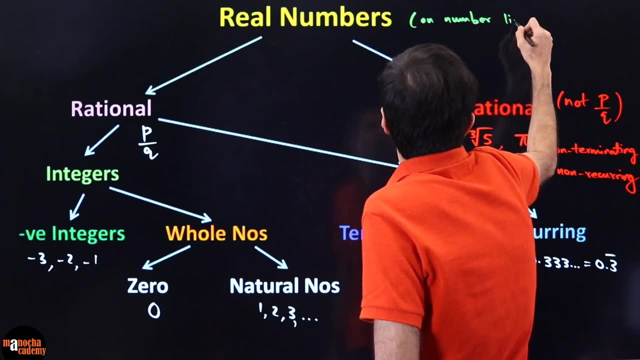 we said, all the real numbers can be represented on the number line. You can represent them on the number line. All of you know what is a number line. Rational numbers are easy fractions and all decimals you guys can easily put, just divide. 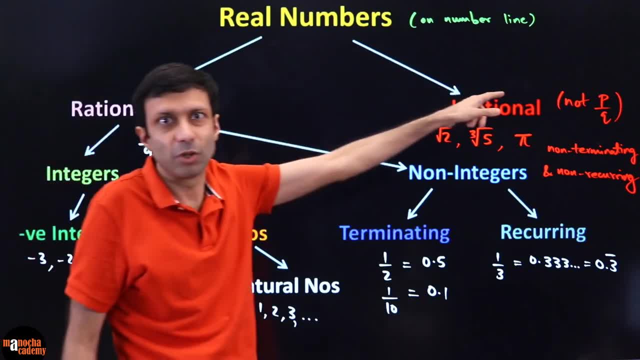 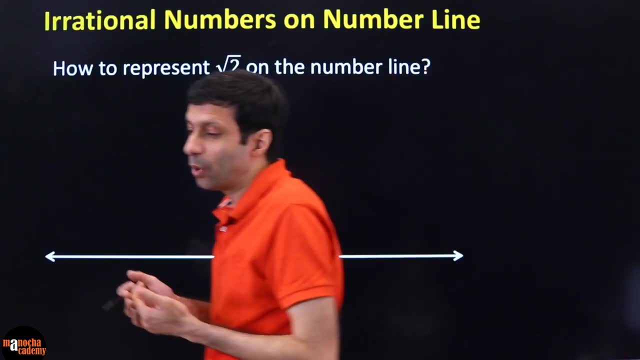 it into parts and put it in, But nu no, You see we have got it and we need to수�ilure, but how do you represent irrational numbers on number line like root 2, right? how will you guys represent this? let's take a look. so the next question is: how do i represent root 2 on the 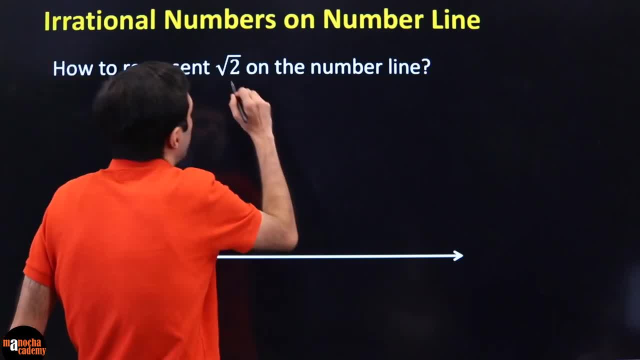 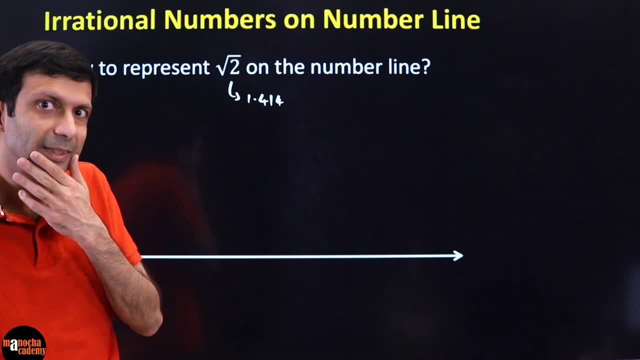 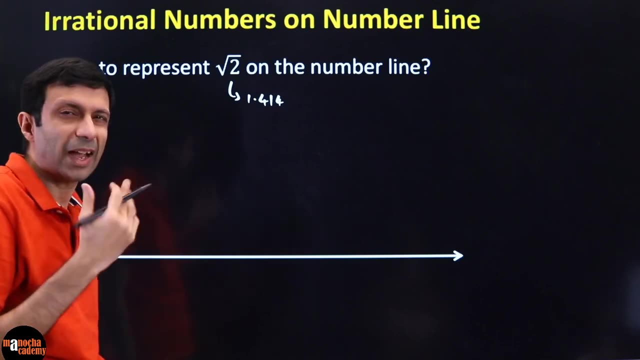 number line. now one option is you can say that: hey, root 2, i know the approximate value is 1.414, so i can you know? roughly put it, will that be accurate? will that be correct? the answer is no. that is not the accurate way to put it here. so how do you represent root 2 very accurately? 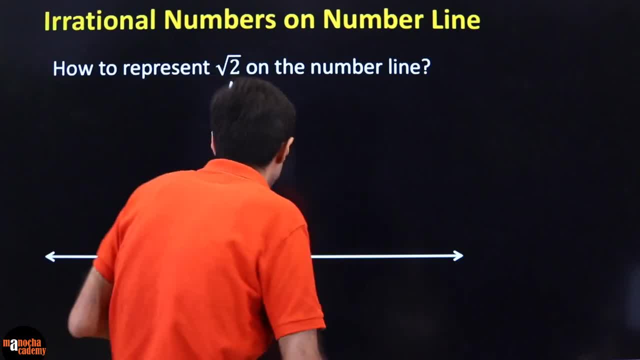 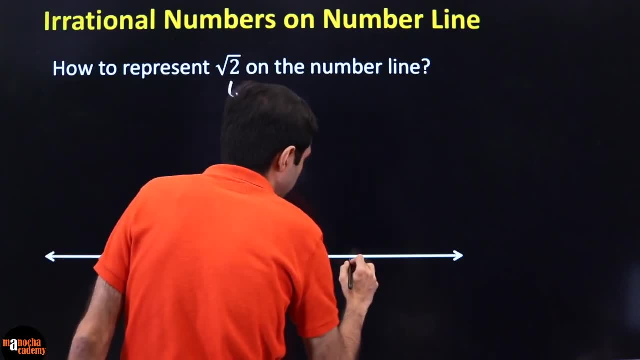 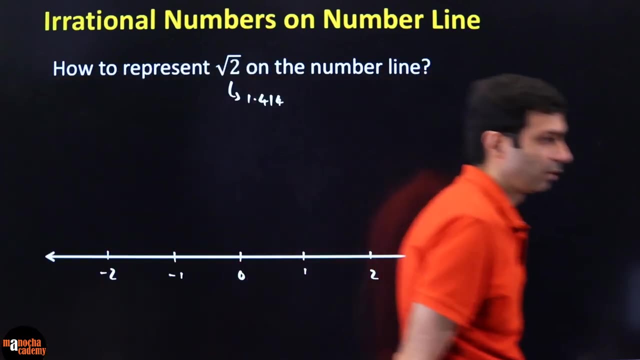 hint is using geometry, so how would you do that? so let's say: this is the number line, so you have 0 here, so this is 0, this is 1, this is 2, 3 minus 1 minus 2, and so on. any idea, guys, how to represent. 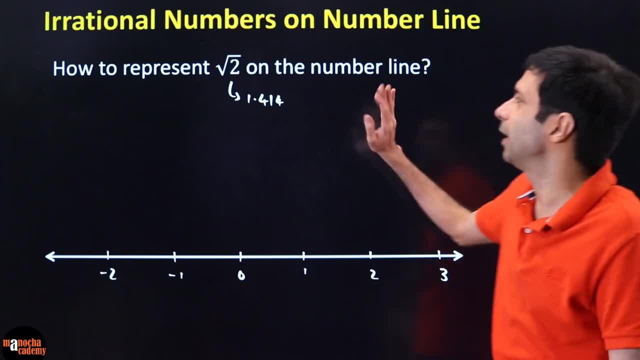 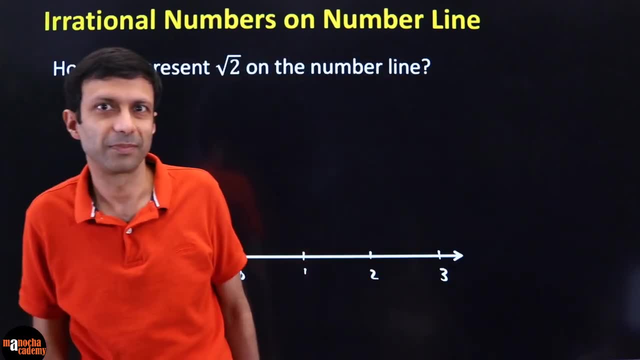 root 2 on the number line. so this will be an approximation. i can't do 1.414. so trick is: do you guys know pythagoras theorem? mr pythagoras, have you heard of pythagoras theorem? yes, yes, so why am i talking? 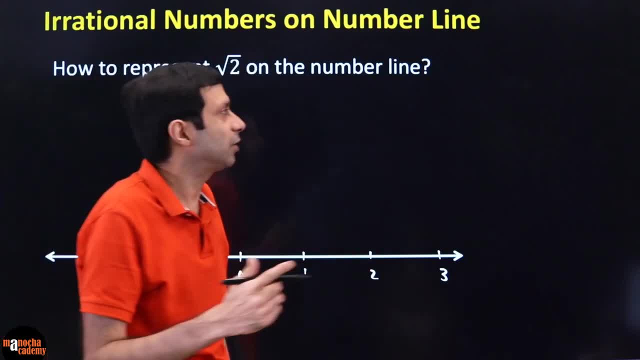 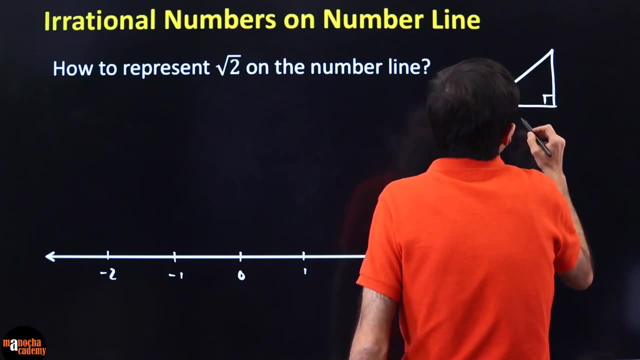 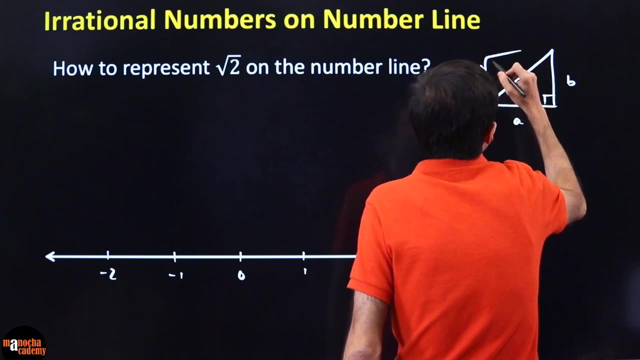 about pythagoras theorem, because, look, we are looking for root 2 and pythagoras theorem. if you guys remember, it is basically a right angle triangle where you have, you know, let's say, this is your, these two sides are a and b, and what is the hypotenuse? it is square root of a square plus. 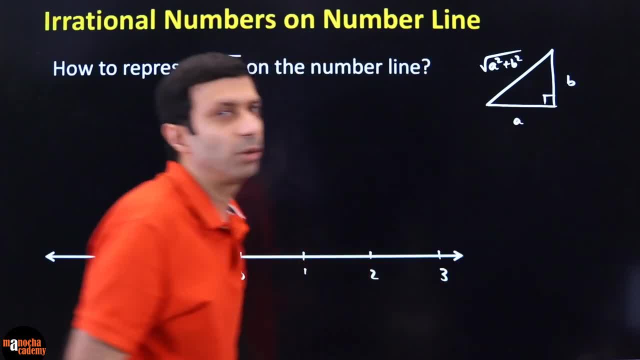 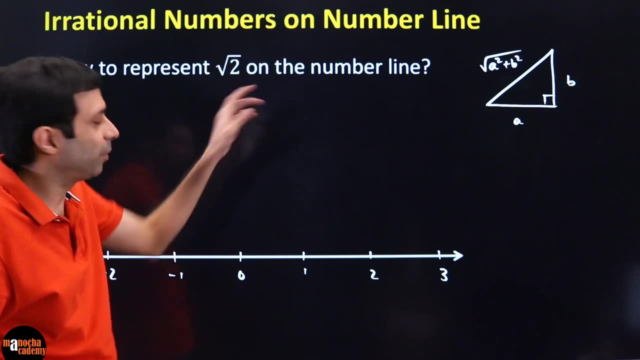 b, square sum of square of the two sides, and you take the root of that. and that is why we are going to use pythagoras, because we want a root number. so if we can use a triangle and form that somehow, we can try to put it here using maybe a compass. 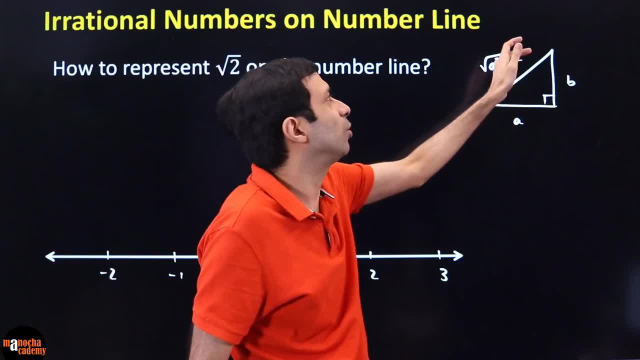 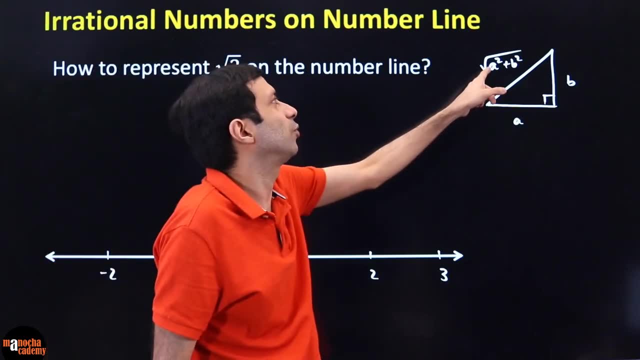 so what should a and b be? so that i get a root 2 over here. what should be the values of a and b? i want a square root of 2, and square root of 2 needs to be a square plus b square. so if you, 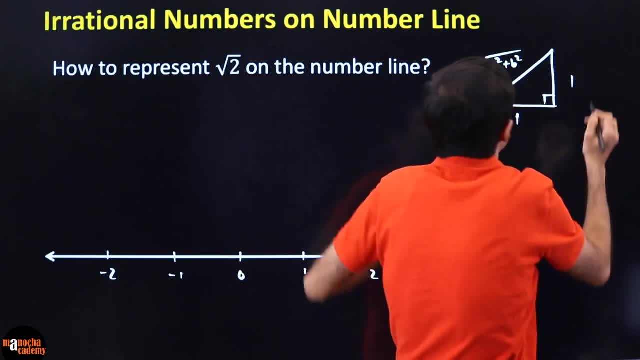 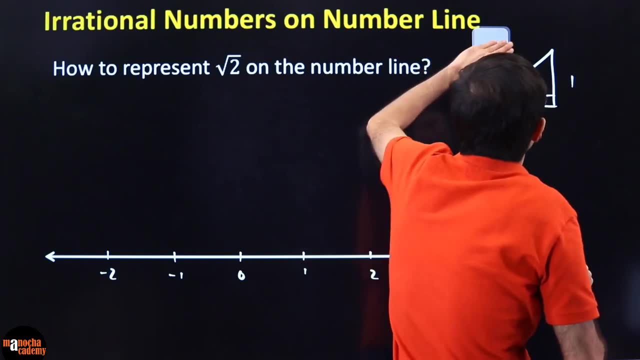 guys think carefully. if a is 1 and b is 1, square root of 1 square plus 1 square is exactly what i want: square root of 1 plus 1. so we know the length of the hypotenuse is going to be root 2. 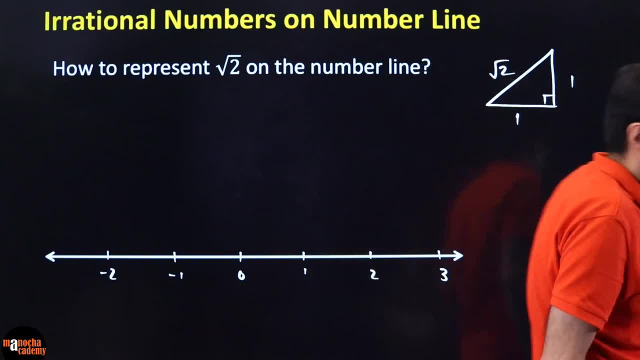 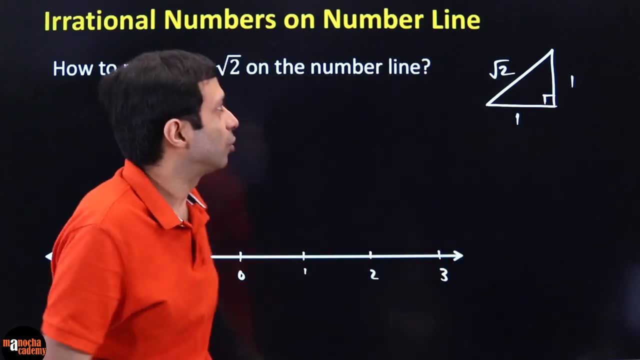 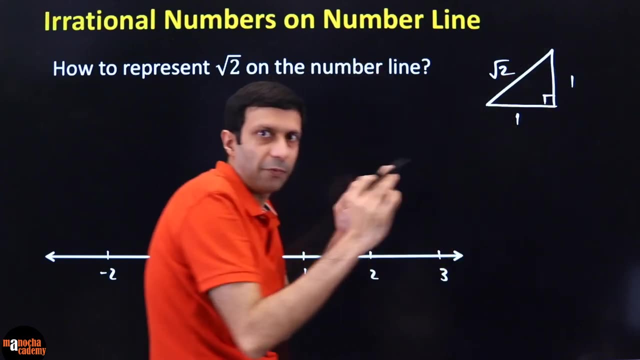 you guys agree. please look at this triangle: very good, yuvraj draw and nehashree 1: 1 right, excellent. so that's exactly what we are going to do here. so if see this one and one, if i can draw this pythagoras, uh, using pythagoras theorem, then this root 2 line is perfect in length, geometry it. 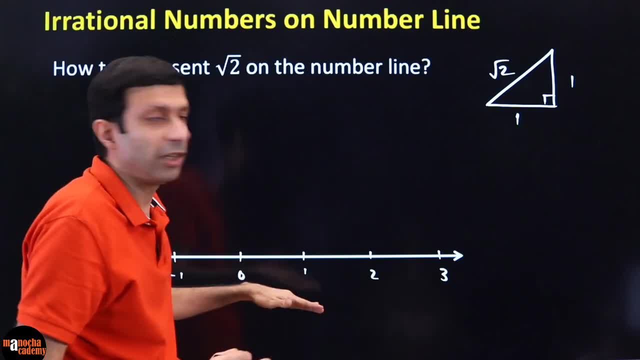 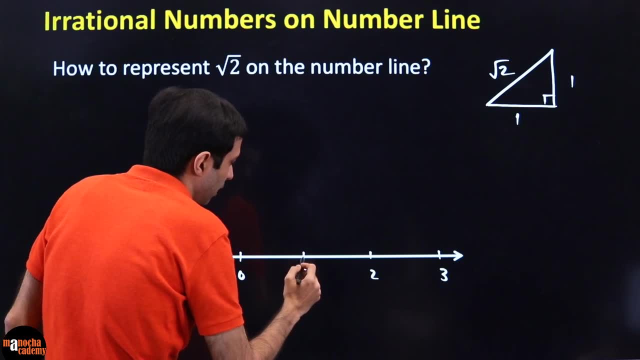 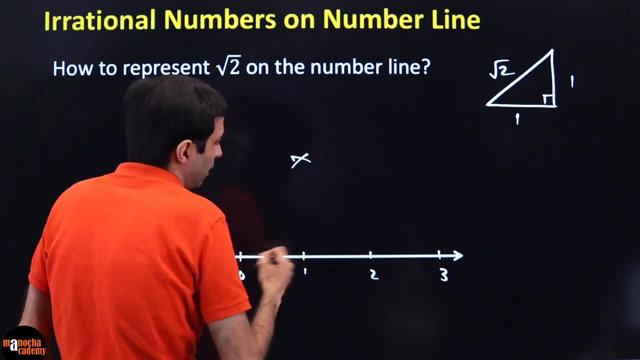 is accurately representing the length root 2 and that i just need to throw it on the number line. very simple: you draw a triangle- here- this is the length one- and you want to draw perpendicular. all of you guys know how to draw a 90 degree angle using this compass, right, so you'll put all these. 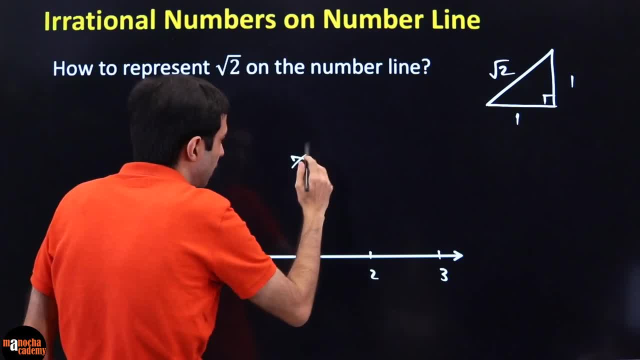 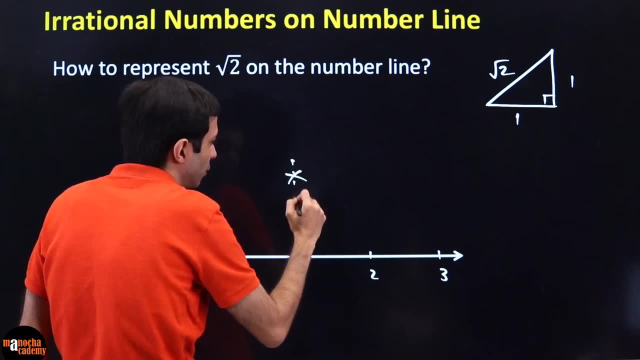 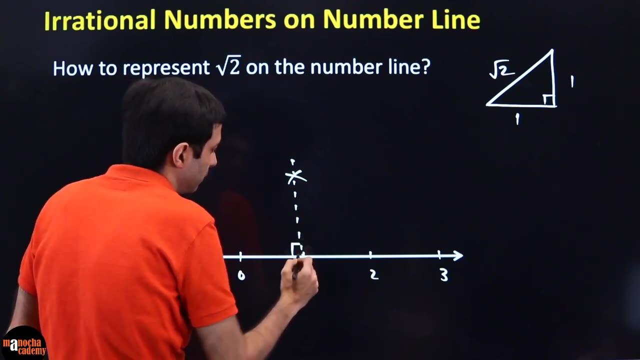 uh, you'll put all these arcs using your compass and draw a 90 degree angle, right? so all of you know how to draw 60, 120, bisect, that and all of those business, or you can draw perpendicular. uh, yeah, so you'll need to do that here, right? so you basically draw a 90 degree here. 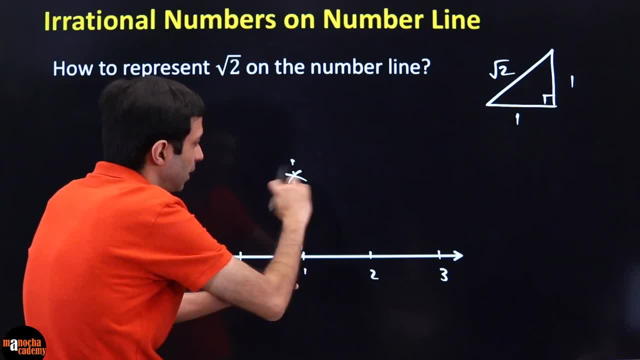 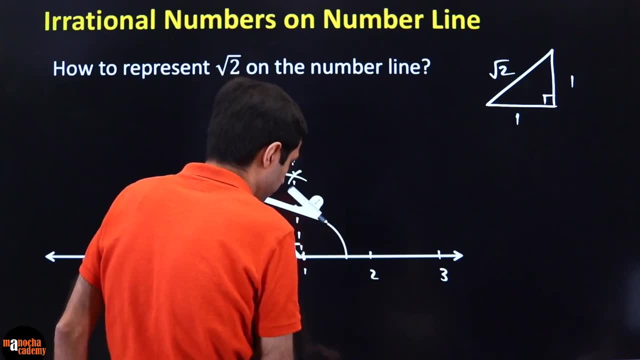 now, once you draw the 90 degree, you measure a length 1 using a compass. so take a compass and put the compass point here and mark the length of. so this measure this length of 1 and use the compass to mark it over here. right, so we will mark a length of. 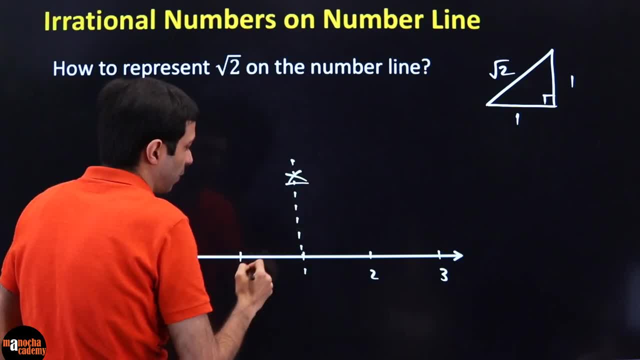 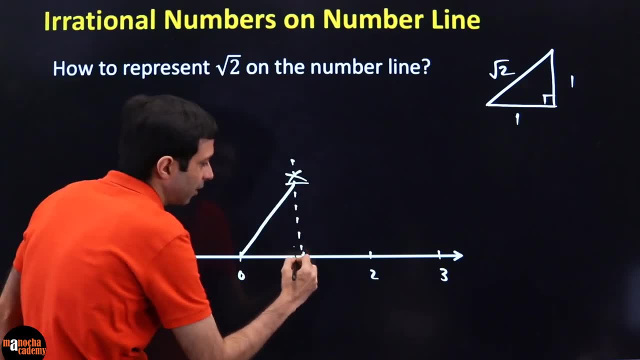 1 over here. using the compass, let's say that is 1. and then when you join this, this line, when you join, that is basically your right angle triangle and the right angle triangle and the left angle triangle. this has the root of length, of root 2. but the only problem is that, hey, i just copied the triangle and 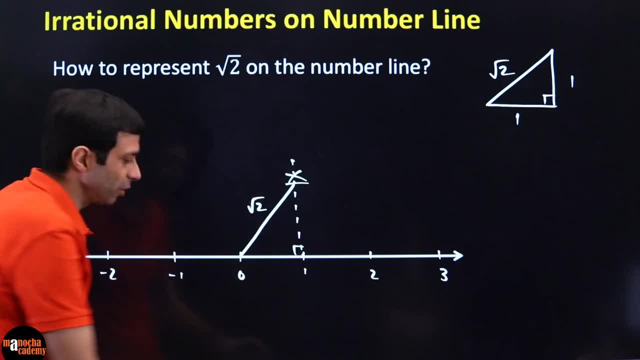 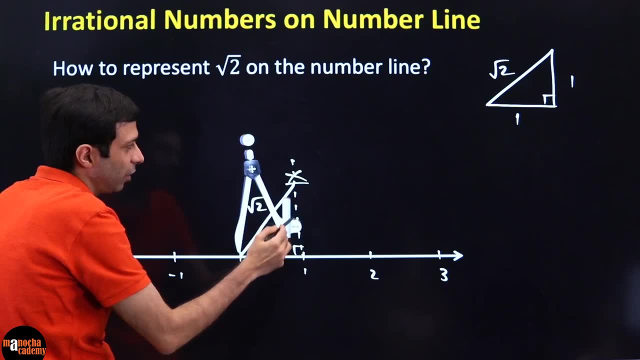 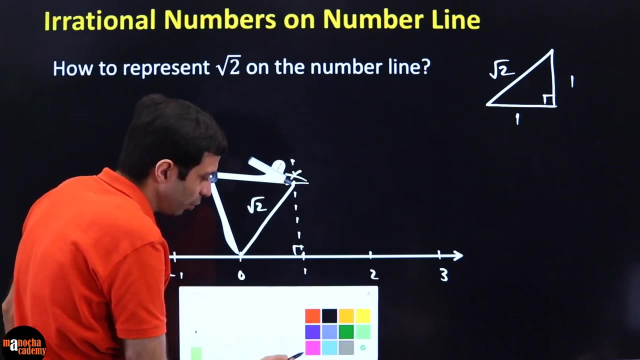 drawn it here. i want the root 2 on the number line. how do you put it on the number line? very easy, again, use your compass tool. put your compass point here accurately with the compass, put it over here, measure this length, root 2 using a compass, and then all you need to do is you need to. 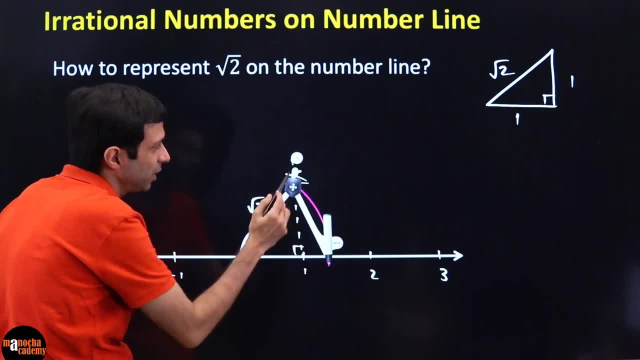 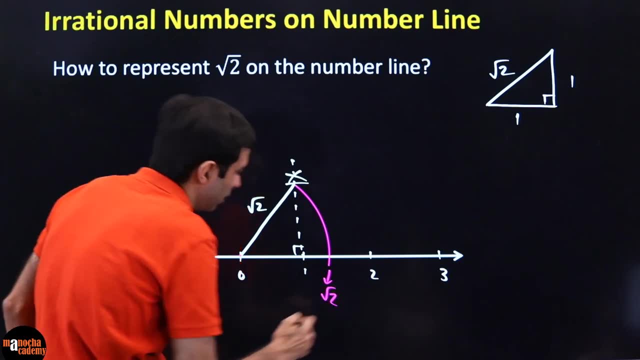 drop this arc, this compass, here and there, you see, you will get where it intersects. the number line is where you get your root 2. did all of you get that? put your compass point here and with that length of root 2, with this length, you draw the. 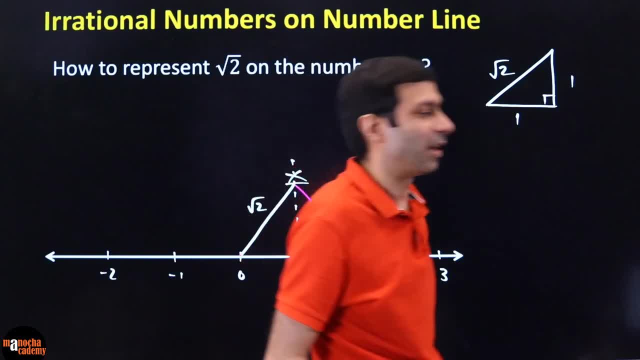 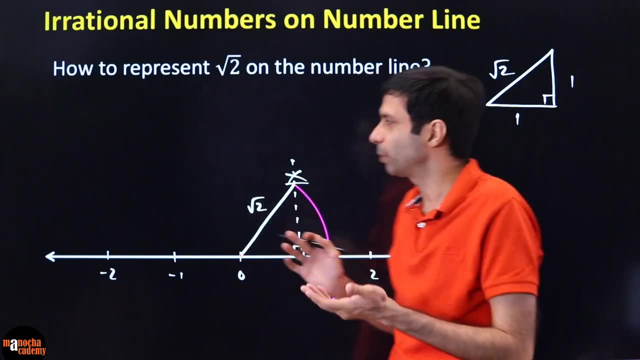 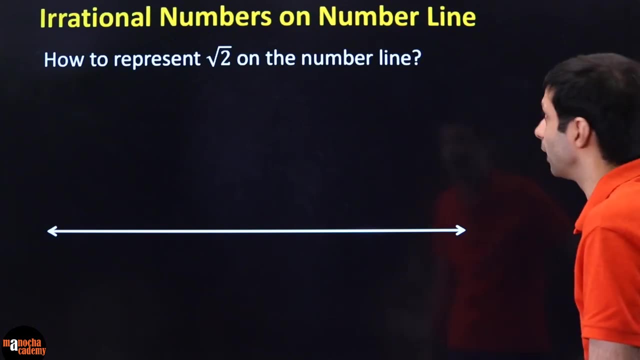 arc, you will get root 2 very accurately on the number line. this is a very basic and important technique. i have some more details on more irrational numbers. you can watch my video. but root 2 and we look at another example. so we have talked about how to represent root 2 on the 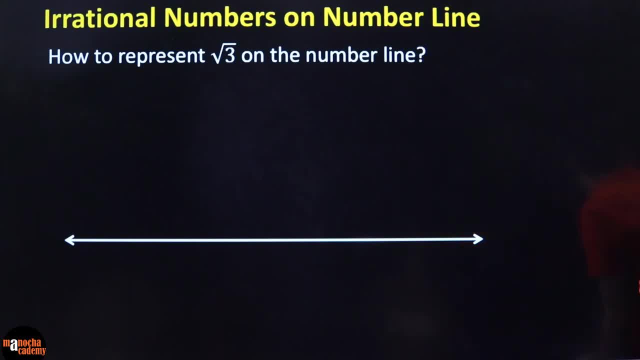 number line. we will talk about how to represent root 3. yes, there is semicircle method also. so, aditya, aditya, that's absolutely right. you guys can watch my video on the semicircle method. so there is a semicircle technique which is very useful for any general number, but that you guys. 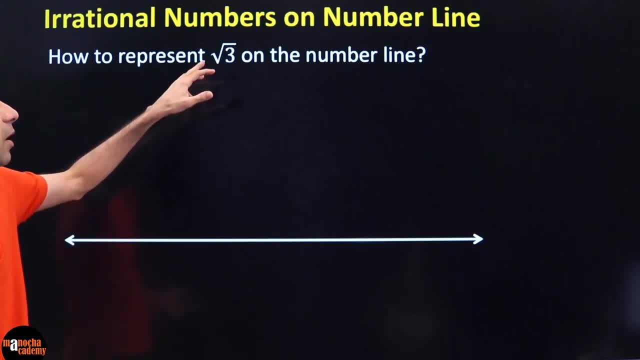 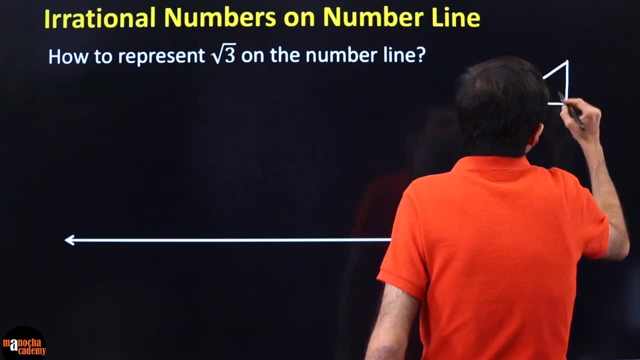 can watch my video. right now we are doing with the simple pythagoras theorem. now, how do you represent root 3? again, think of it. you need a triangle here. you need a triangle in such a form that it's hypotenuse square. you need a triangle in such a form that it's hypotenuse square. 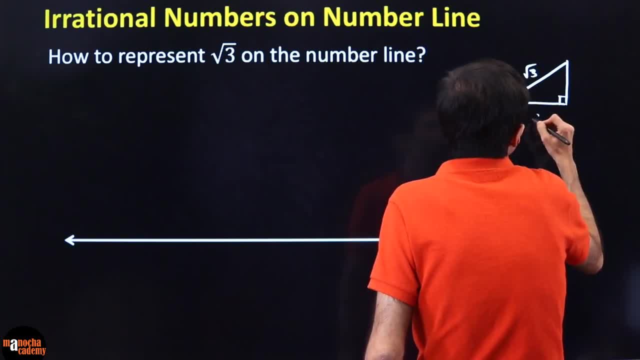 you need a triangle in such a form that it's, hypotenuse, square root of 3. so to get square root of 3, what do i need? so this is remember a and b. so this is square root of a square plus b square. now, let's say b is 1. what should my a, b so that i get a root, so that 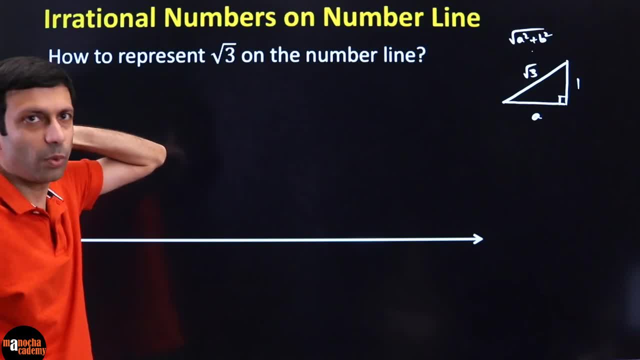 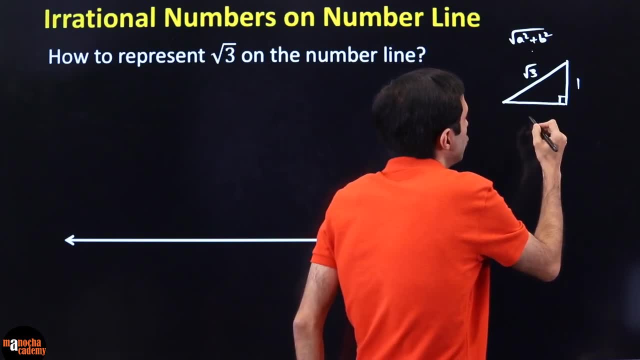 i get a 3 within that square root, that means a square should be 2. right, then 2 plus 1 will give me a 3. if a square should be 2, then a needs to be square root of 2. please check, that is this. this is. 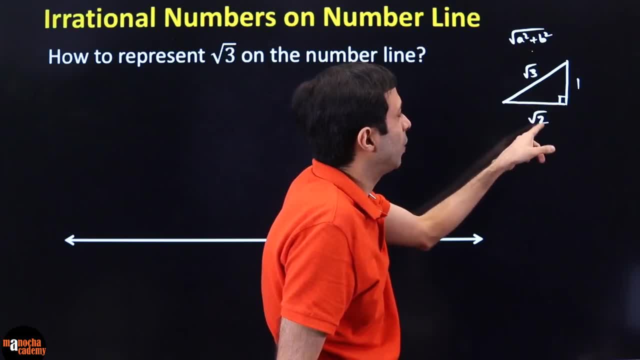 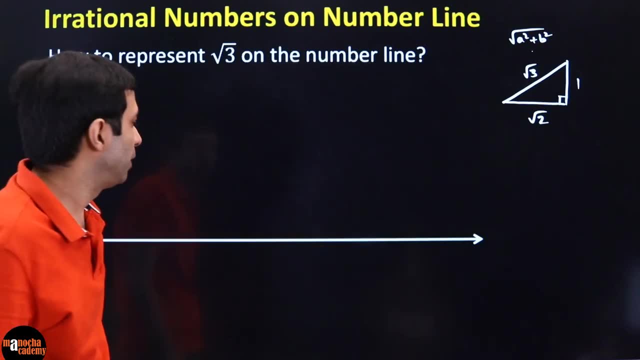 this, this pythagoras, uh, uh, numbers correct. square of root: 2 is 2, 2 plus 1 is 3, see root of 3. so i need such a triangle now. how do i get that very simple again. if this is your number line, okay, if this is. 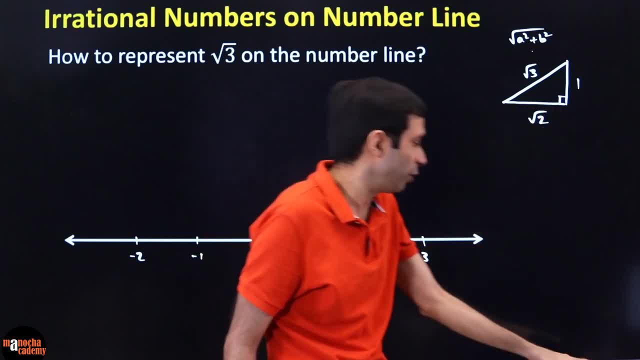 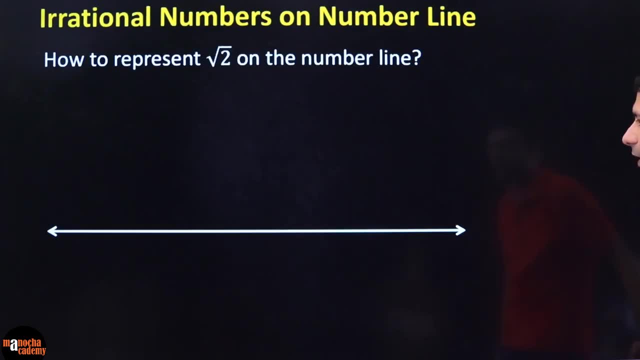 your number line. first thing is you get root 2. how do you get root 2? we just did it. you get root 2 accurately using your compass and staff, right? so first get root 2 on the number line. so you followed the previous steps. and you got a root 2 on the number line. so you followed the previous. 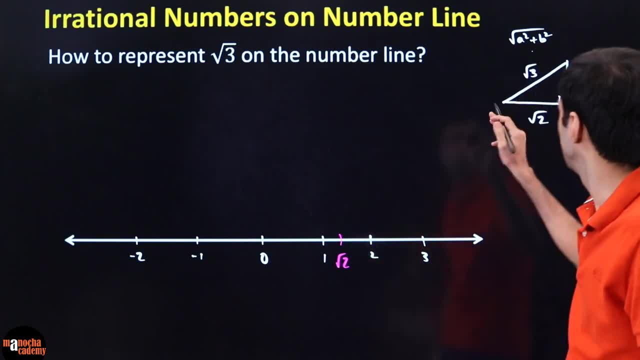 steps and you got a root 2 on the number line. so you followed the previous steps and you got a root 2 over here. root 2 over here now. since you have got root 2- you just now. since you have got root 2, you just need to draw your one. how do you draw the one you? 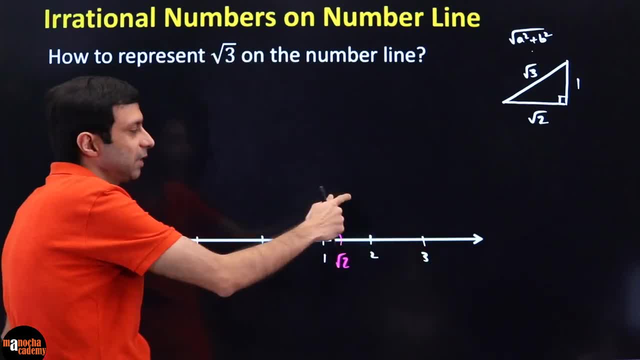 need to draw your one. how do you draw the one? you draw perpendicular. how do you draw perpendicular? draw perpendicular. how do you draw perpendicular? you know how to draw 60 degree, 120 bisect. that you know how to draw 60 degree, 120 bisect. that you guys know how to draw perpendicular at this. 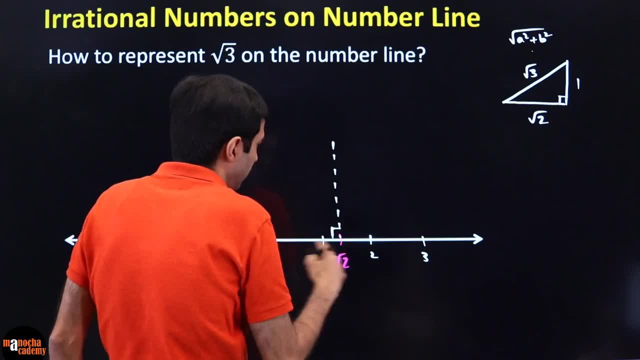 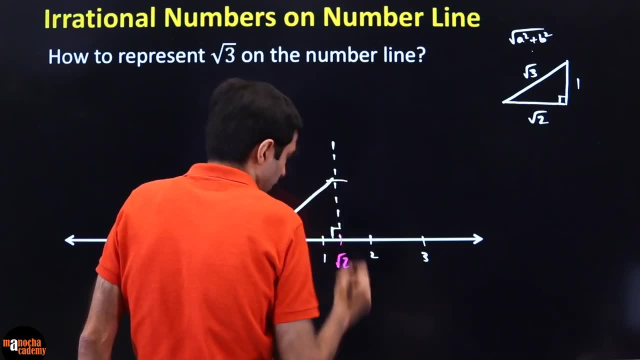 you guys know how to draw perpendicular at this point, so please draw that and then cut a length of point. so please draw that and then cut a length of one. so let's say that is your one. now you join one. so let's say that is your one. now you join from zero to this. there is your pythagoras triangle. 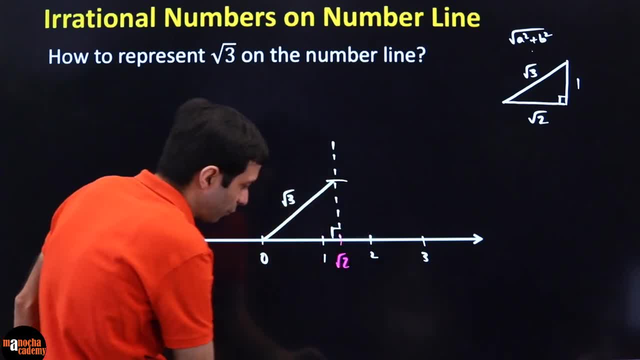 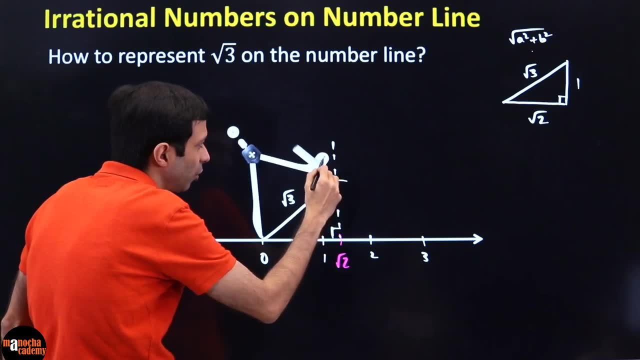 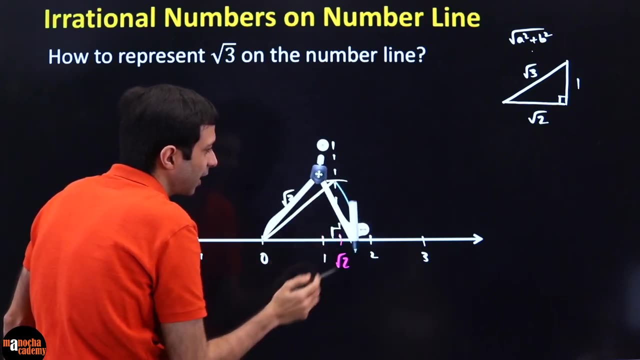 and this is having a length of root 3. now all you have to do, very simple, just keep your compass point again at zero, measure the length root 3 over here and just bring down your compass like this and accurately you will get not 1.732 but this will be the accurate representation on. 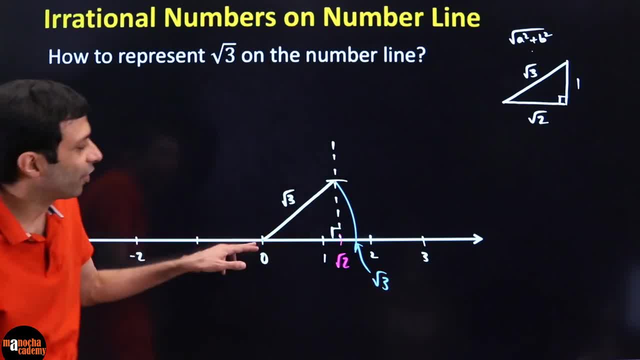 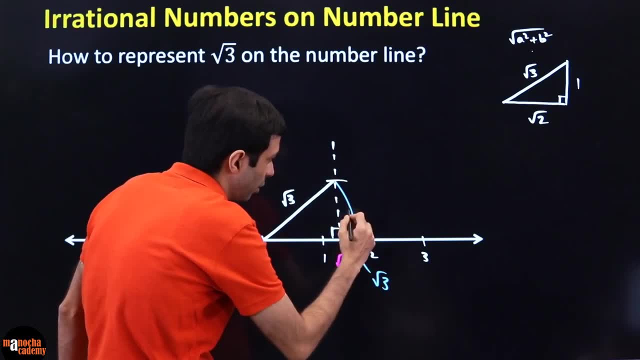 the number line of square root of 3 using a triangle of length root 2, and this is of length and this is of length 1.. how did i get this one? very simple: all you have to do is put the compass here and mark a length. 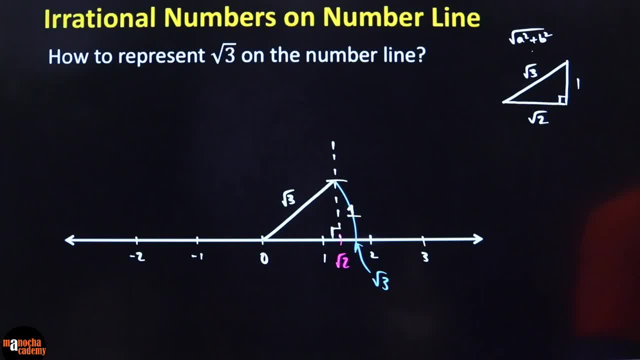 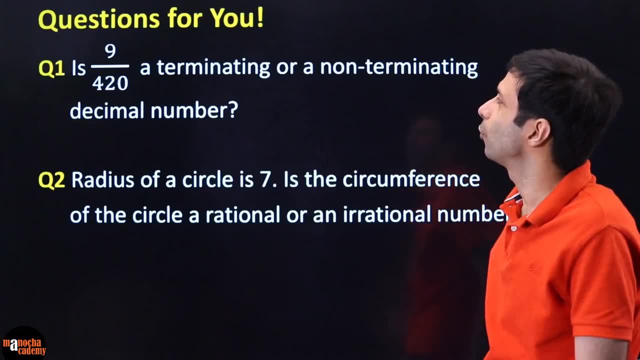 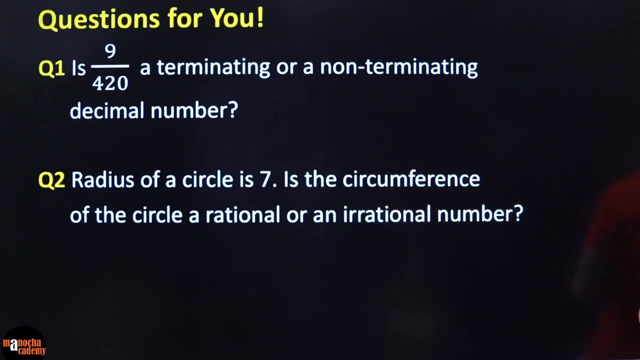 of one here. that's it. that's all you needed to do, so this one is clear to all of you. i have a couple of questions for you now. how do you decide? is 9 by 420 a terminating or non-terminating decimal number? can you guys do that for me? is it a terminating or a non-terminating decimal number? 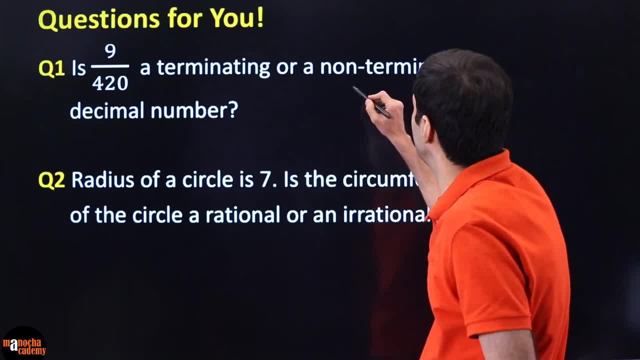 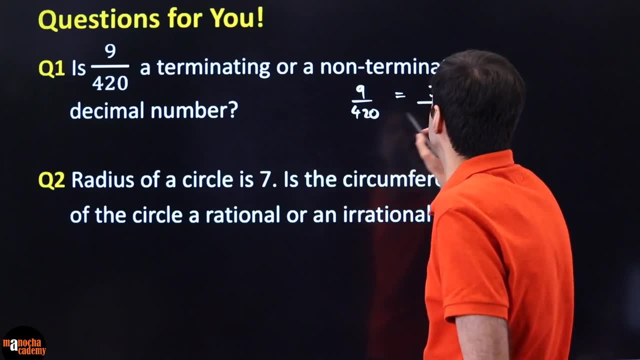 so again, let's uh to do this. first, let's write 9 by 420, 9 is nothing but 3 times 3, so you should always make sure you simplify your fraction. what is 420? 420 is 2 times 3 times 7 times 2 times 5. 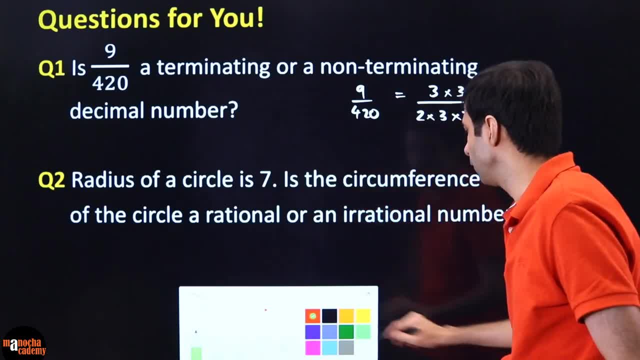 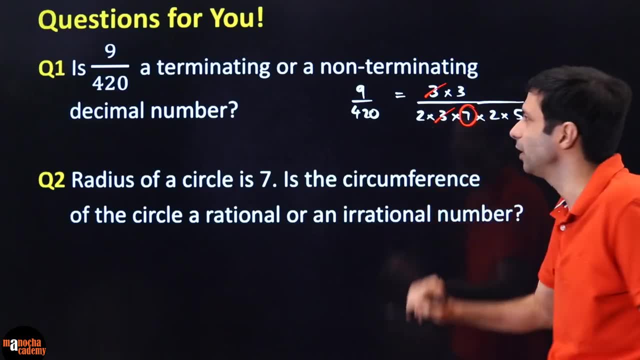 right, i'm breaking it into its factors. you can see 3 and 5 will. 3 and 3 will get cancelled here, but you can see that the denominator is having 2, 2, 5, but there is a 7 here. so you can see that the denominator is having 2, 2, 5, but there is a 7 here. so you can see that. 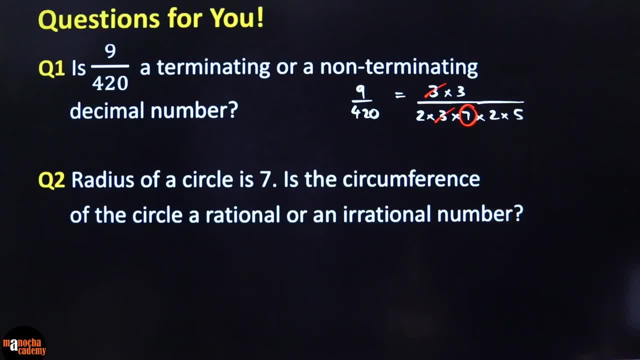 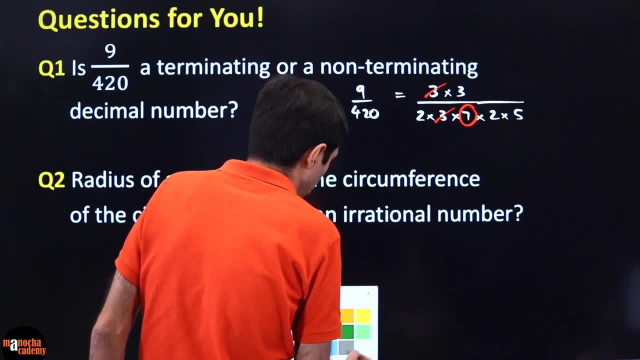 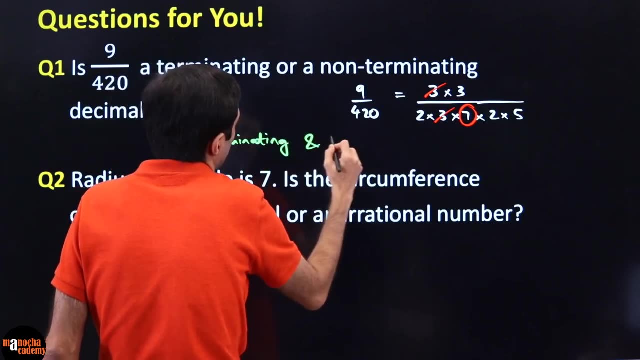 so what do you guys think? will it be terminating or non-terminating? clearly it is going to be non-terminating, but repeating, recurring, because there is a factor other than 2 and 5. so answer is: non-terminating, but also, and recurring. crystal clear. last one: radius of a circle is 7, is the 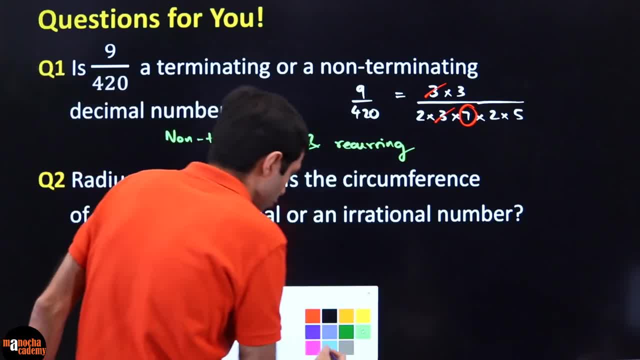 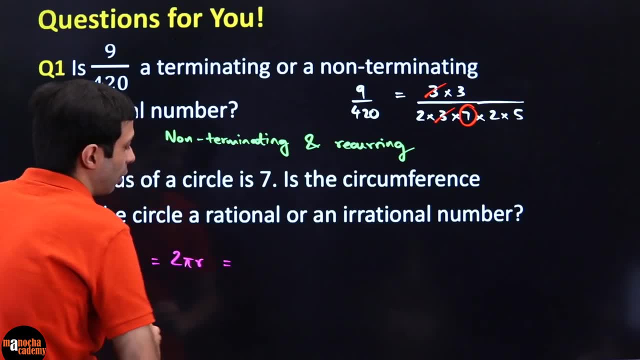 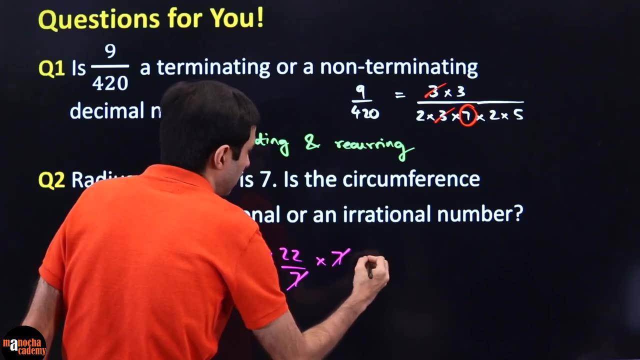 circumference of the circle, a rational or an irrational number. so what is the circumference of a circle? c circumference is 2 pi r. now, a lot of times we are tempted to do this: 2 pi is 22 by 7 times 7. so we say, hey, 7, 7. cancelled answer is 44. whatever be the units rational number, right, what do you? 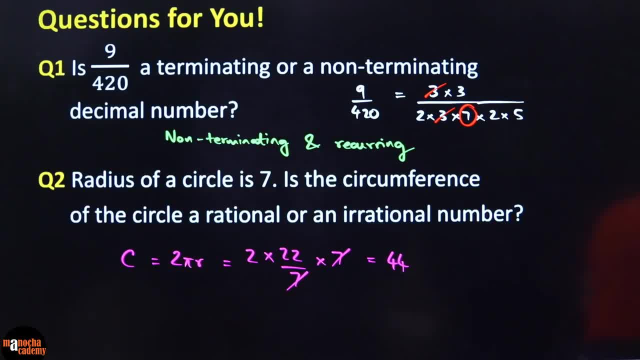 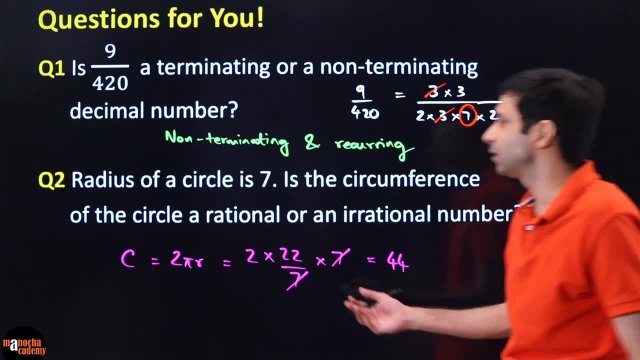 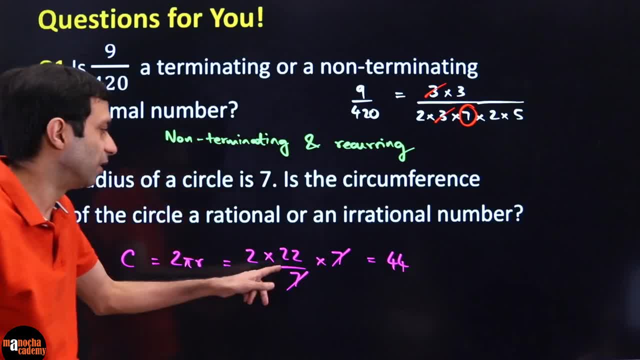 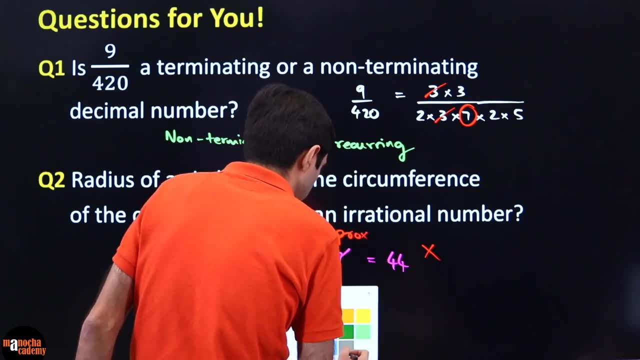 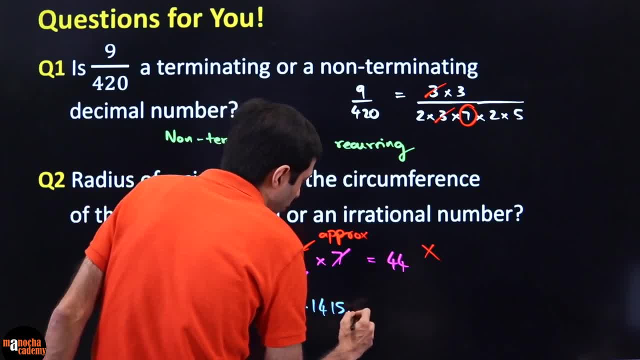 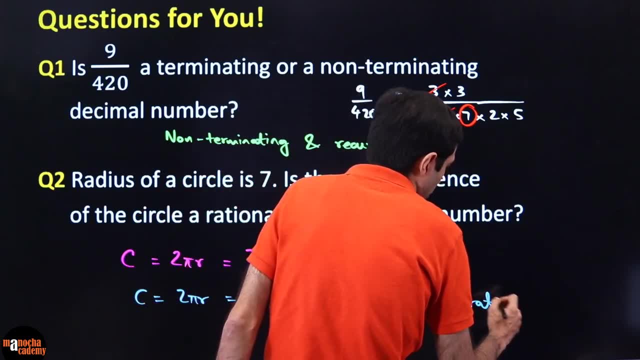 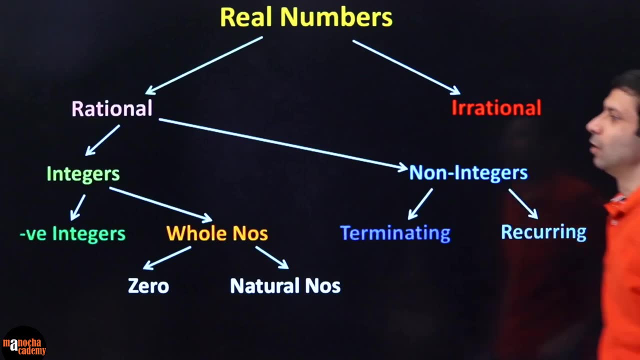 2 into 3.14159. dot dot, dot, right. whatever times 7, then it will always give you a irrational number. so you have to use the accurate value. so the correct answer is irrational. okay, so this was a trick question. so, in summary, i would again remind you. please remember this important chart. 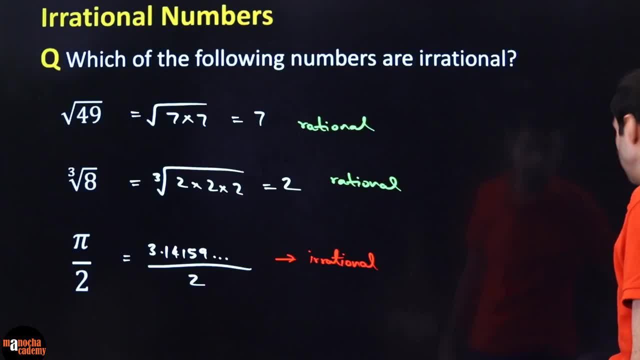 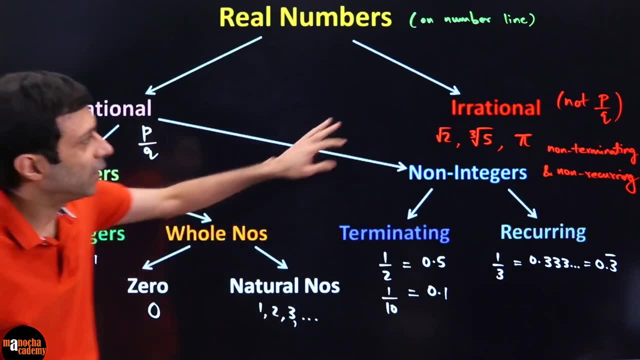 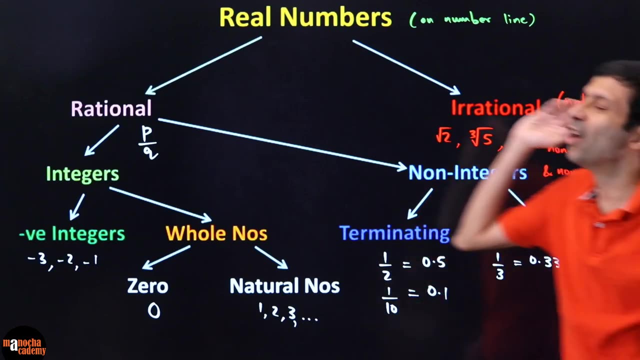 that we did and the easiest way to remember it is with these, all these examples. so you should write down this chart. i made it very simple for you, very clear, and please write understand these words: terminating, recurring, non-terminating, non-recurring. then this whole real numbers is going to be. 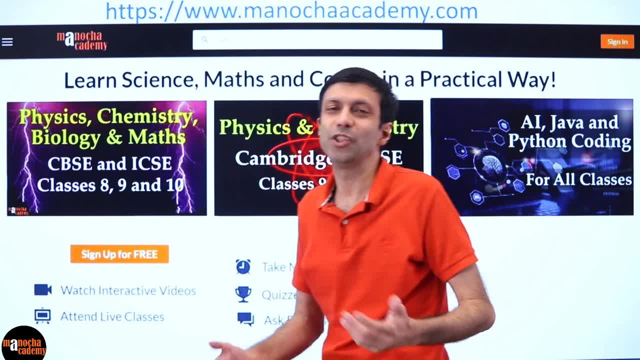 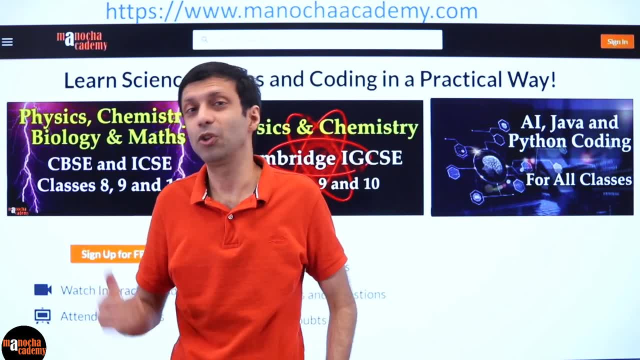 really easy for you, okay, so hope you enjoyed this maths class on real numbers, or what we call as number systems, and hope the concepts are crystal clear. and do check out the other courses on our website if you haven't taken the other courses, and also please do share it out with your friends. 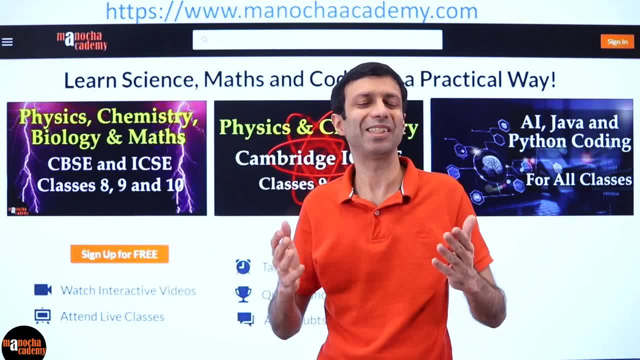 so stay connected with manucha academy and just enjoy your learning.